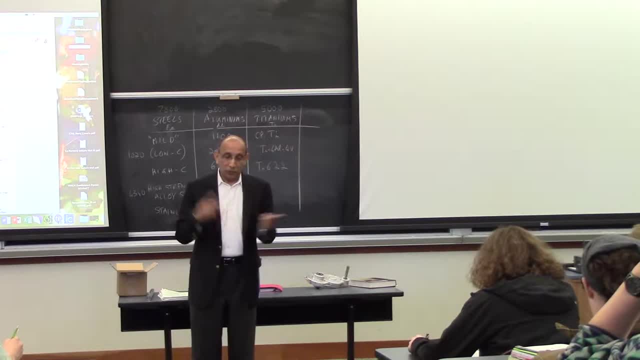 So it costs you money. The second: so aluminum is all over us, so aluminum would be cheap to extract. The second part of that is demand. So if people want a lot of it, then you make a lot of it and you buy it. 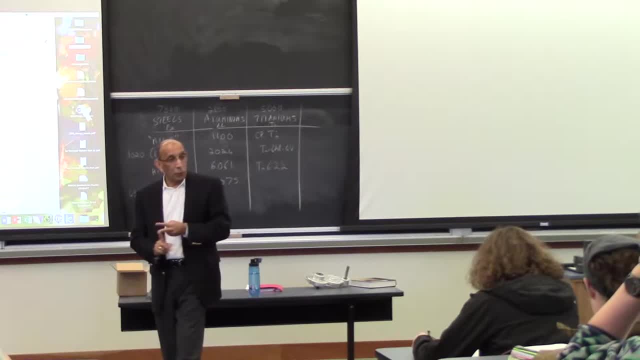 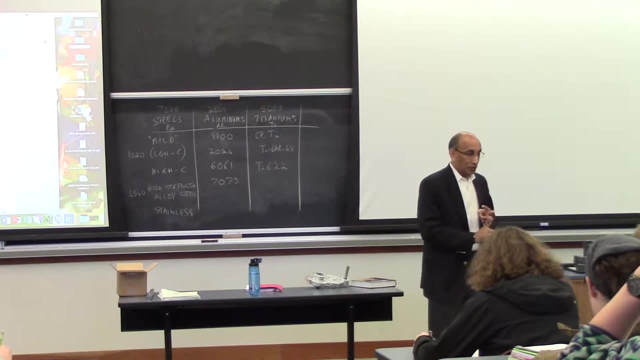 So TI-6 forward. people want a lot of it. Price is lower than on the other, your TI-622,, which people don't need that much. And the third piece is sort of processing cost, What it takes to actually make this thing and provide it to you. 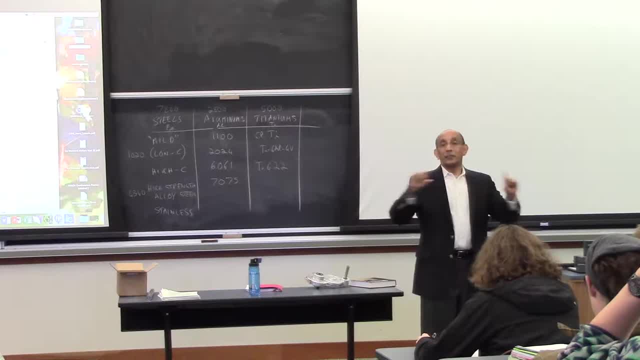 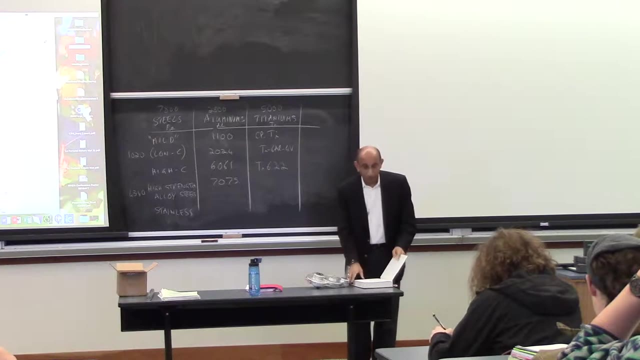 So if you want a plate of titanium versus a plate of steam, it's easier to make than a plate of steam, So the cost is lower. So those are the three pieces. Okay, Alright, so just remember these things. If you look in our textbook, you have properties for all of these in the back. 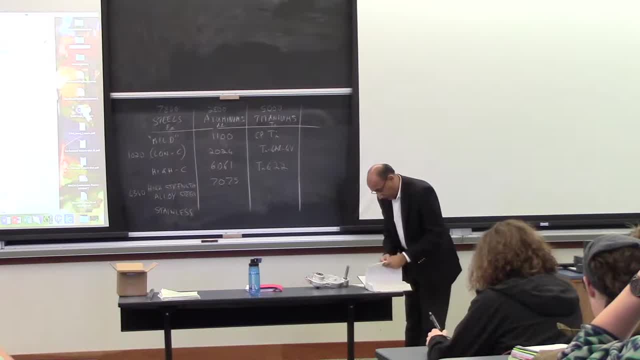 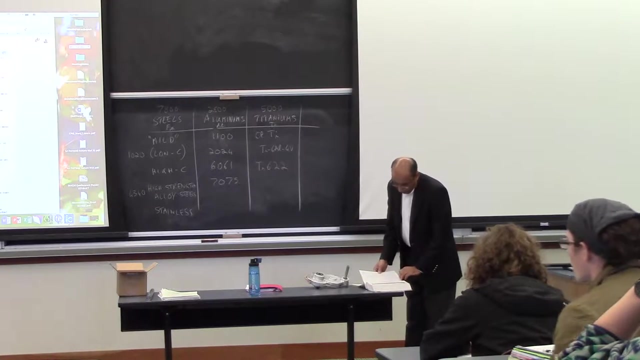 Right, so if you go look at, let's see what table we have. So if you go to the table, page 21 and on, So from page 20 through 21,. those are all steels: 22,, 23,, 24,. these are your amounts. 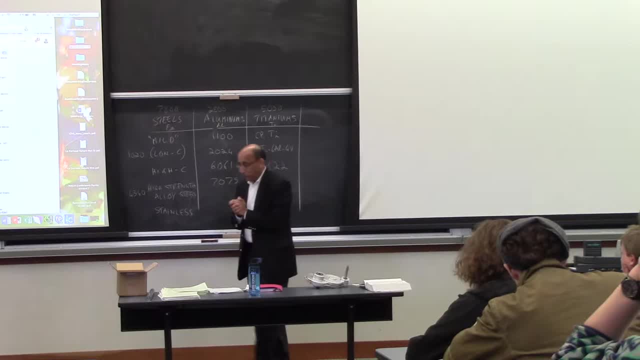 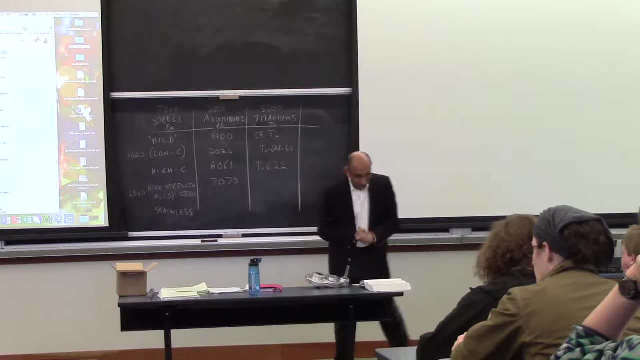 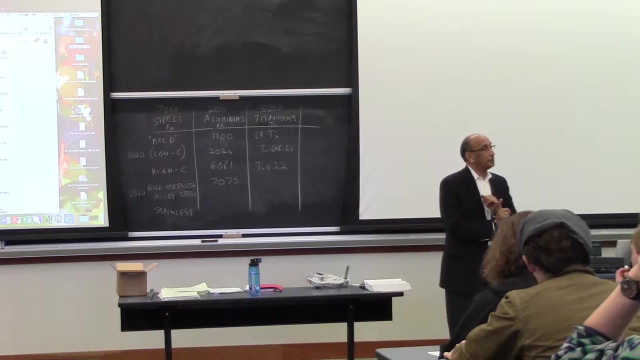 Alright. So did you guys want to say something? What problem? Is that a problem? I was aware that you were Okay. Thank you, Alright. so when you need particular properties, you go to those tables Or you go to the ASTM handbooks, which you can get online. 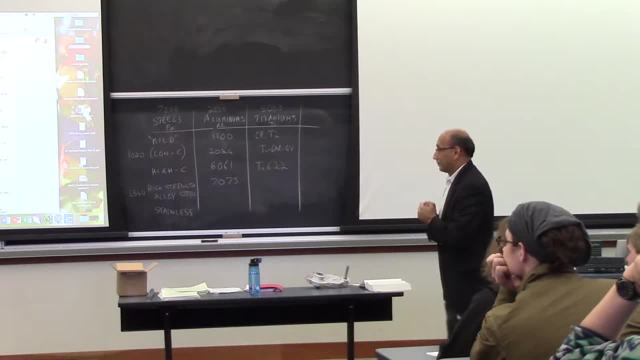 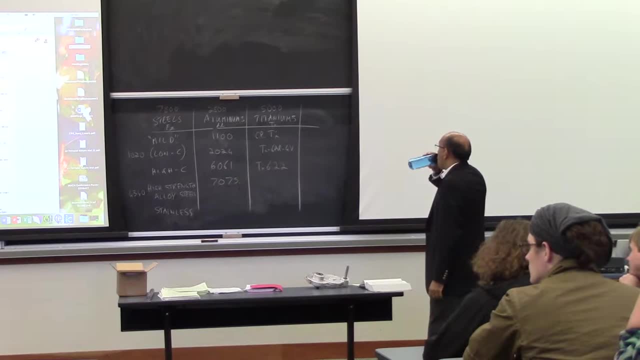 Or the ASTM handbooks which you can get online. I was just going to say about the design problems. Let's see One, please staple them. But two, check and make sure that you have a grade for the design, the last design problem that you just came in. 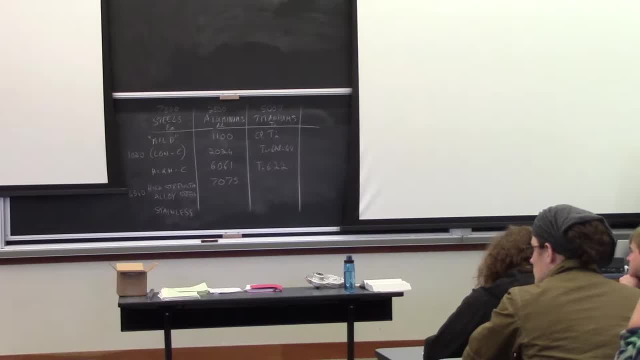 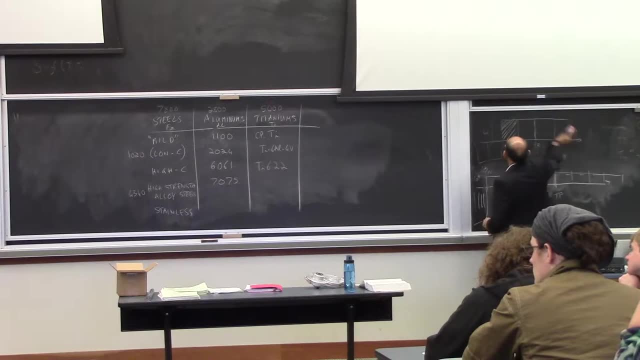 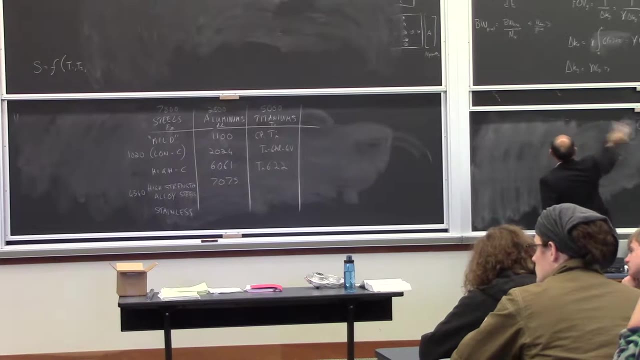 Pretty sure I got everybody, But some of the groups I just mentioned and I sent a lengthy, verbose email about things to look for for the next design problem. Please take a look at that, because it was like really nice grading these And Chris is grading the next one. 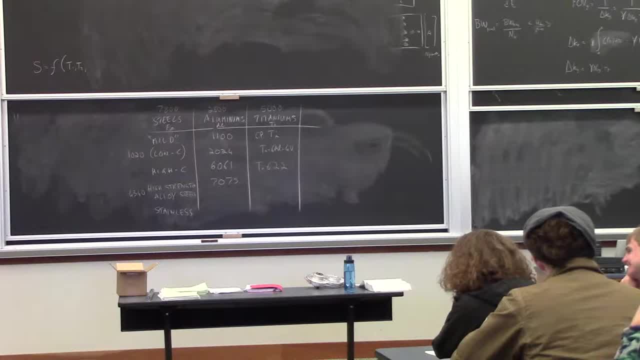 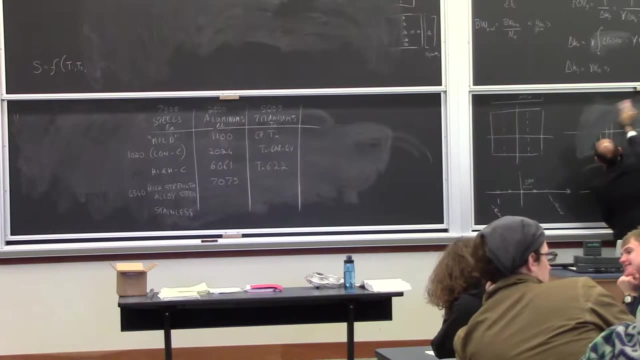 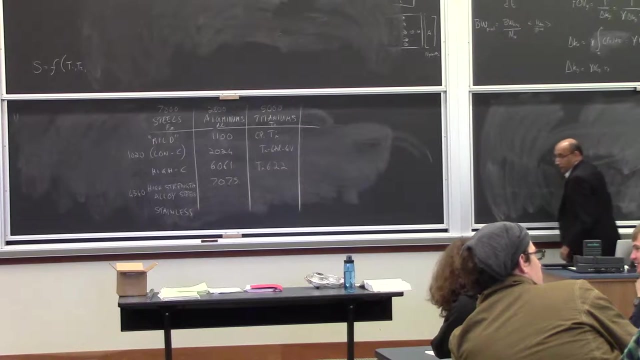 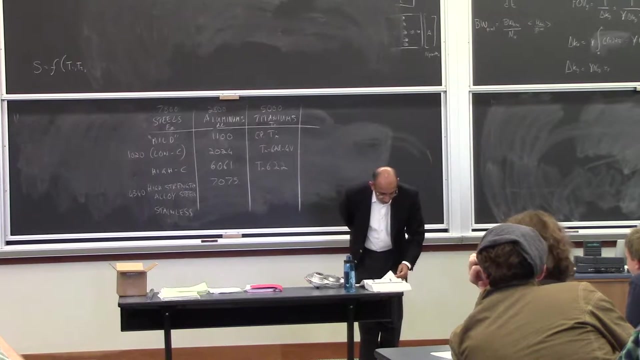 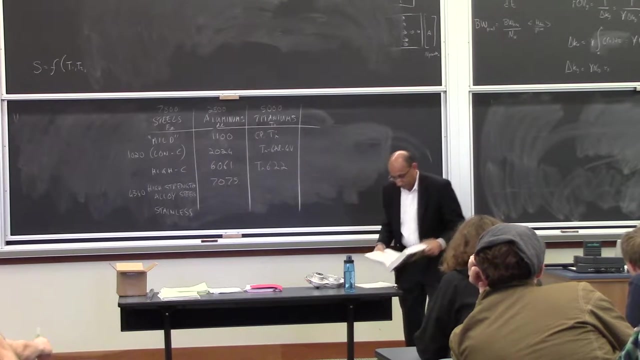 and he probably won't be as nice, Alright. that being said, that's it. Any questions for anybody? Alright, thank you. Okay, Let me just give you some numbers off the table, So let's look at So. What I mean by heat treatment is. it turns out that the strength of a metal alloy depends on the temperature that it's seen in the past. 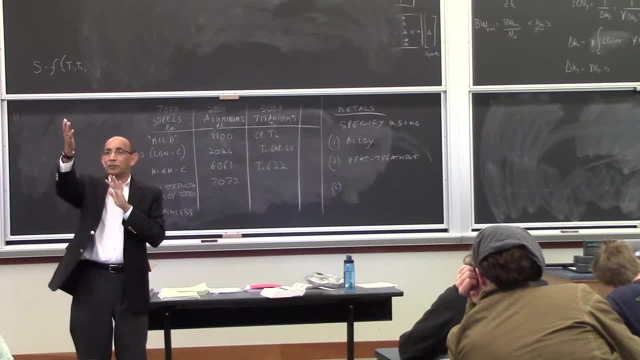 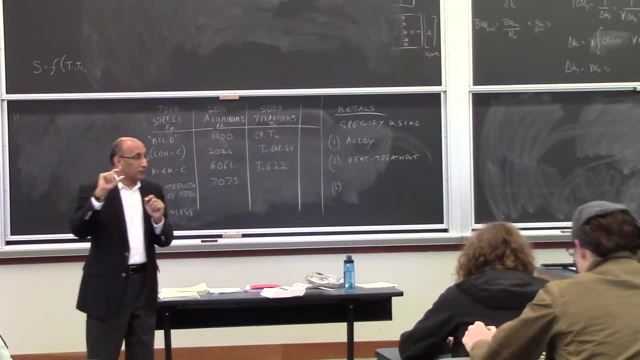 If you take a metal, so let's go back and look at the viruses and maybe come on top of all this. So the strength of an alloy, the strength of a metal, is determined by the easing with which you can move some defects to the back. those defects are called dislocations. And the easing with which the dislocations can move is determined by things like grain size, how big the crystals are inside the metal. If I take this thing and I heat it up for a long time, the crystals become very thick. then the strength goes down. 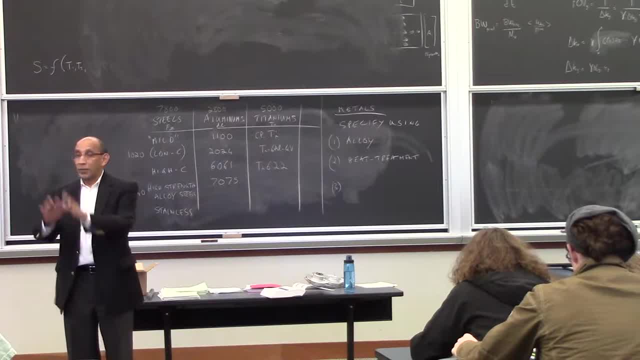 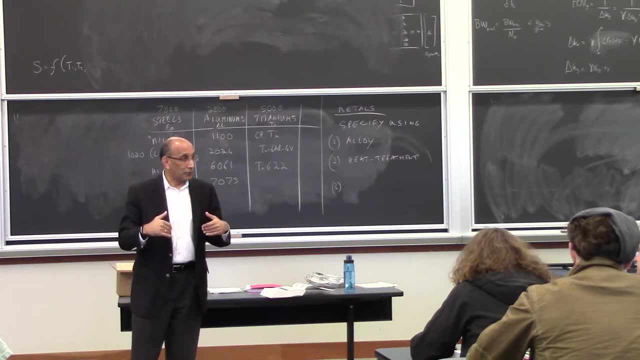 So it's the same alloy. all the compositions are the same. Remember I talked about if you store this thing in a very high temperature for a long time, the strength changes. that's what's happening: The grain sizes have grown and the strength goes down. 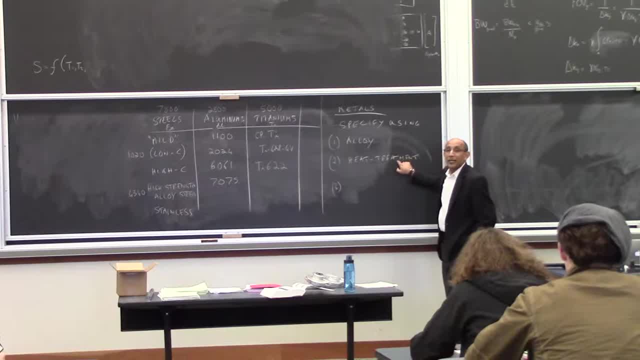 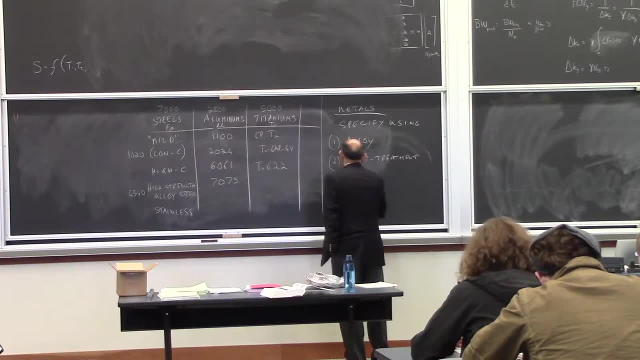 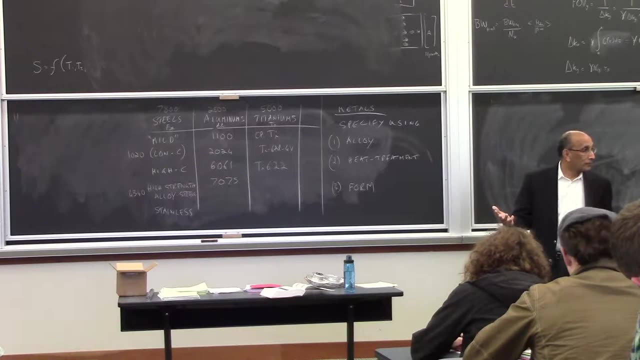 So the second thing you want to specify always is: under what conditions do you get the results? How was it treated? So the third thing you want to specify is the form of the alloy. Are you looking for plate or rod or strip, or what are you trying to buy? 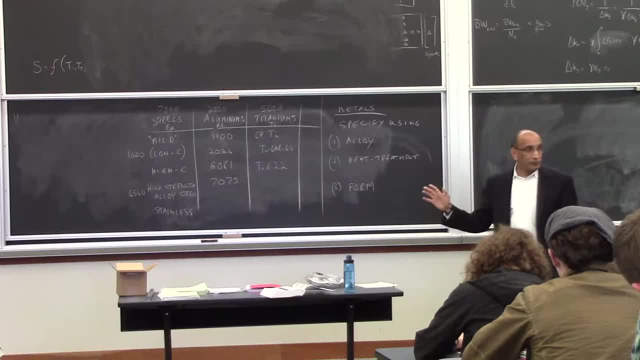 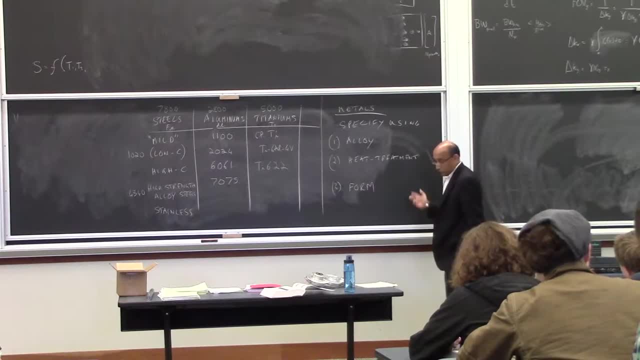 You never make an alloy right, You just buy it. So when you go to buy it, these are the three things you can tell them. So, to give you an example, with 6061, I have a number for that here- 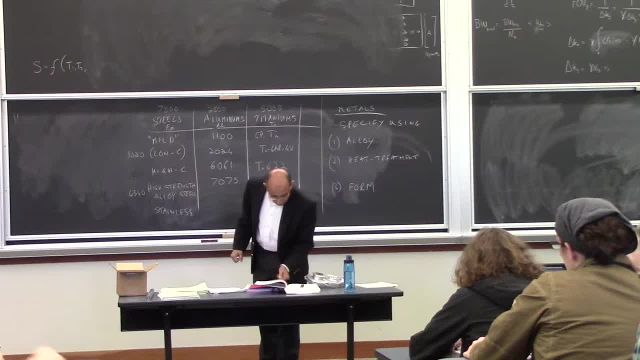 So this is the number, This is the weight. So this is the number. This is the aluminum, So this is the ratio, This is the weight, And there's also a certain amount of alloy coming out, but I'll just not go too far down. 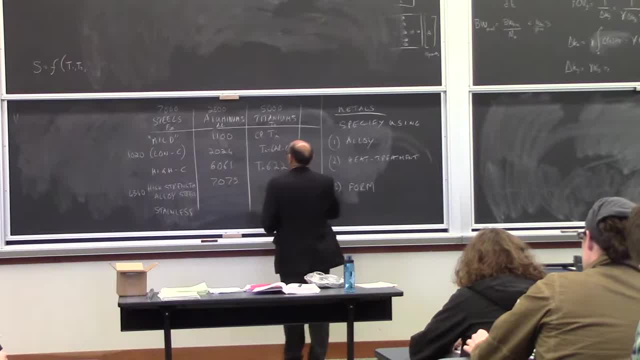 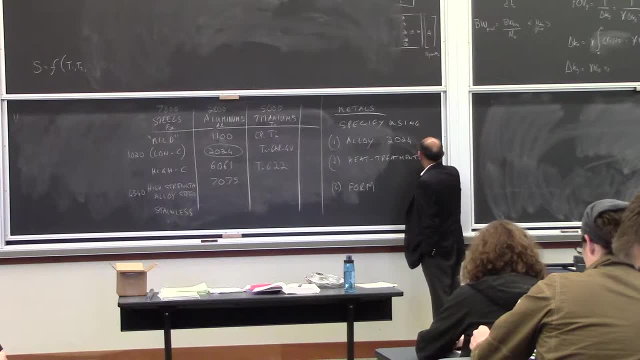 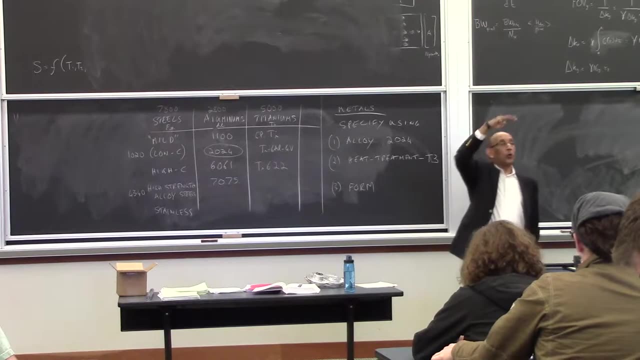 here. So you might consider this a 20-24 alloy. So let's take this case. You might specify an alloy as being a 20-24 alloy. You might then say: the heat treatment is T3. That specifies that you take this thing up to a certain temperature, hold it at a temperature. for some time and then cool it again. It's called an aging temperature. And then you might say that you want plate, So you go in and buy a plate of 2024 T3.. That's what you do, isn't it? 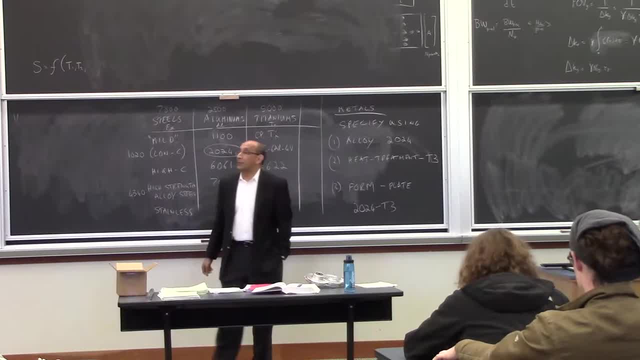 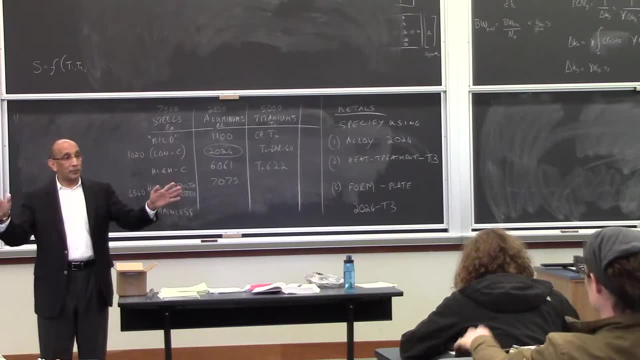 2024 O has a yield strength of 76 megapascals. So one's 346, the other's 76. So if you just go in and tell somebody I want 2024, and you don't tell them what heat treatment they want, 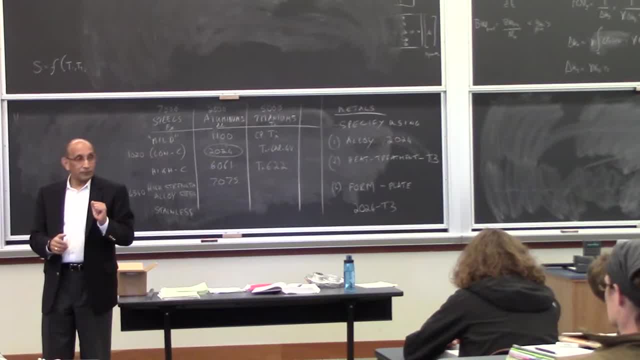 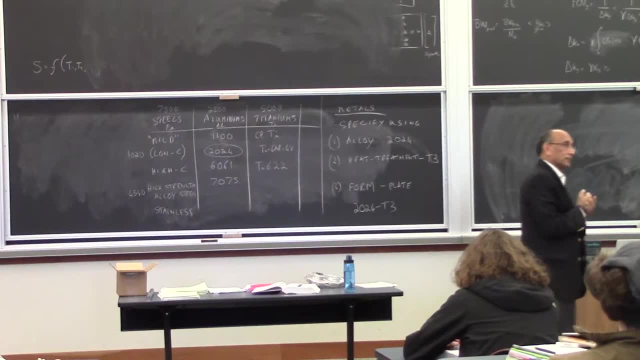 you might end up with something with a yield strength of 76. So you have to specify heat treatment. Why would you do it? in the effort of annealing it. So sometimes, when you want to make the plate, for instance, you might want to make it soft, of course. 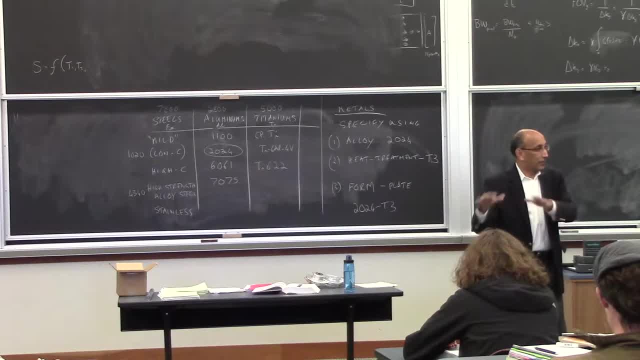 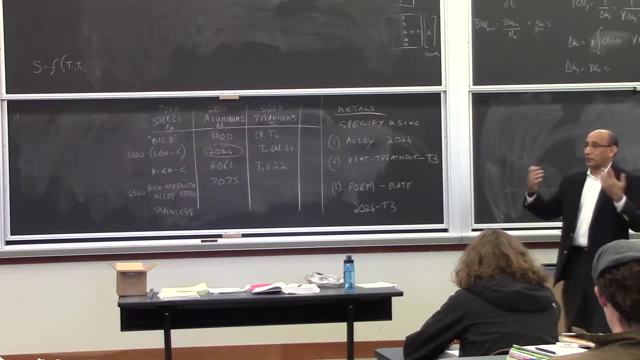 then hammer it into a plate, then heat it up And get a T3 condition to increase the strength again. So there are times when you want it soft. Most of us on the mechanical engineering side we're going to buy it and use it if we want it soft. 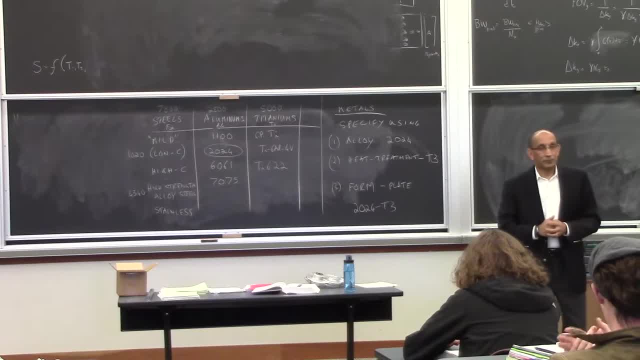 But when you're making the thing, you may want to make it soft. The other thing is the really hard. things are hard to machine. So let's say you want to machine something of a particular shape. You may want to machine it while it's soft and then heat treat it. 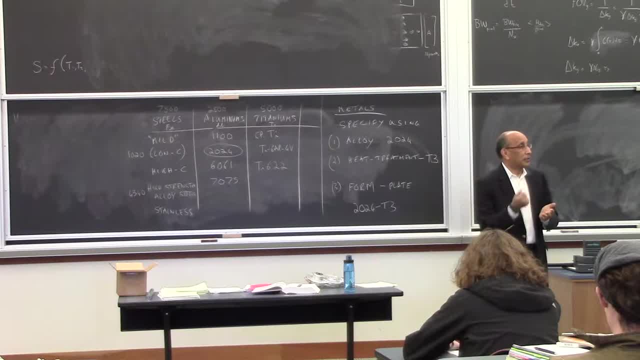 So those of you who remember seeing how people make soaps: you heat it up, you hammer it, you make it the shape you want and you quench it. That's the heat treatment That makes it hard. All right, So everyone have a key idea. 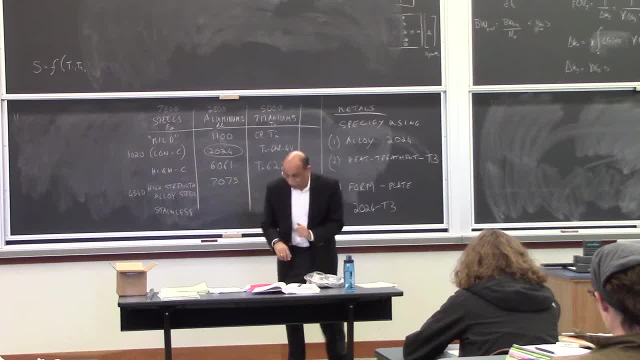 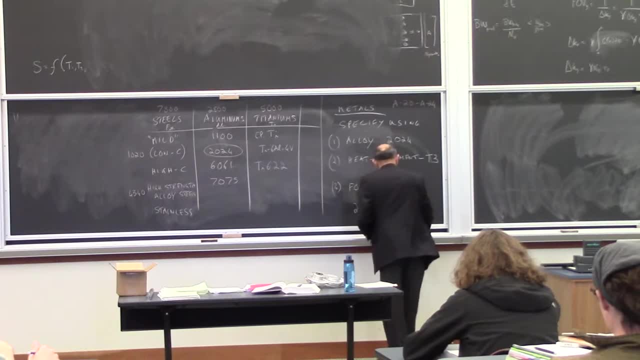 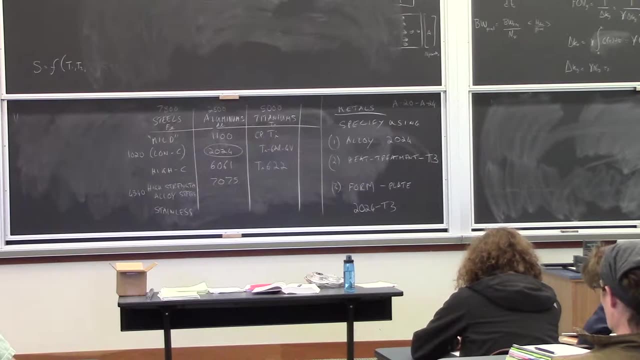 We'll go through this in more detail when Nia comes through, But just make sure you look at the right places in the book. So, A20.. Thank you. So we're going to shift gears now and talk about shafts. So we're going to shift gears now and talk about shafts. 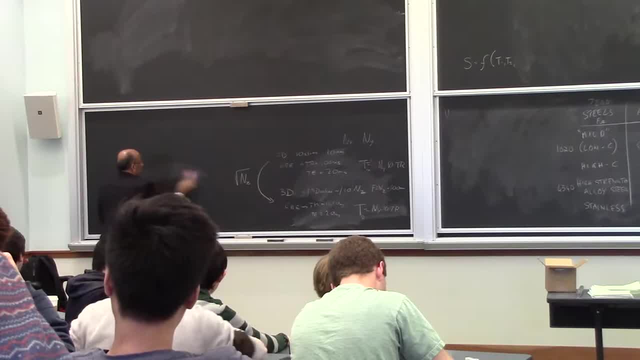 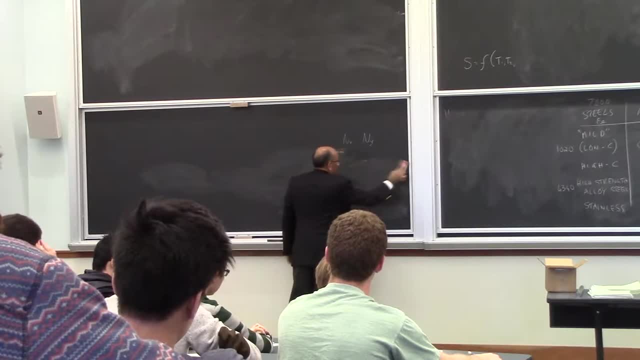 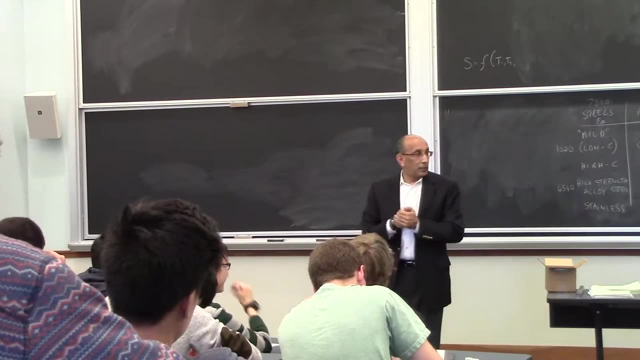 There was one question about the midterm. So right now the midterm. the second midterm is scheduled for April 17th. Can you keep this up? So So what's the next week? And I thought that you guys have another exam on the 20th. 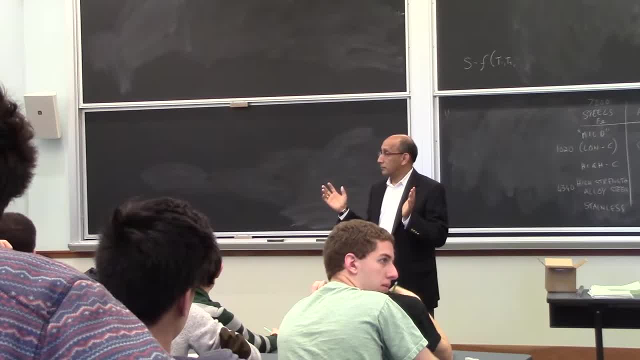 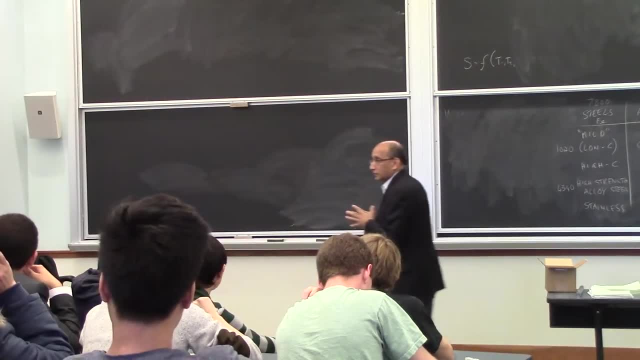 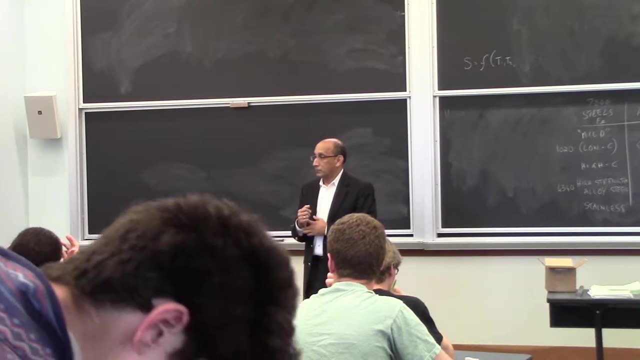 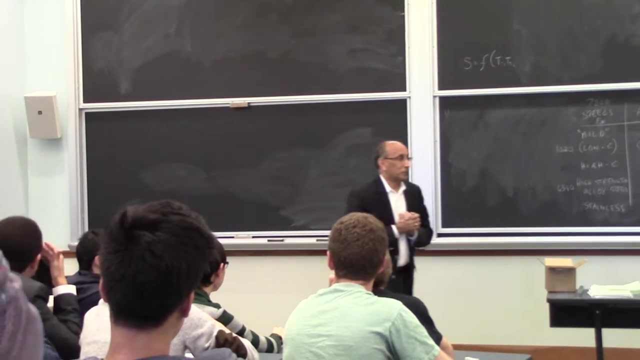 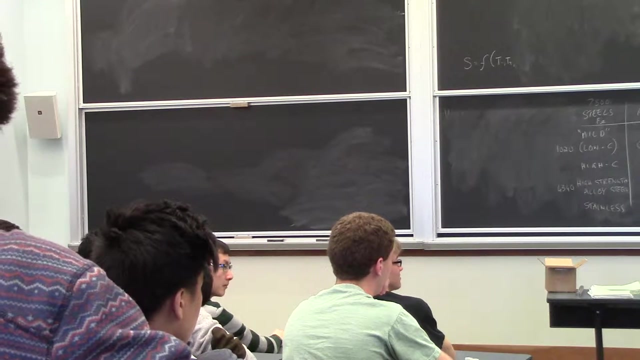 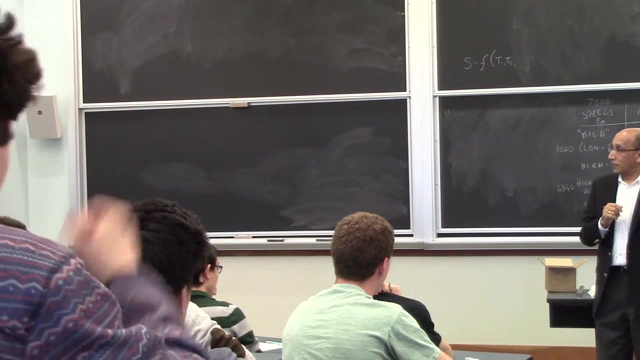 So what is that? What's the next week's exam, on the 20th? Who's the instructor? All right, So I'm going to email it to some other TV players We'll visit. Okay, Thank you, Just give me one. 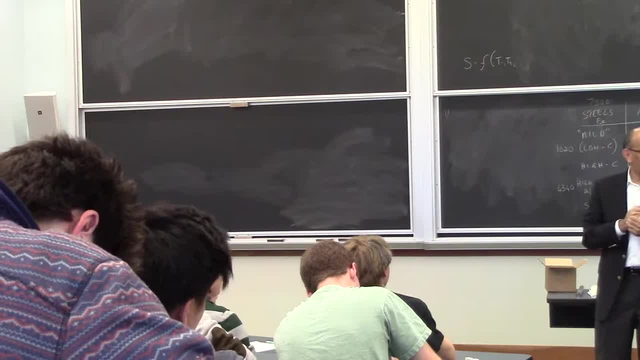 One second, All right. So all right, We'll focus on right now Until I tell you otherwise. OK, All right, So we'll get back with you guys in a minute. All right, We'll get back with you guys. 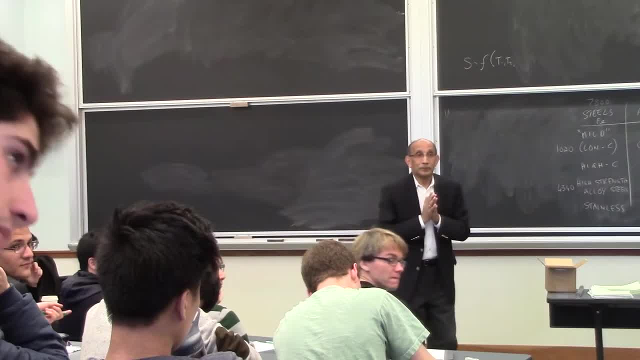 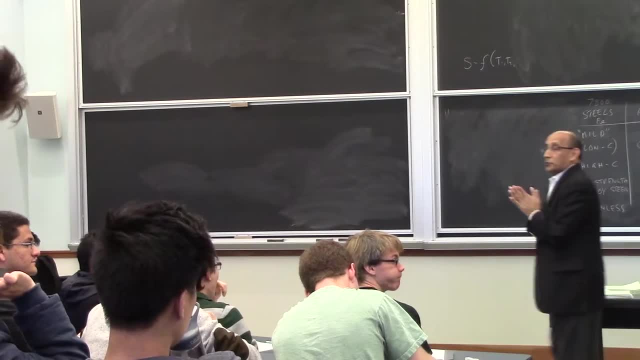 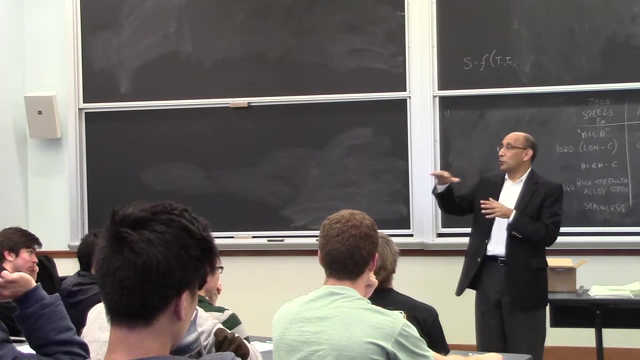 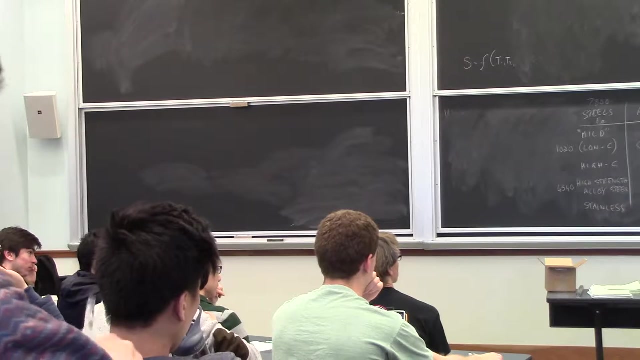 OK, Thank you. Thank you. I also sent out emails to some of you if you were in danger of having, let's say, a low D or heading towards an F, required to provide feedback to the academic advising office. So some of you may get emails from them. 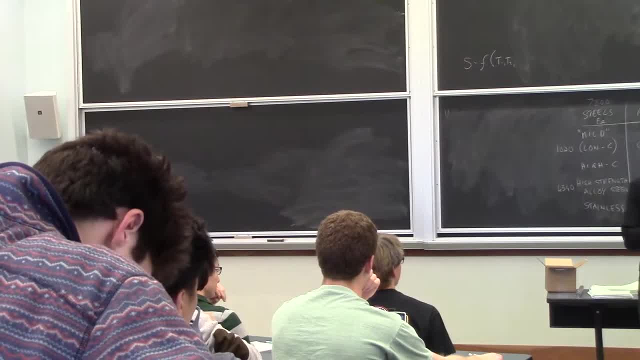 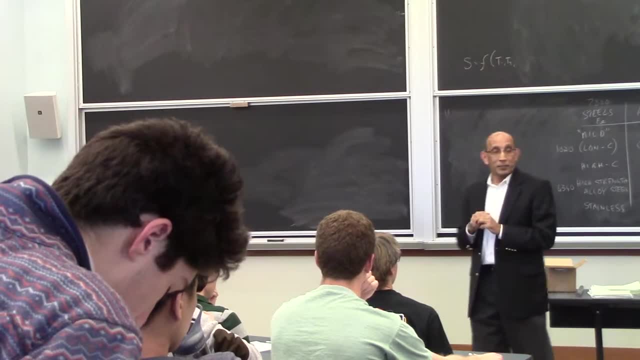 I remember what I said: if you got less than 35 in the final grade, but in the grade for the mid-term, you should have an appointment with me. You should talk to me about what's going on there and how I can help. 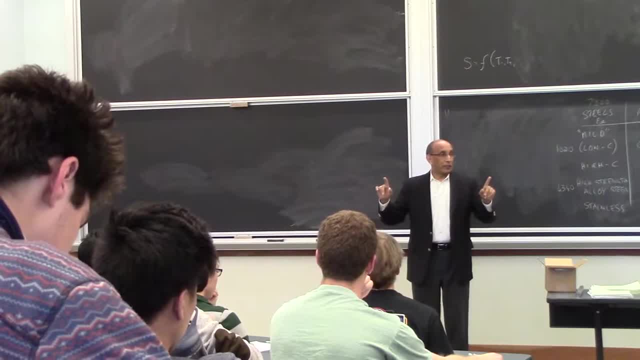 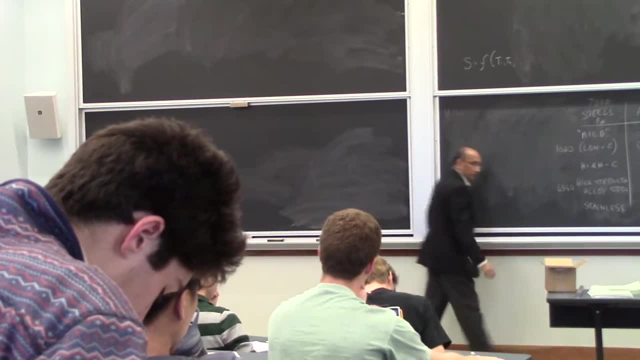 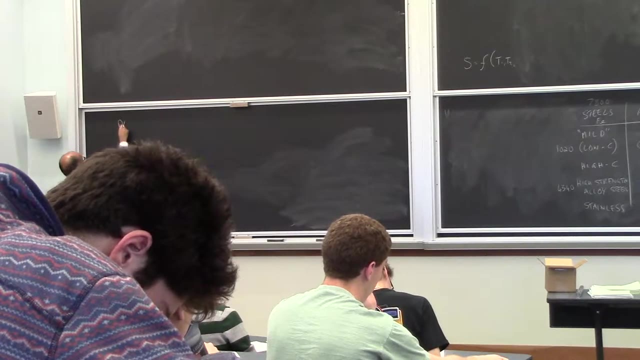 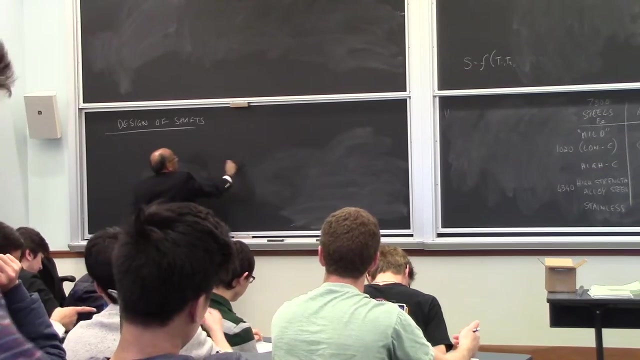 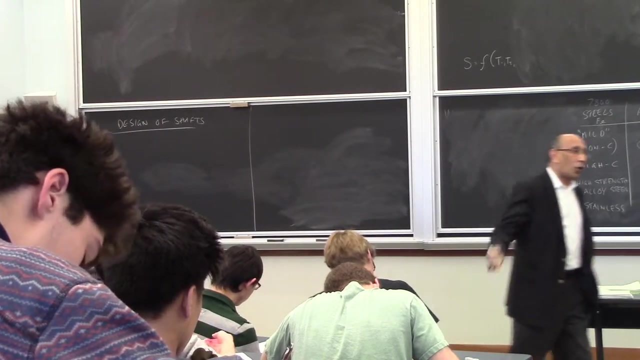 Any other questions before we get back into class? I know we've gone through So push-ups. The reason we're talking about shafts right now is because it's a great example of where they can break all the things we've done so far together into one. 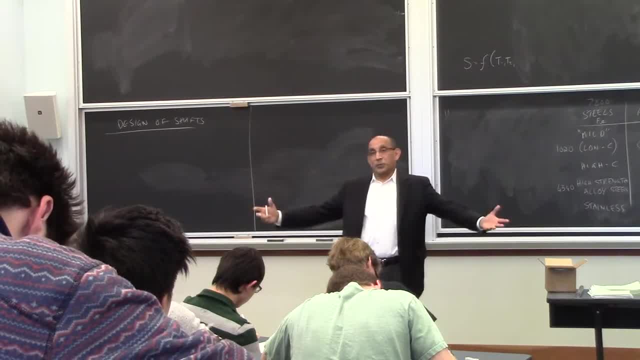 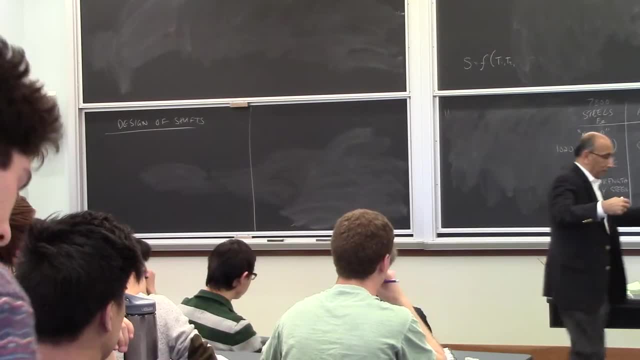 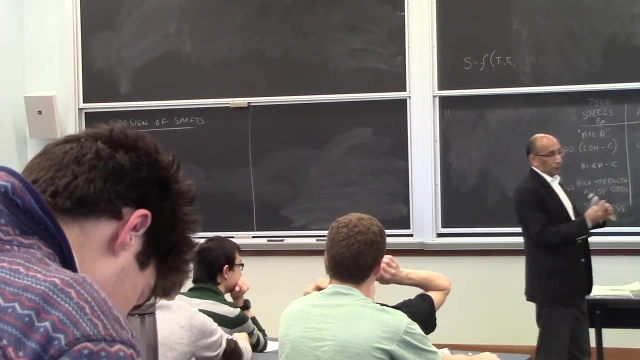 So a shaft is essentially a rod of some sort, typically rotates. that's what we call the shaft. Otherwise we just call it a rod, And it's usually carrying torque. So I don't know where we got this from, but here's an example of a shaft. 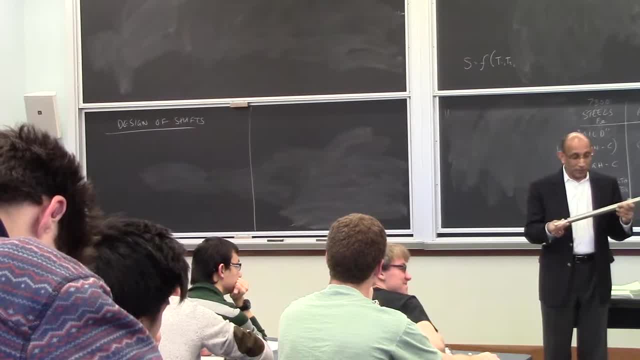 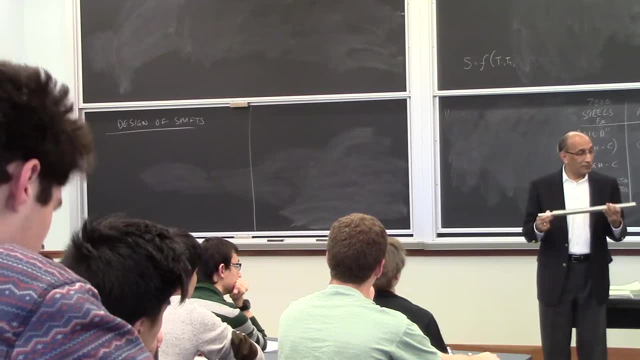 This is a bar, All right. So we let one of the bar head people tell us exactly what it is. All right, This is stainless steel 17-pulse. When did you say, Oh, we'll come to that later. 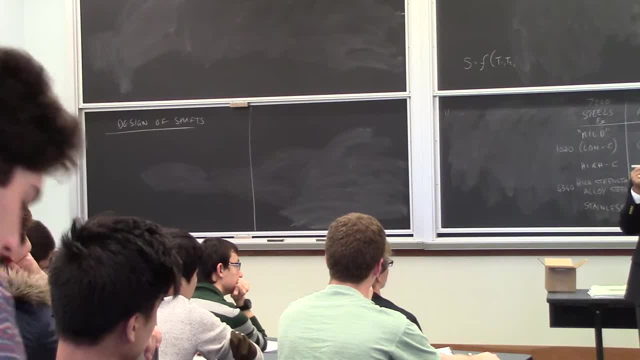 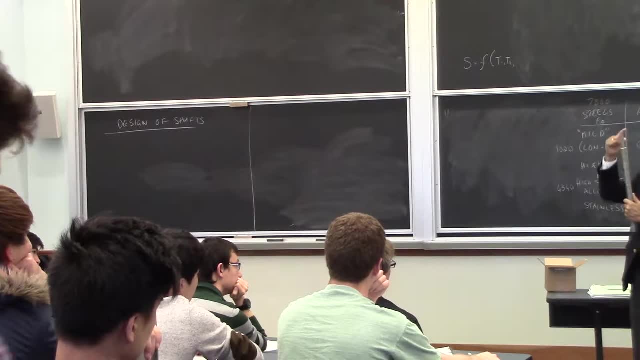 It's got Some grooves come into it. You should ask why you have the grooves So typically they're key waves. It's got grooves. It's got changes in cross-section. You can see it's narrow, then it becomes fat. 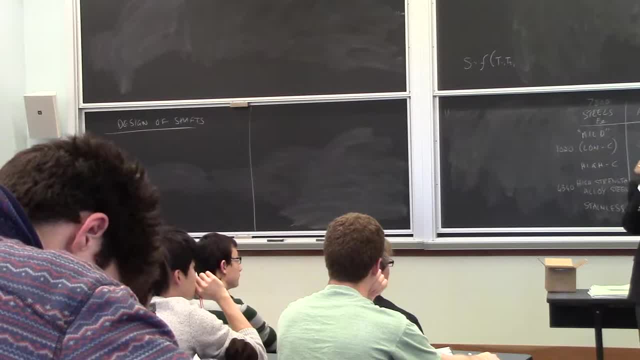 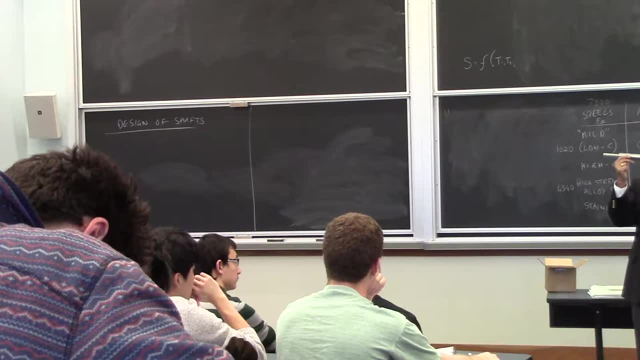 Clearly it's got a stress concentration when it changes cross-section. I don't know whether you guys have thought about that stress concentration or not, Something to think about, So you put a lot of stress concentration into this thing. So if you think about something like this, right, 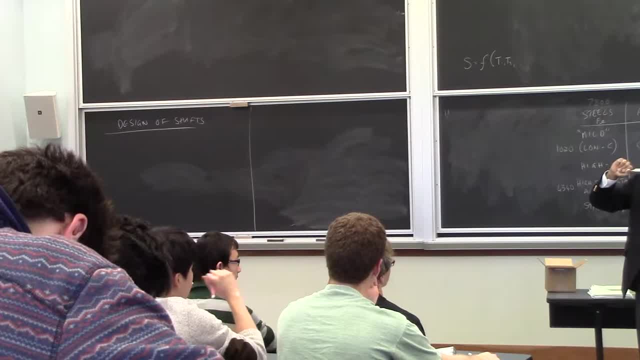 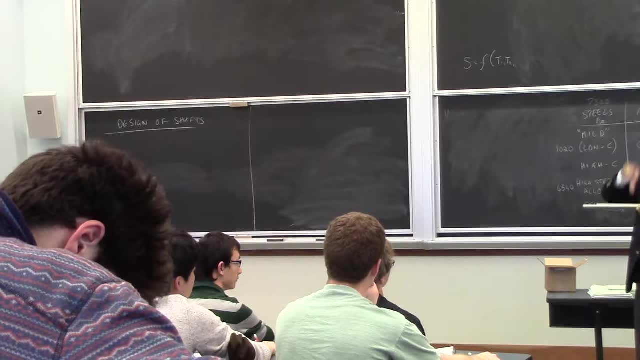 It's going to be put in torque in torque. So you're going to apply torque, So you are putting in torque in torque. Typically, it's got its own weight. We've tossed this around. It's pretty heavy. You're going to put gears and things like that on it. 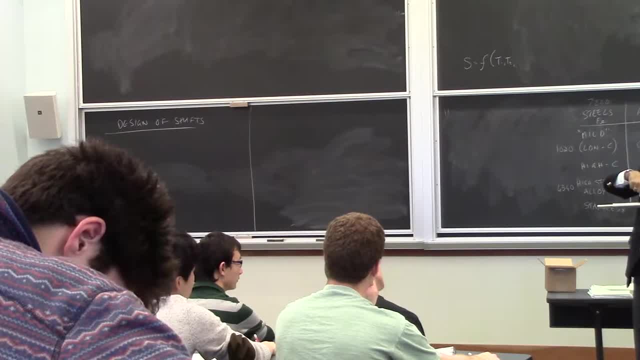 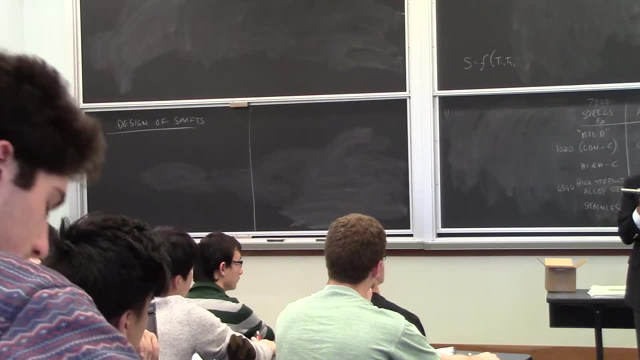 Those have their own weight. So you've got forces acting this way, So this thing is also in bending, So you've got torsion and bending on this one shaft. So let me actually pass it around. We'll start with you guys. 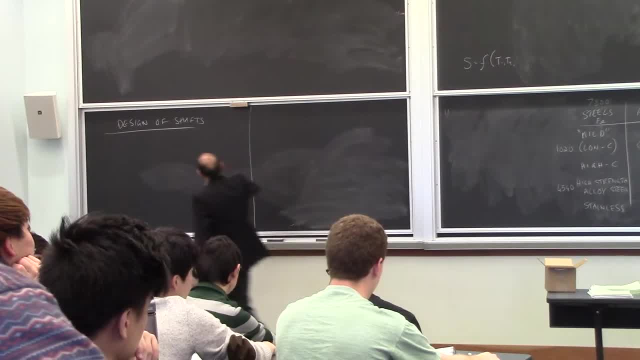 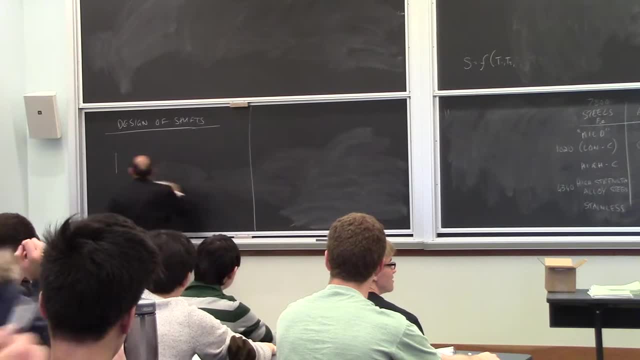 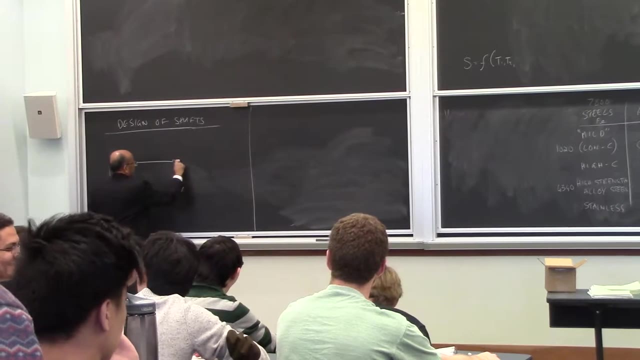 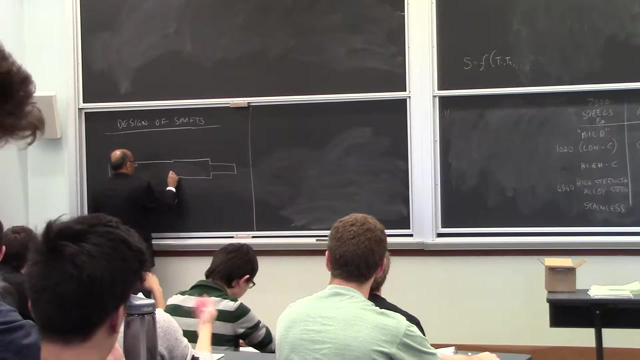 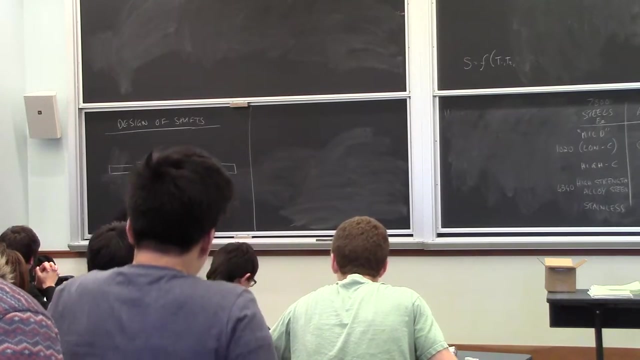 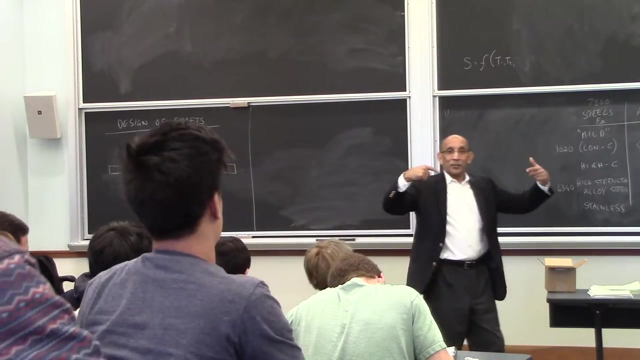 Please don't swing it around, Just pass it. Let's take a look at the difference of size. Imagine something like this, So this might be what it looks like. This is a piece of luck. It is access to the metric meaning you can generate. 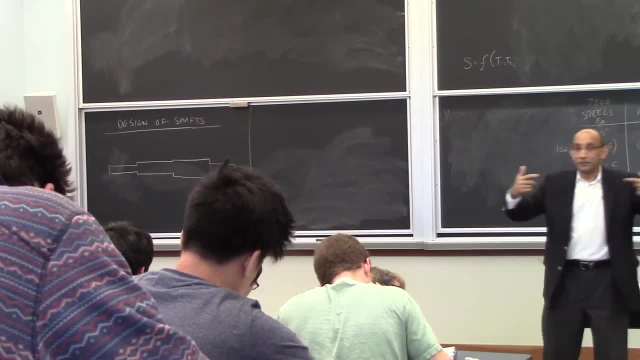 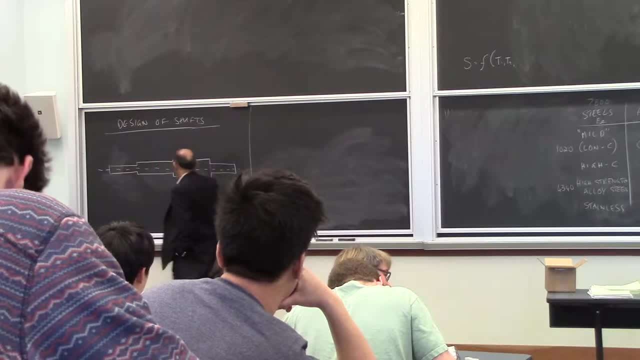 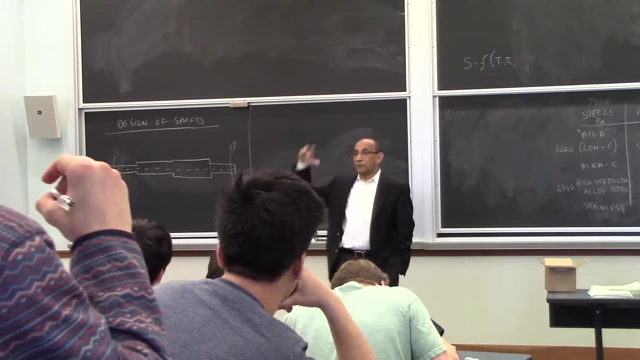 it by spinning it on a lathe, for instance Right. So you've got an axis down there. You're applying a torque. You might apply the torque typically through gears. The gears have to be mounted somehow, So you're trying to. 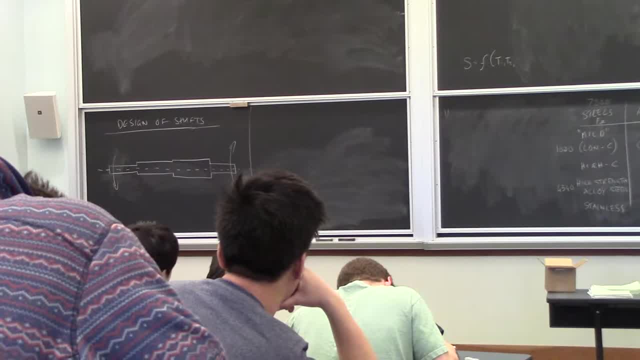 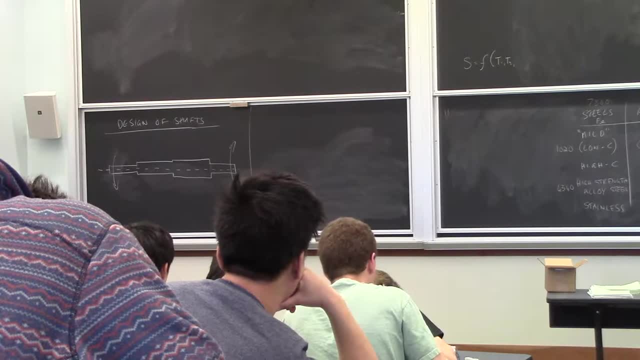 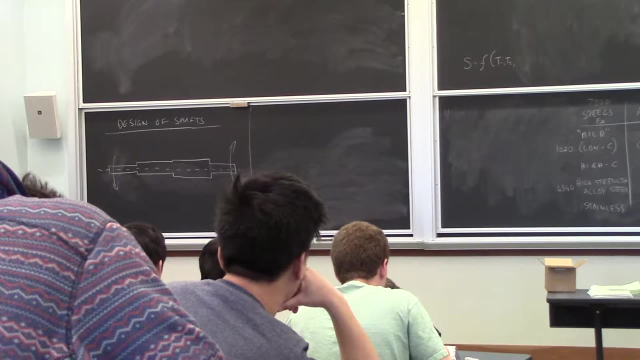 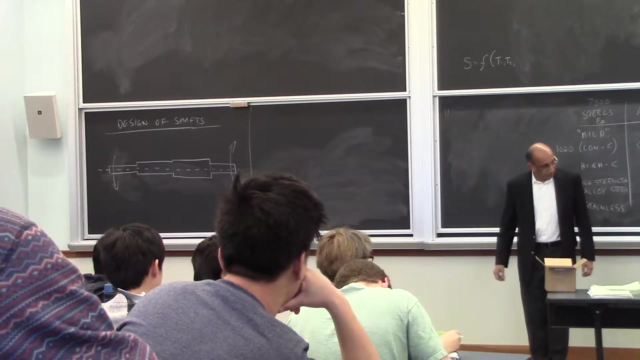 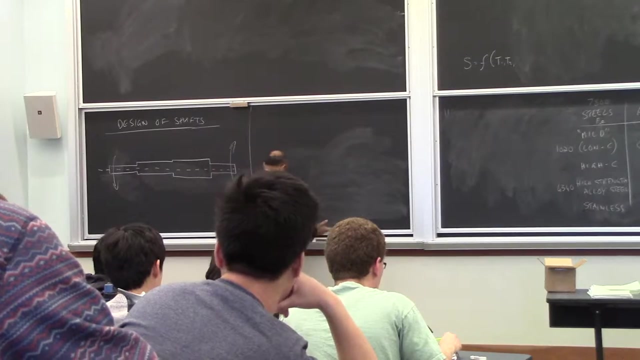 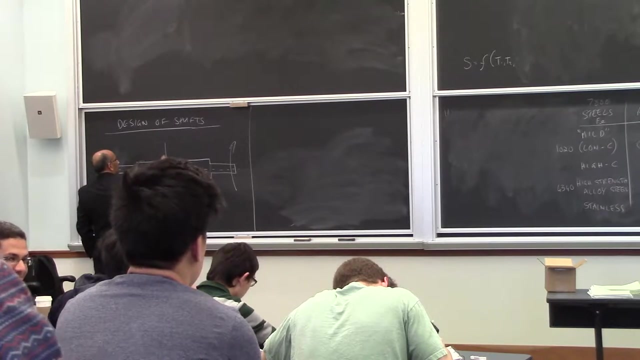 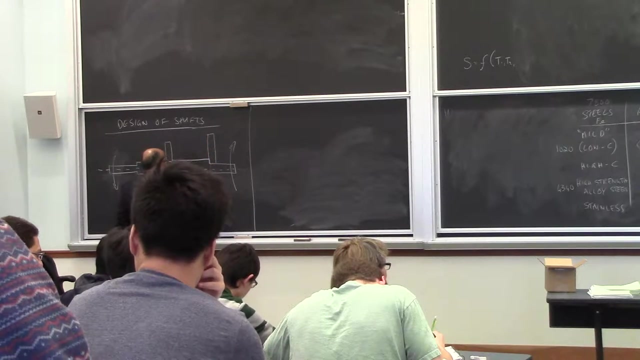 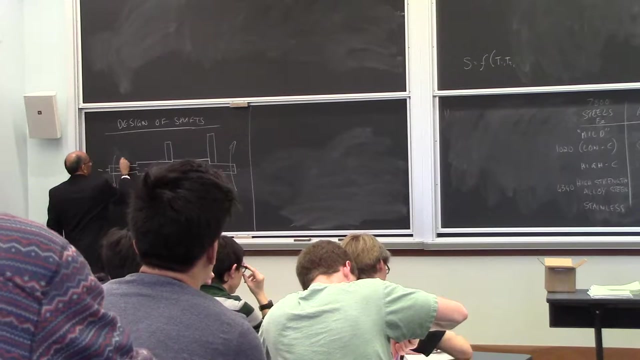 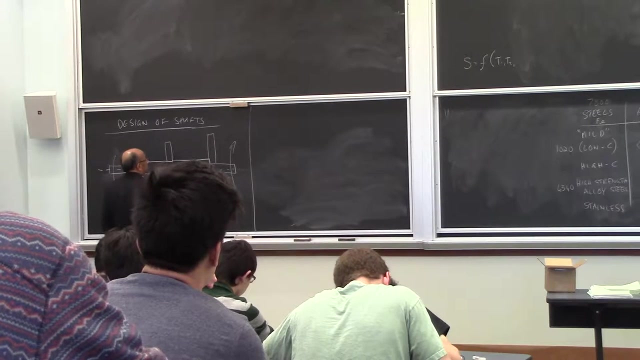 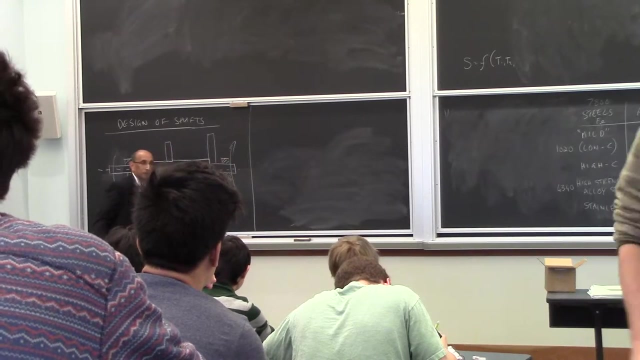 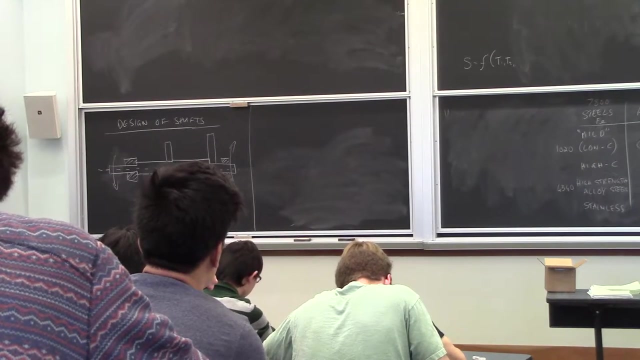 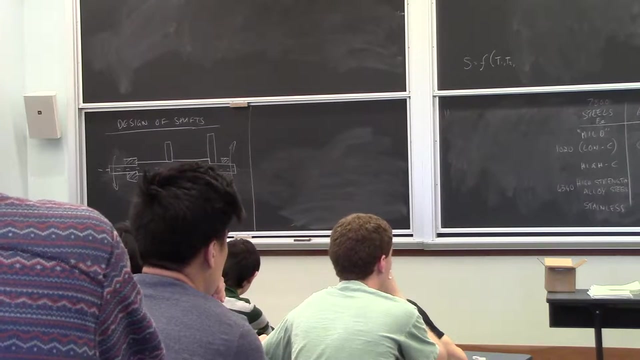 turn the gear without having it slip. with respect to the torque. 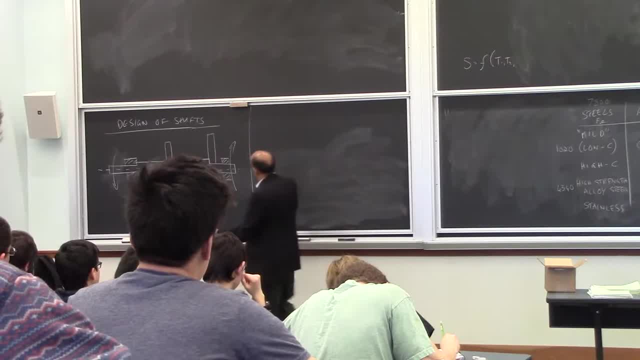 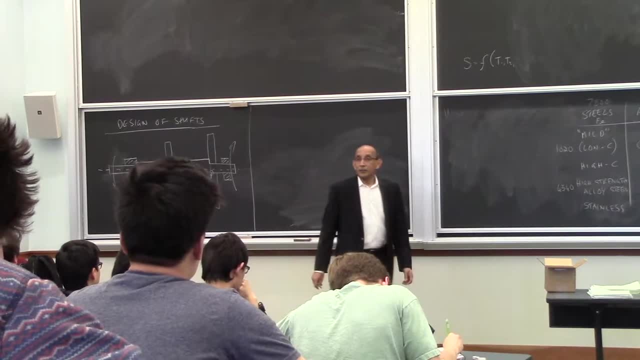 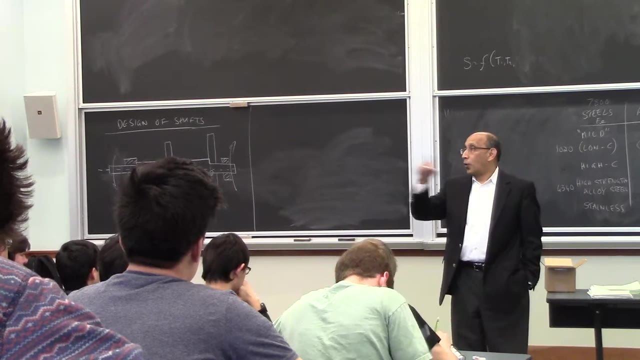 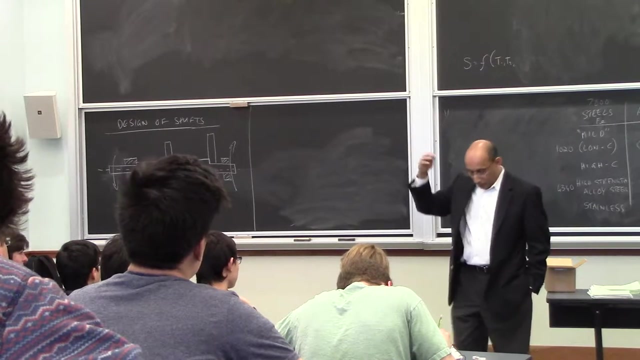 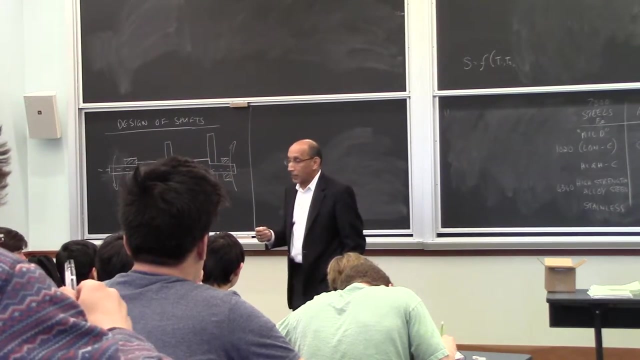 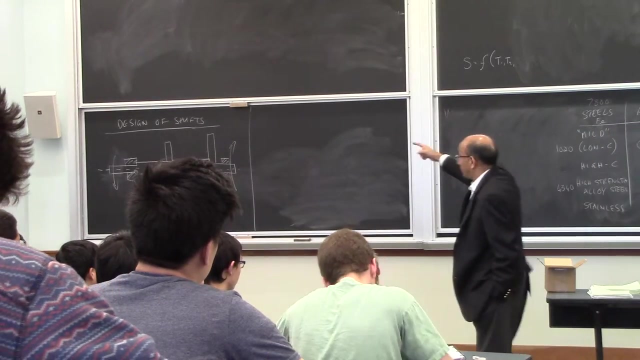 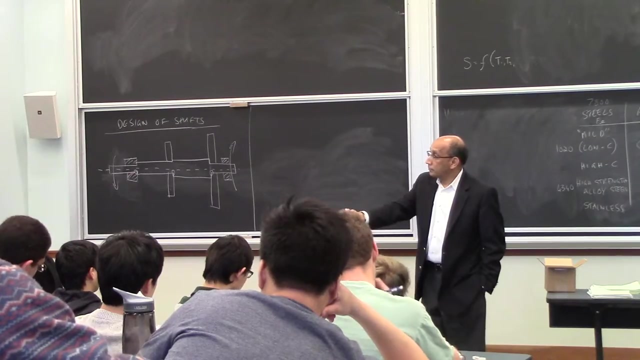 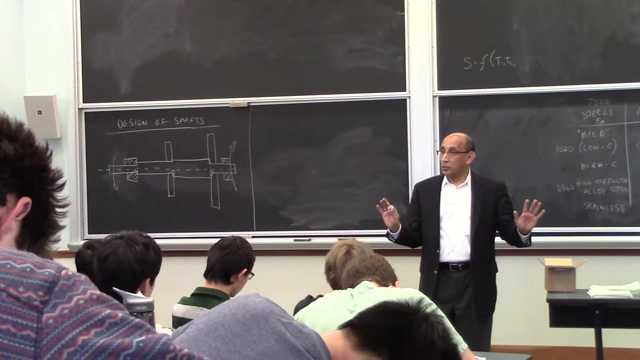 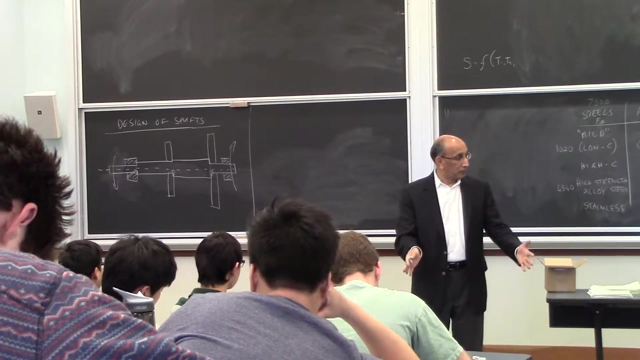 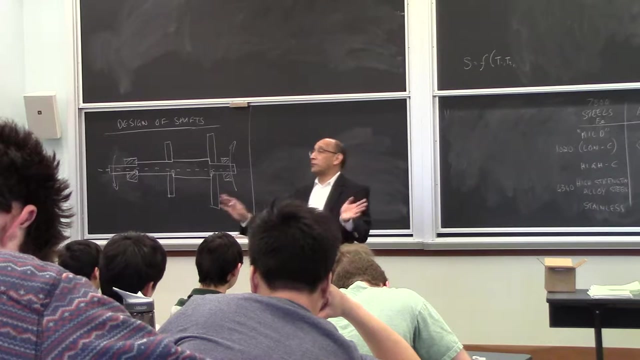 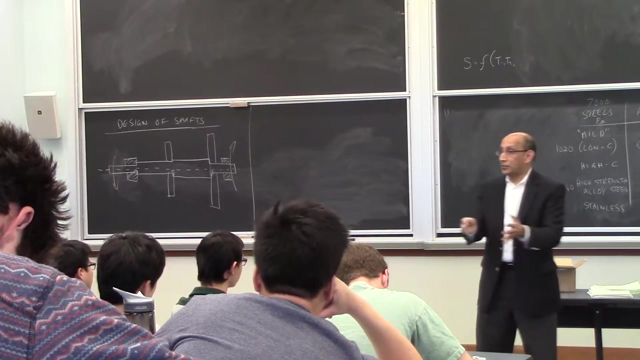 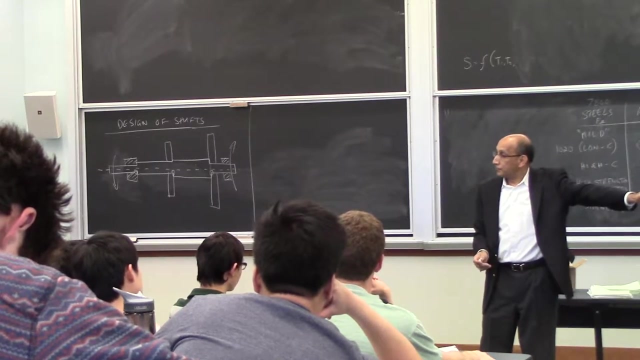 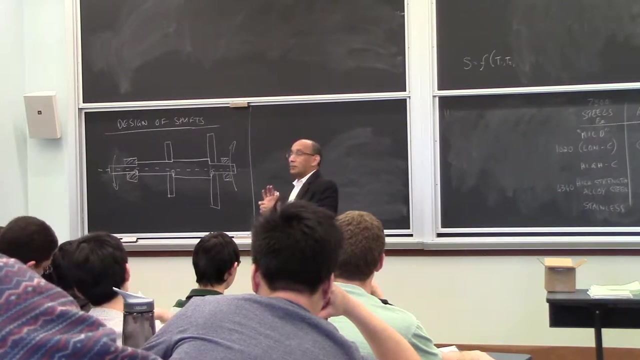 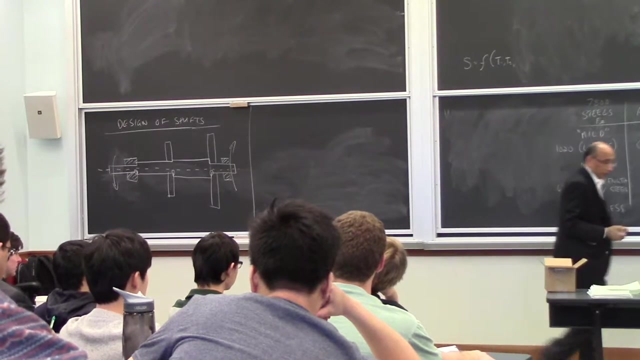 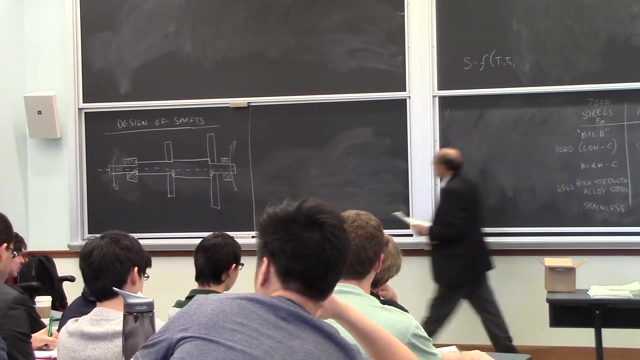 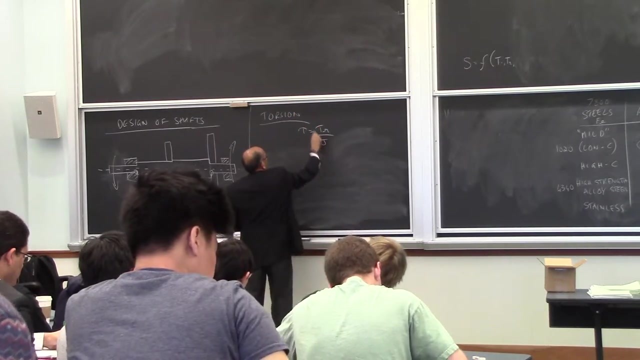 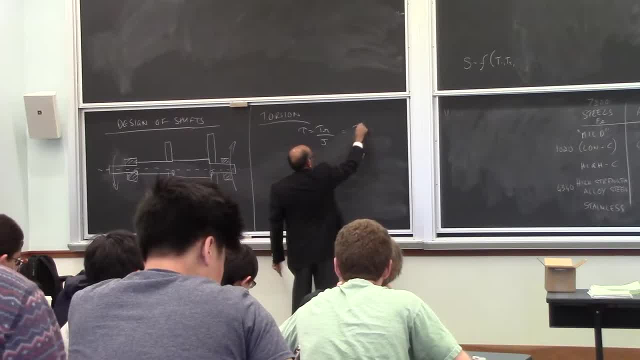 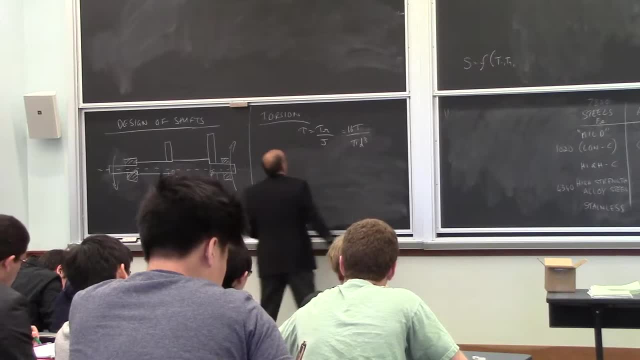 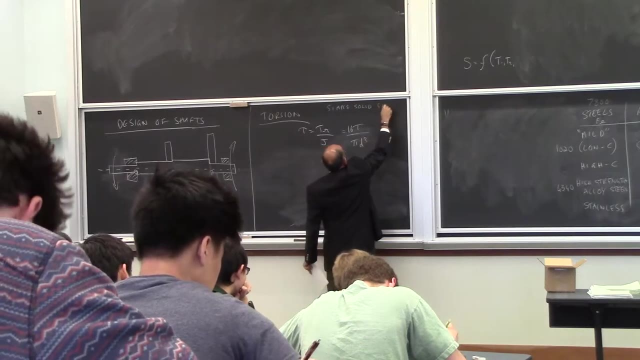 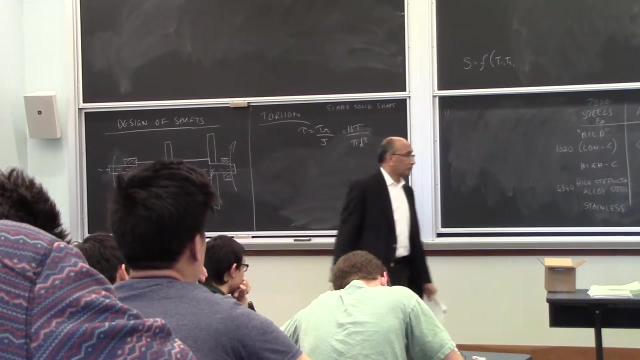 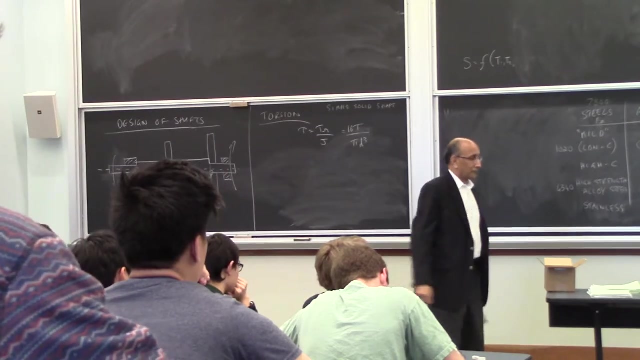 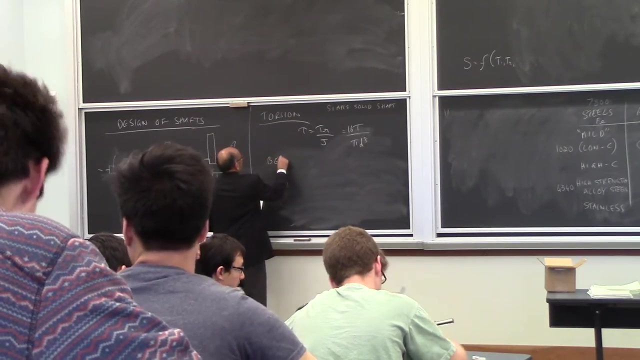 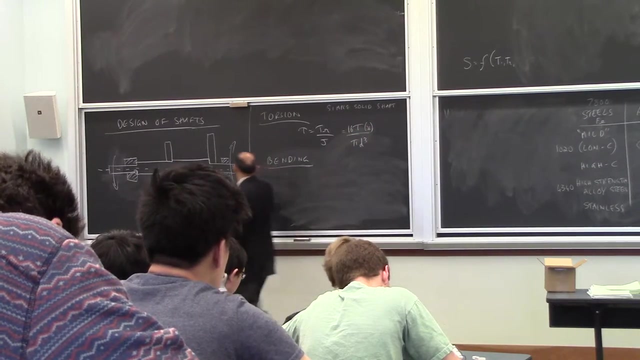 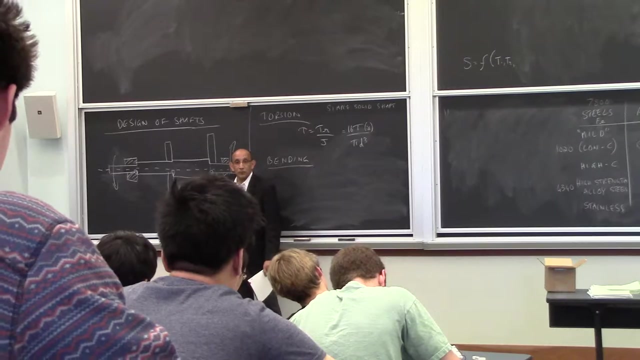 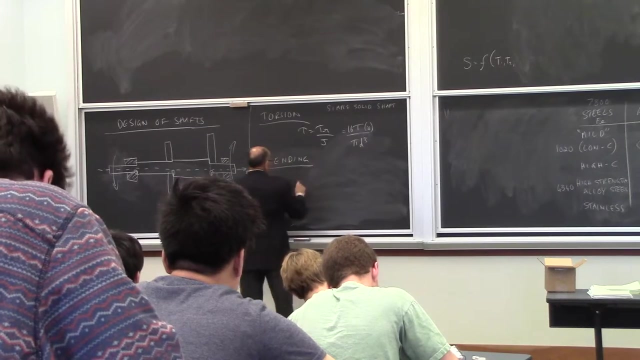 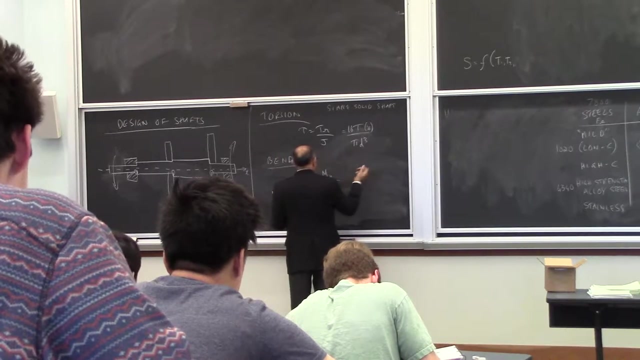 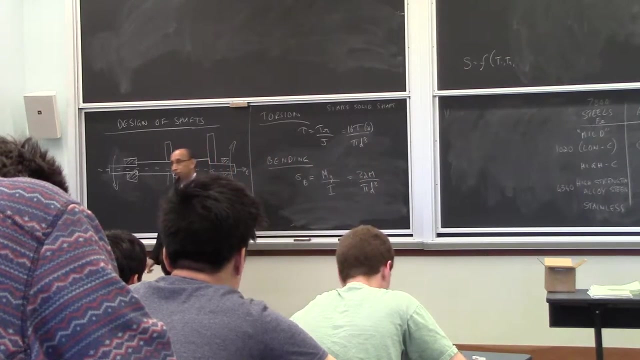 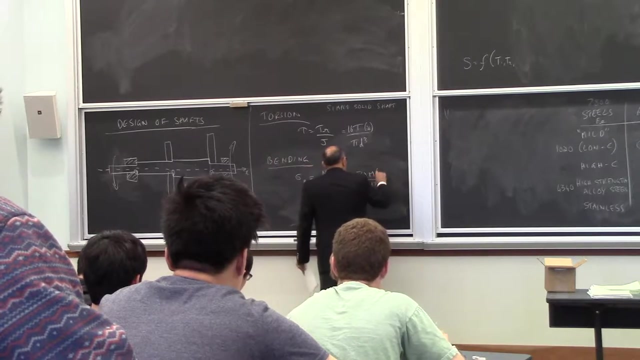 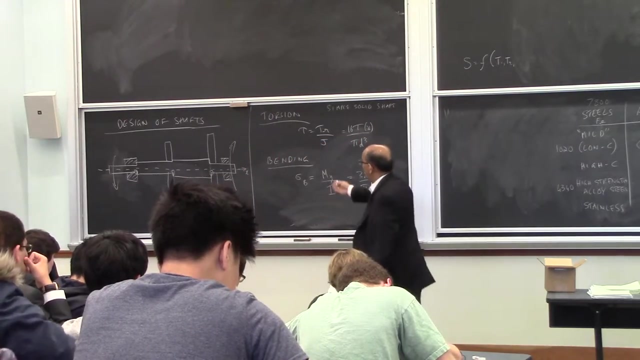 m over pi over 2 for a simple common check. But that was the function of x2.. So if you think about this right, 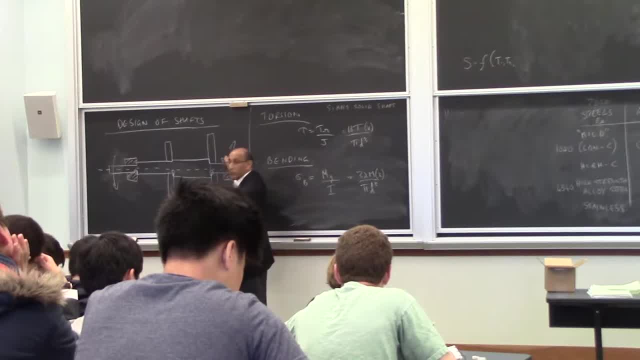 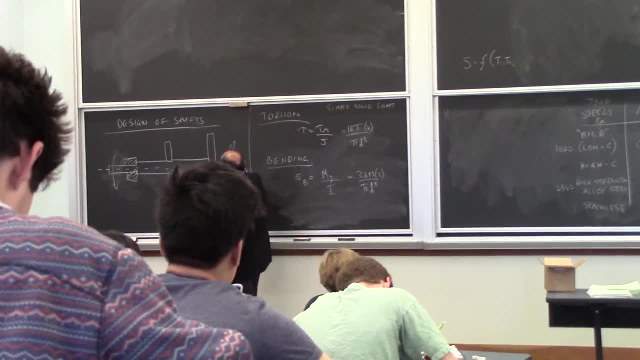 Forget the dark at the moment. These are. that is the way of supporting it. So these are like your simply supported set, Except it's able to go, And these are also the dark side. There's all the weight that's being applied. 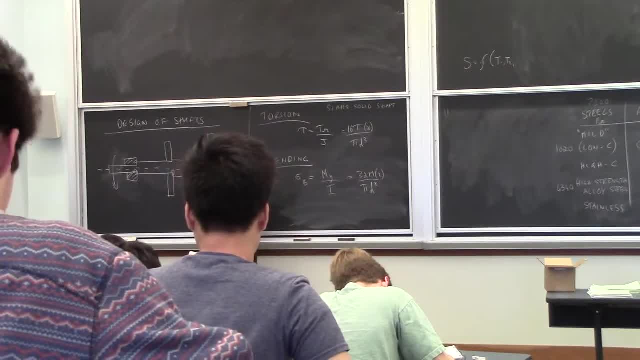 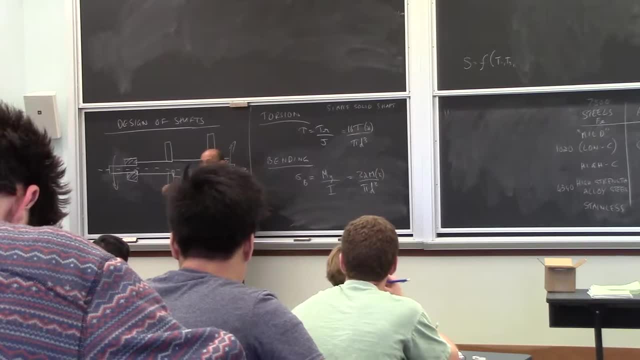 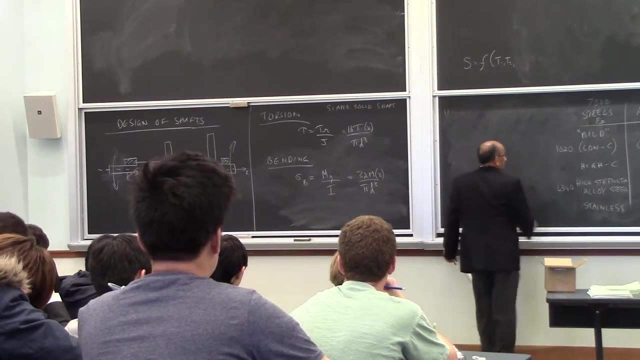 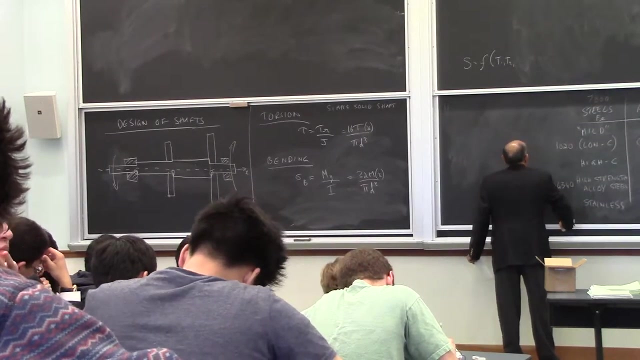 So the weight of the shaft is like a uniform load, A uniformly distributed load. That's how it works. And then you have the weights of each field, Which I like to point out. Okay, so that's the better case of You may have a tension load. 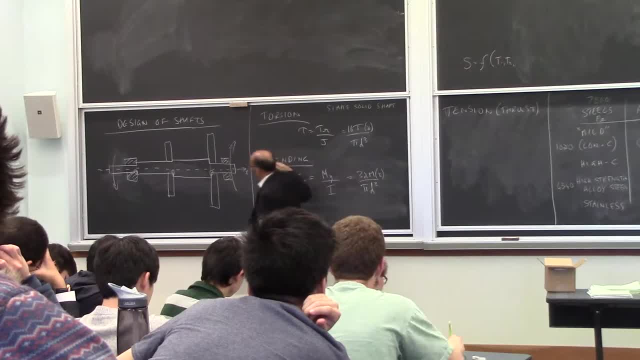 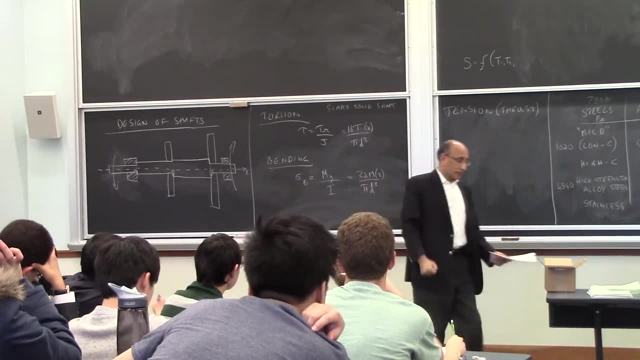 Or a compression load, It's possible that you have something pushing on the shaft this way, Along the axis. You'll find that most often when you have vertical shafts. If you're running a shaft vertically right, You'll find weights that are also acting along the length of the shaft. 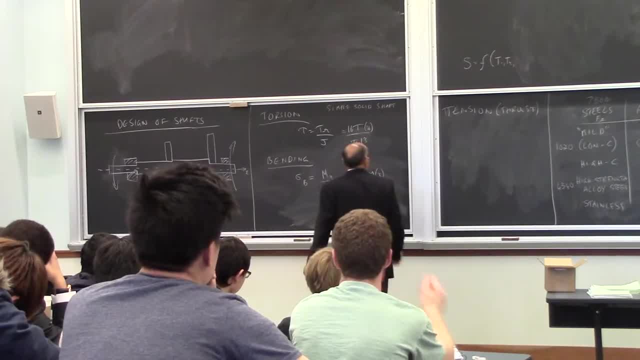 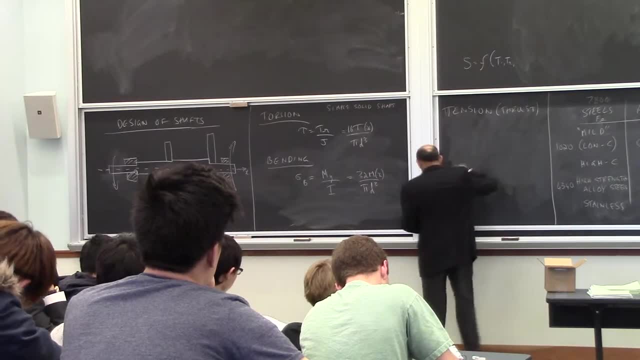 Typically for horizontal shafts. you don't often have these, They don't happen. We call them cross loads along the axis. So a cross load, you know what is this one. First the tension And then just the force of gravity, right. 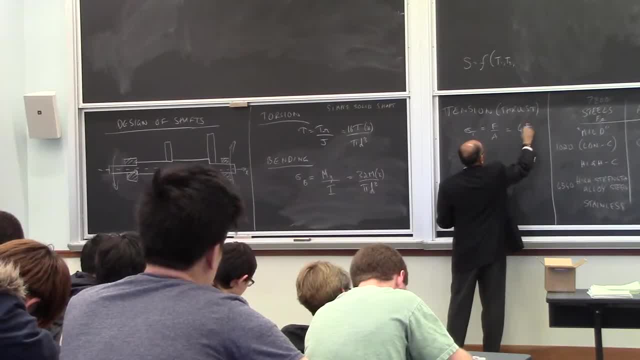 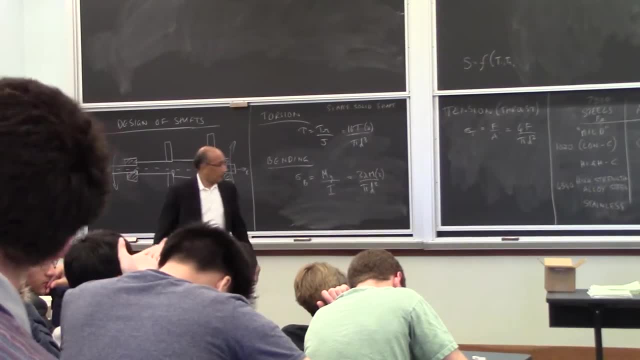 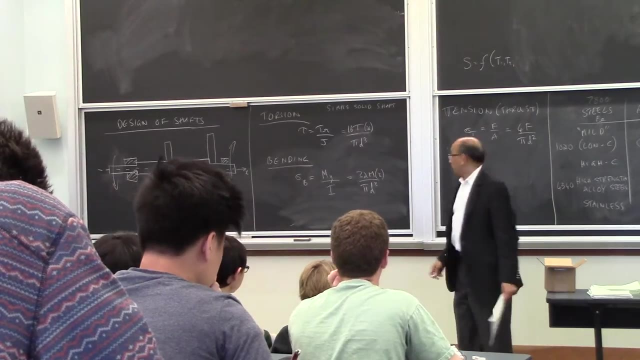 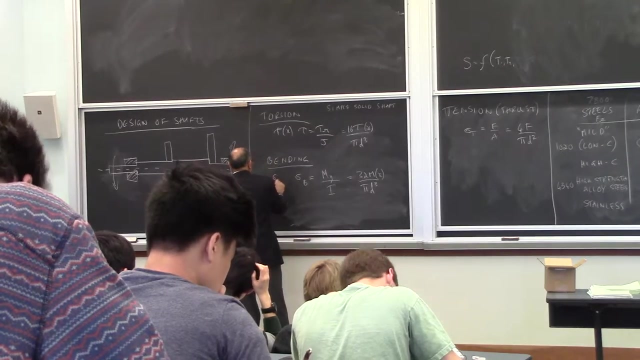 Which in this case would be. That's it. It comes under stress. So tau is a function of x, Because t is a function of x. Sigma v is a function of x. Z plus z, M is a function of x. 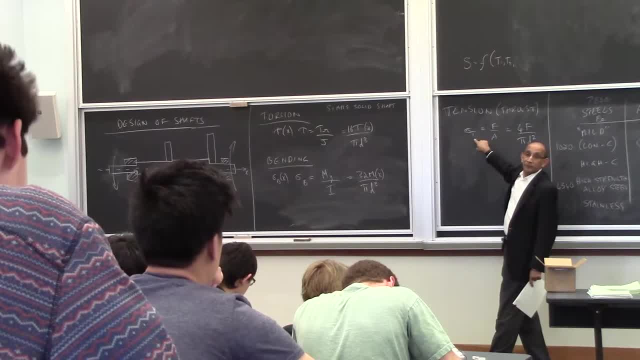 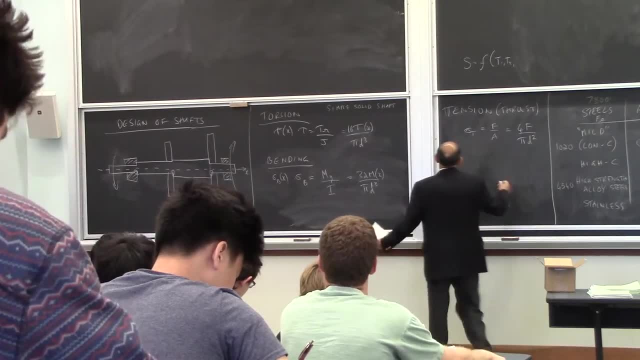 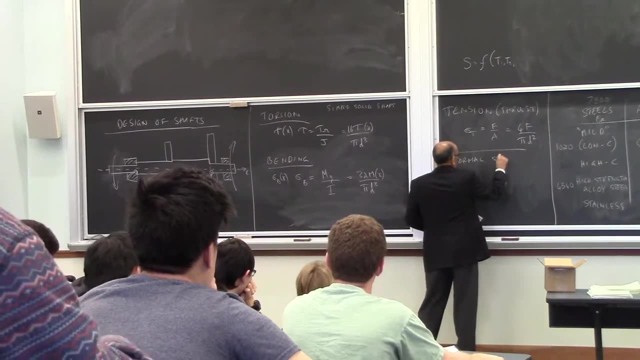 Sigma t is usually not a function of x. But you have all the stresses. Now you just have to decide where is the maximum, How? If you were to look just at the tensile stresses Or just at the normal stresses, That would be some sigma equals sigma v plus m. 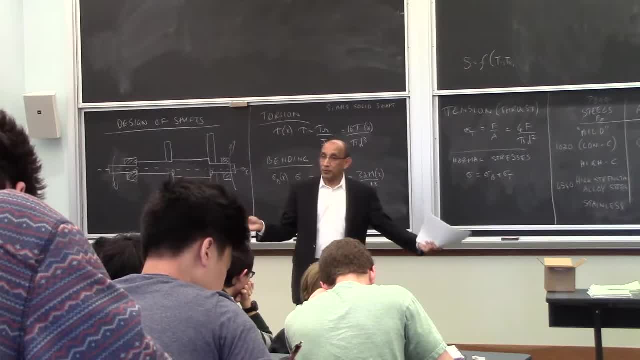 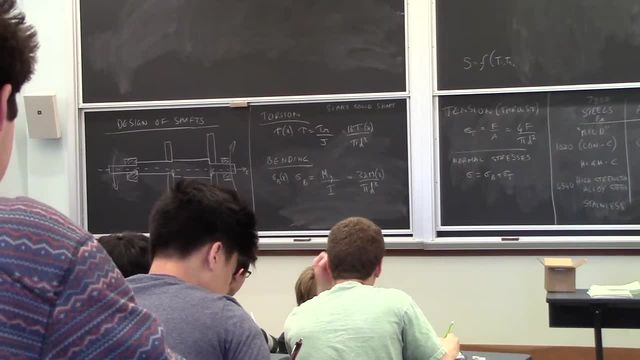 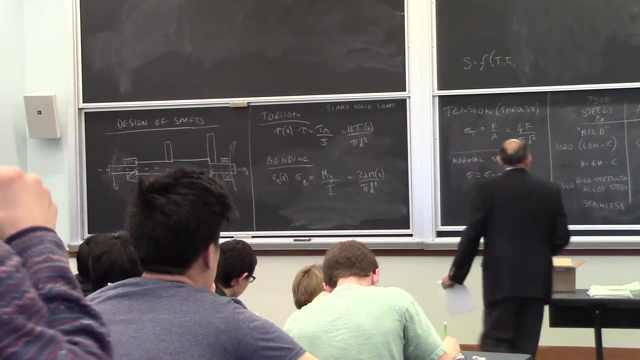 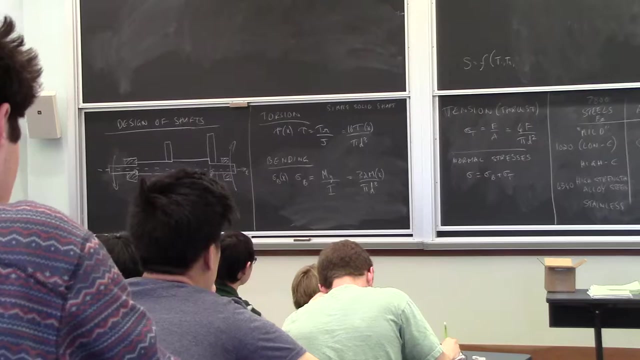 But you have no tau, Neither the stresses. There is no class to go there. sigma v: That's the beam problem. It's not the normal level, It's just a beam with a non-functional section. Right, This is what we have compiled here. 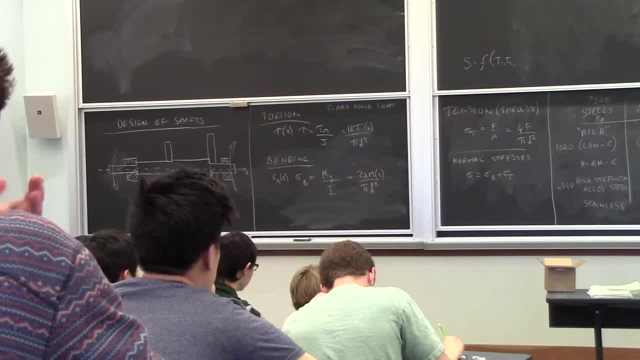 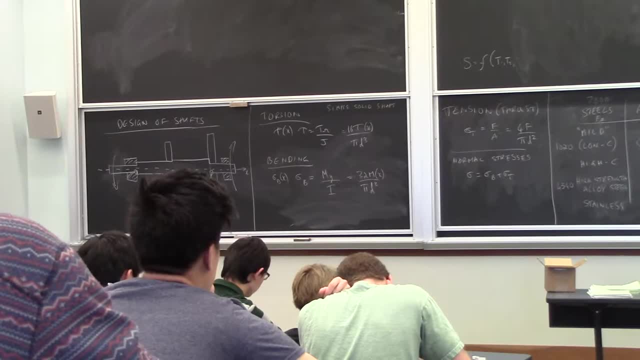 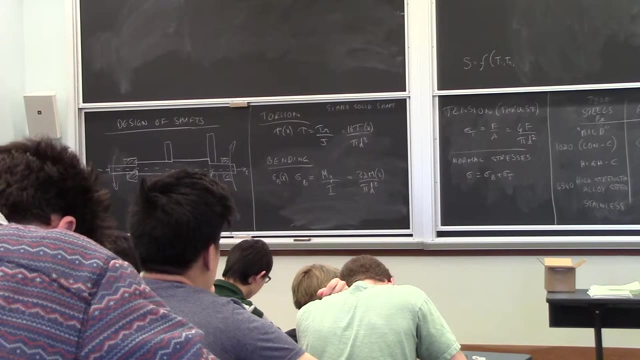 All of those are on the same time. We've done this before, We just want to do that, So I might decide I want to use a stress column In which the ischemia would look like: tau max equals sy over 2n. 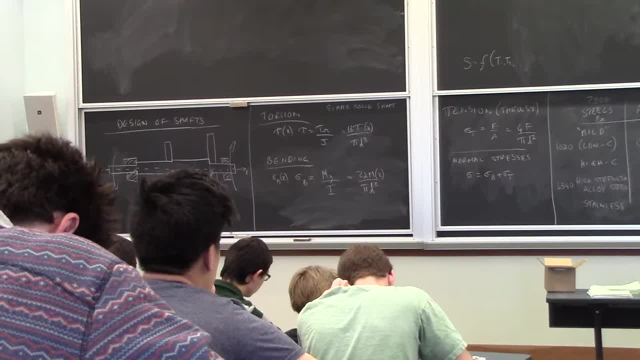 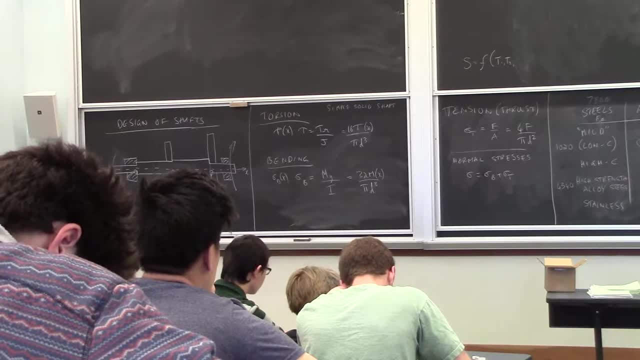 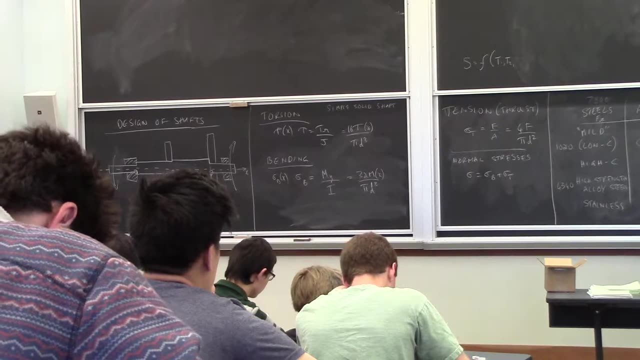 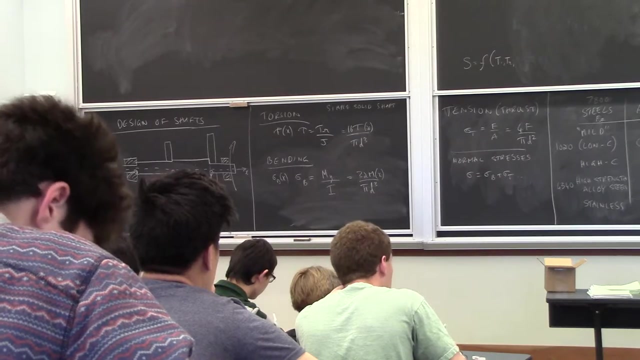 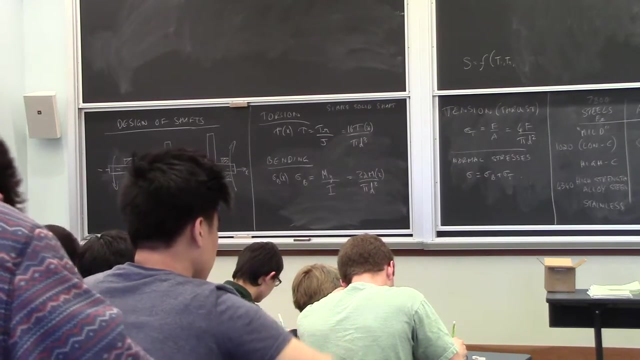 Which in this case would mean that square root of sigma over 2 squared plus tau squared, Where sigma is the sum of these normal stresses, Or if I do one-needles. I can calculate it that way. If I'm doing one-needles, I'll be looking at sigma equals e. 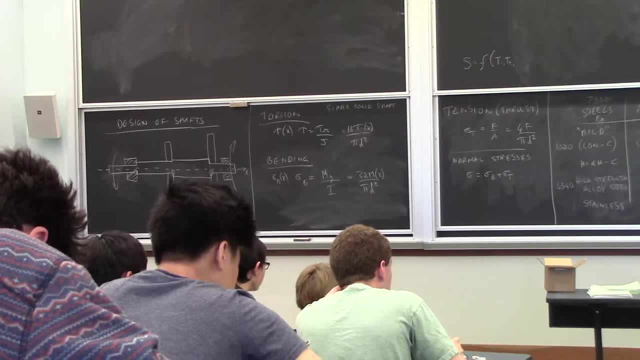 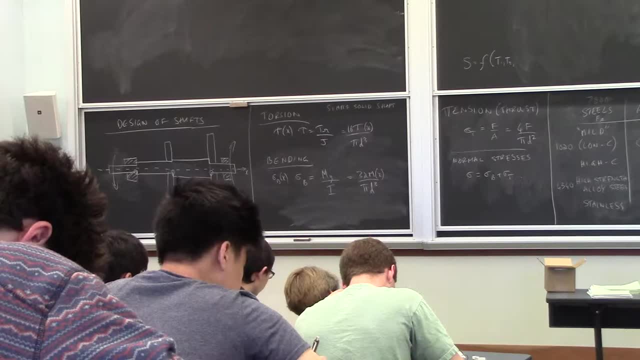 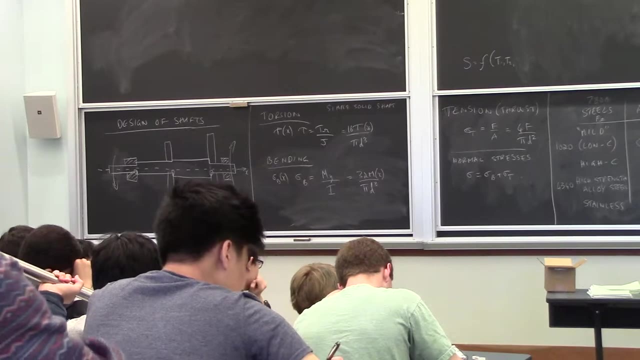 And I'm sending tau equal to sy over 2.. I can choose either one of these. It's my design choice. This one is more conservative than that, So let's just walk this through for a second. What am I actually doing when I design a shaft? 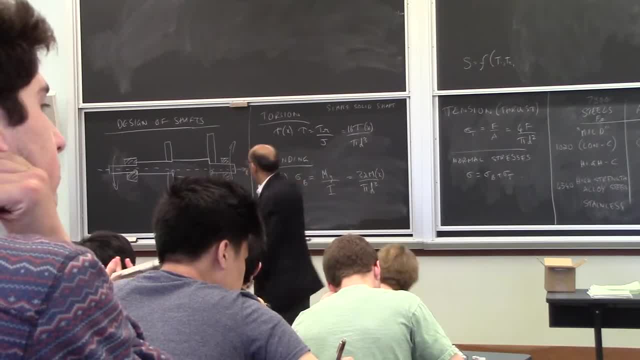 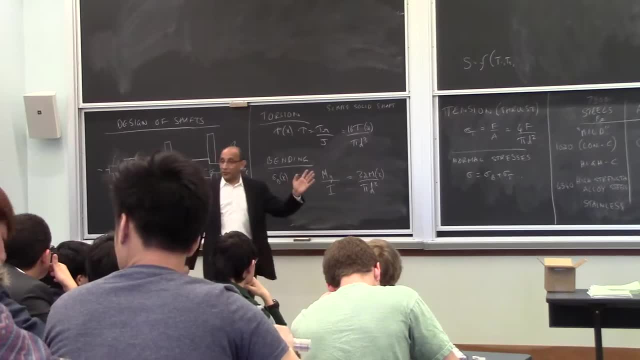 Because you can see, designing a shaft is analyzing a shaft. If you give me this, If you give me all the diameters, then all I have to do is calculate what the stresses are. Then that's exactly what I've done here Up to this point: I've calculated all the stresses. 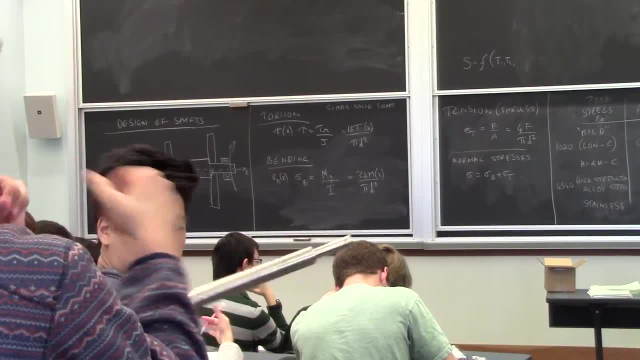 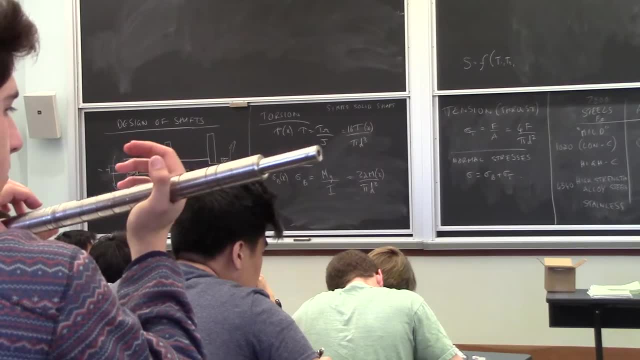 And done. I know where the stresses are going to be maximum And I can decide whether it will fail or not. Designing a shaft is. I want to calculate what the diameters should be. I know what torque I want to apply. I know what bending moments we're going to get. 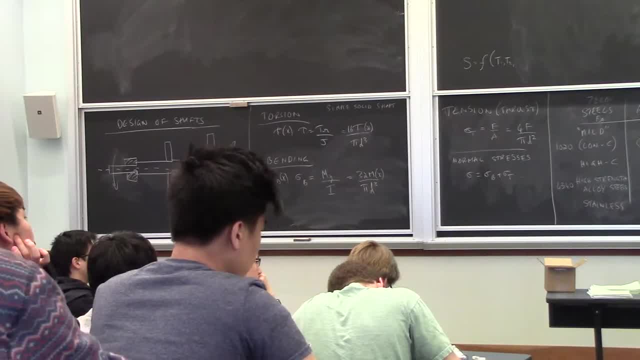 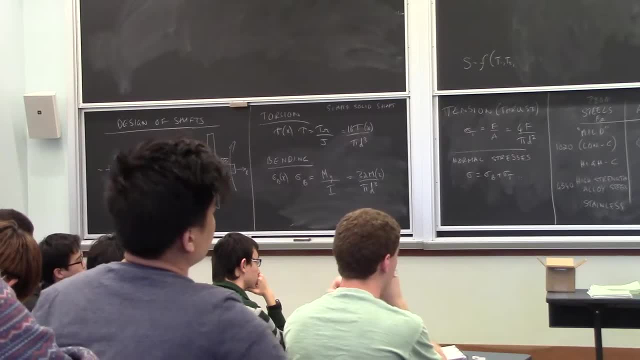 I want to calculate. I want to calculate what the shaft diameter should be. So in that case, what I'm doing is saying I'll give you sy. So you tell me at 17 post, stainless steel, I know sy. I choose the diameter of safety. 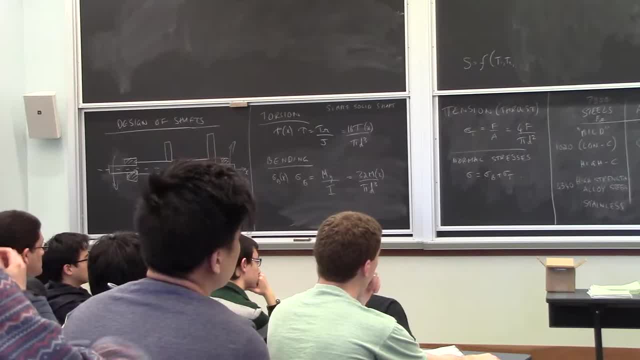 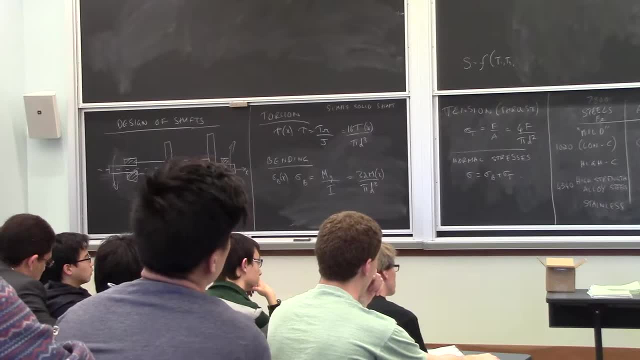 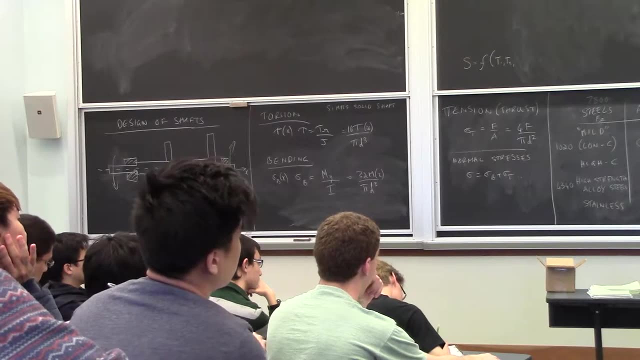 So I know the size. I want to solve this equation now for d, The diameter of the shaft. I will solve it at where I see the critical point, Where I think the torque and bending moment is going to be the maximum. So I look for where will this be maximum? 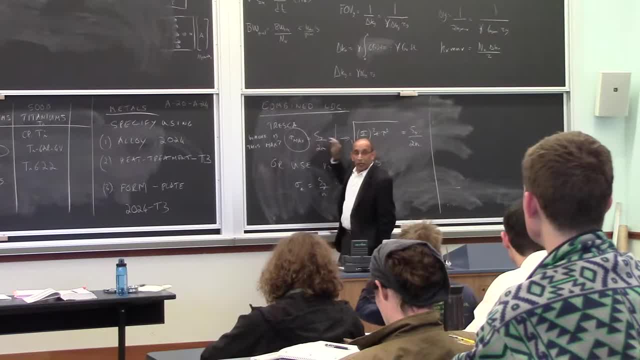 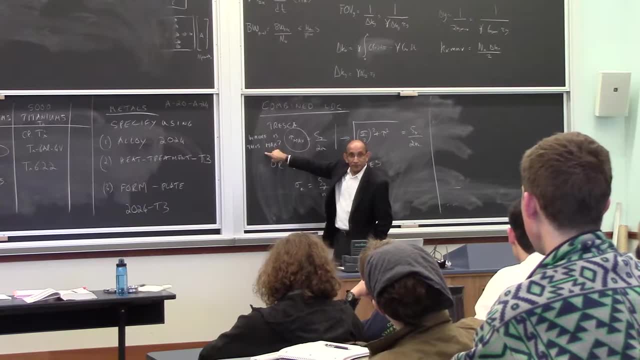 Remember, term max is just half sigma 1 minus sigma 3.. So every position term max is different. I look along the length of the shaft to decide where will this be the highest. I calculate the diameter of the shaft there by simply plugging these things in. 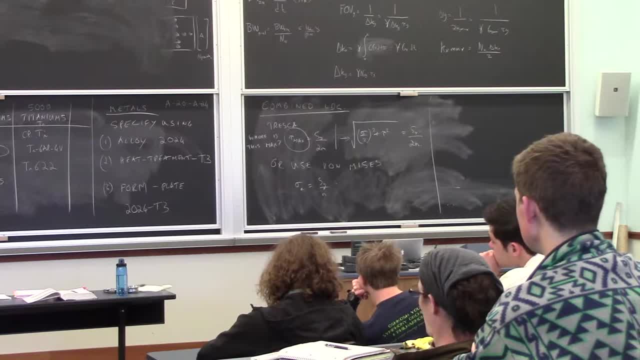 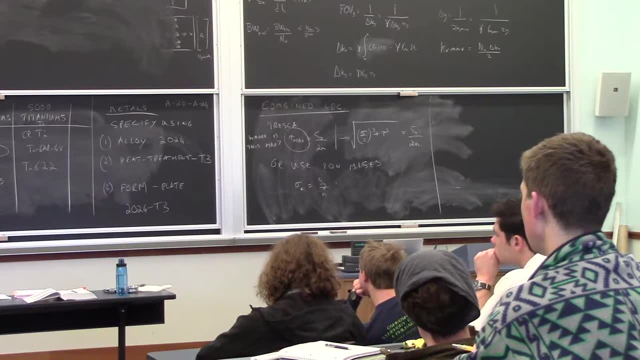 So let's assume that there's no truss node. If I just have these two, Then my d is going to go as tau to the 1 third. The d here goes as sigma to the 1 third, But sigma and tau are in here. 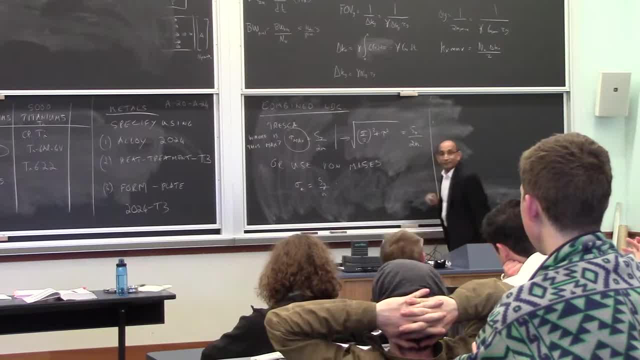 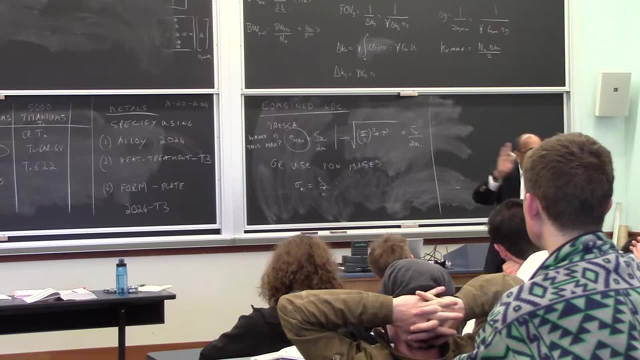 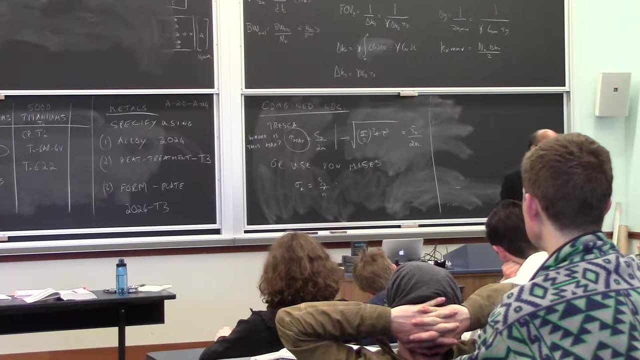 And so I'll plug those in here and solve this. Once I know d in the most dangerous place, Then I work backwards from there to all the other places And I design the nucleus for each of those shafts. So that's the design. 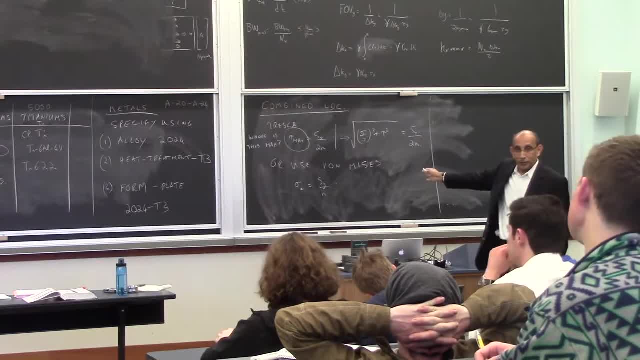 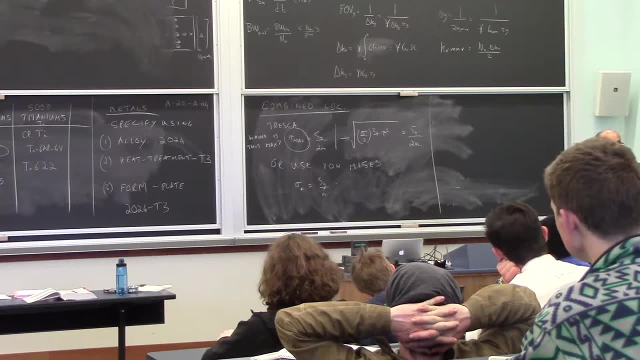 The analysis problem is: you give me the diameter. I can't give you that, But you are looking at the problem, The two paths. Either someone gives you the shaft and you're analyzing it Like you have here, Or the other path is someone gives you the loads. 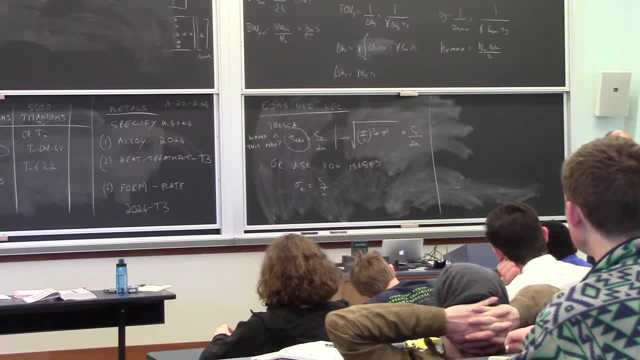 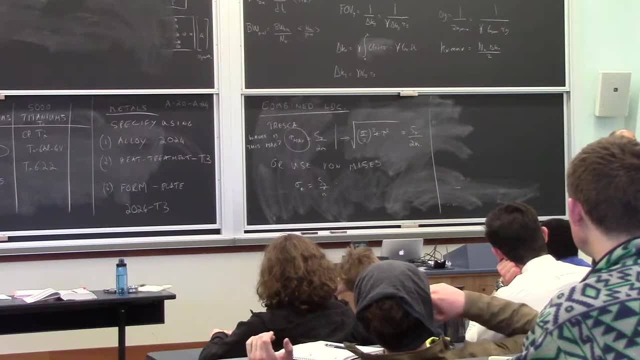 They tell you what torque you have to carry, Which is actually your design problem, And you don't give anything to me And you design the shaft And you design the diameter. So the design problem we're getting today is to design the shaft in the wind tunnel. 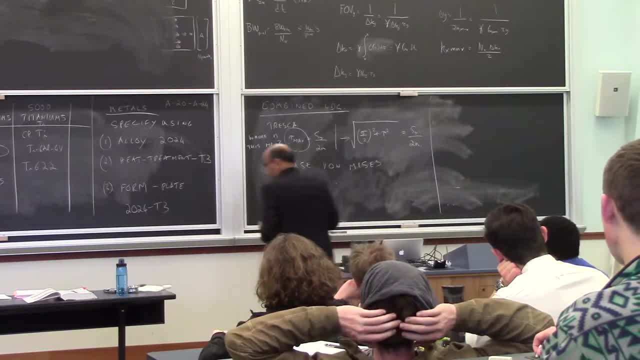 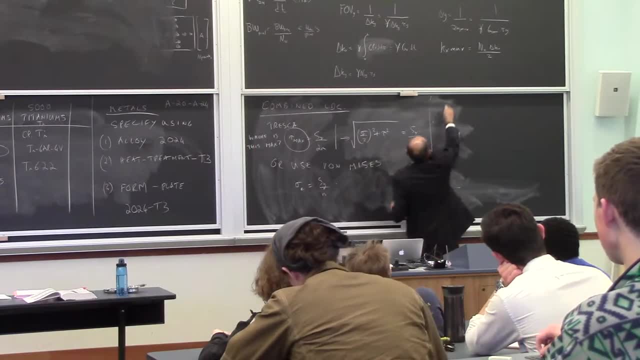 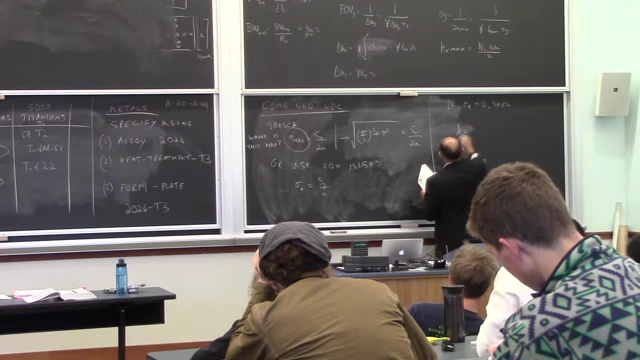 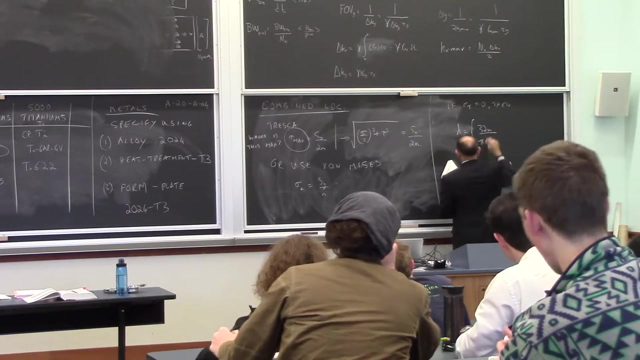 That would be part of the wind. That's in the beginning of the problem. If sigma t is equal to zero, Then you get them very quick. As a result of the analysis, V will be 32 and or pi, f, y, Or it will be m squared plus. 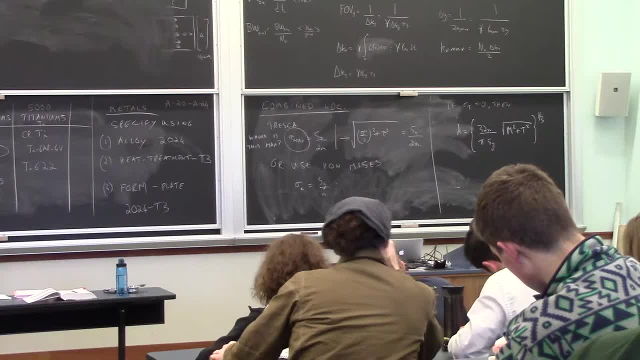 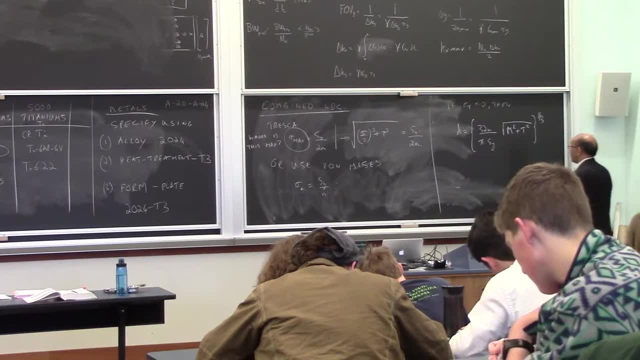 So if you know m and t The moment at the top, You didn't have to give me. So when you're designing a shaft, You end up with this thing. that Well, okay, I could choose s? y first And then i v. 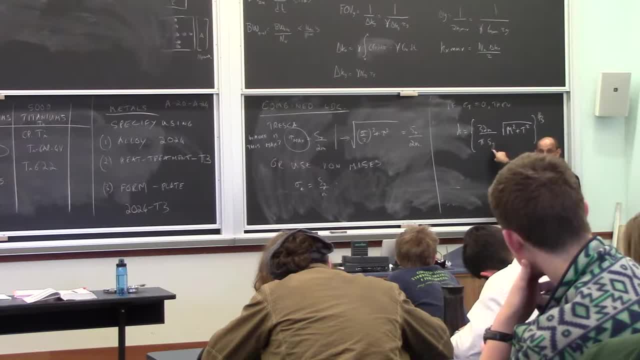 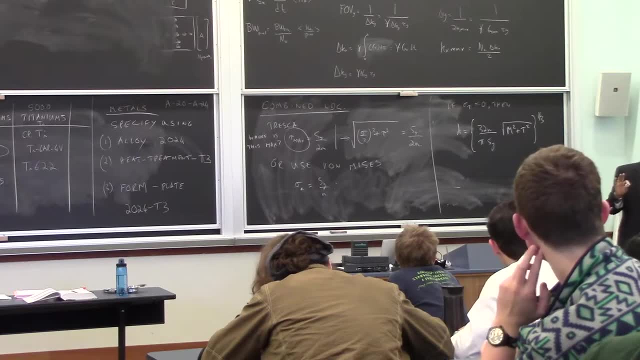 Or I could Say: this is the d I want And that's my s? y, And you can decide what the t you want. You can go either way. Typically, When we're doing these designs, It's good to Start by making a material choice. 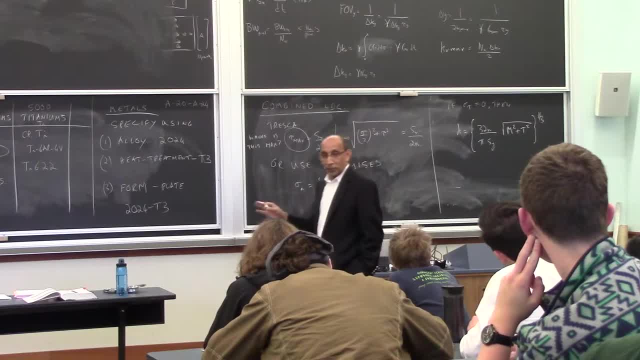 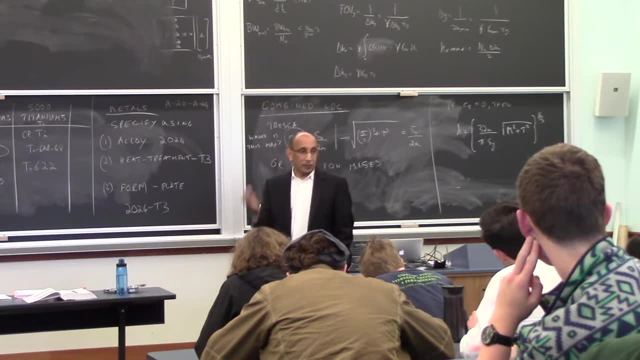 Do something cheap, Get an s? y at all, And then see if you can make this first with a cheap material, And if you can't, Then you go back and say: All right, Let's move on to a different, Increase mass. 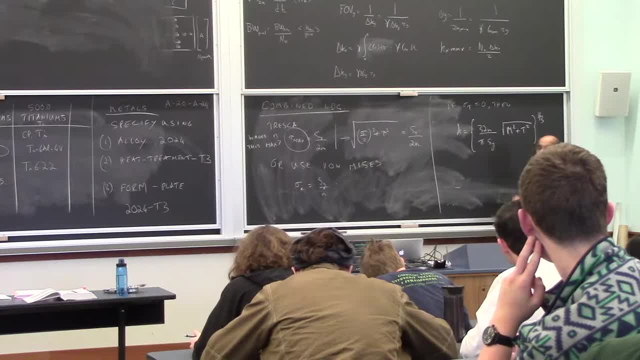 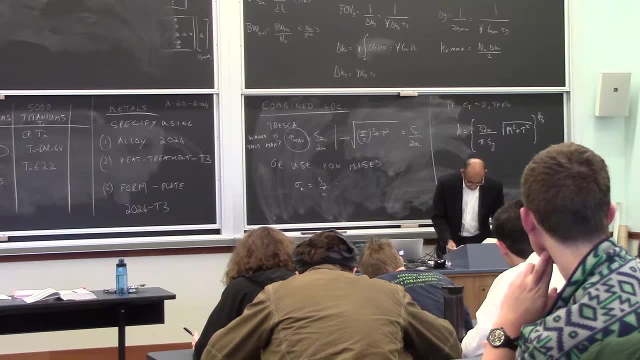 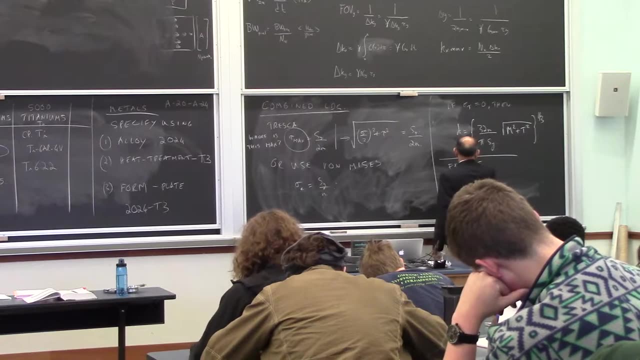 If sigma t is not equal to zero, Well, you just have to do this In the calculator Or in my lab Or somewhere. It's fairly simple. Oh, Let's talk about what happens in terms of the t. So the fact is: 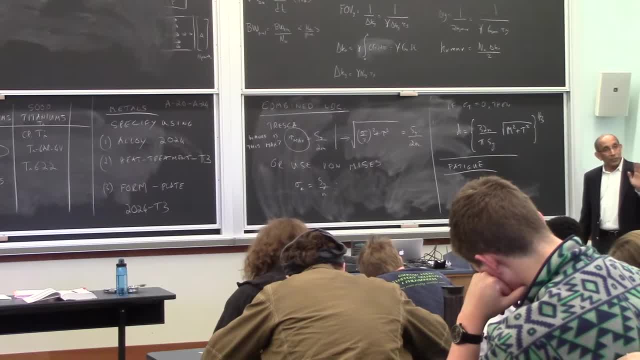 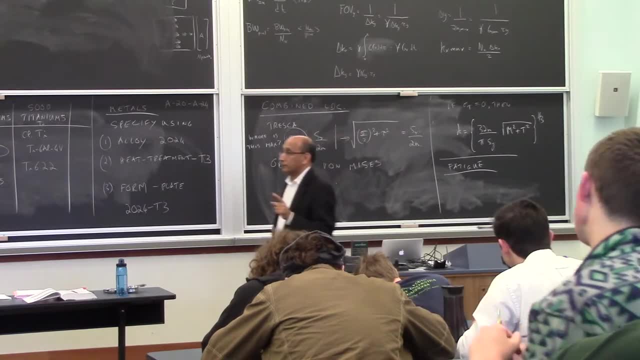 For any shaft in fatigue, The torque Is a steady load. The torque doesn't change Typically, But the bending moment Is a fully reversible Right. So Because the weight is always acting this way. So if you think about a given part of the shaft, 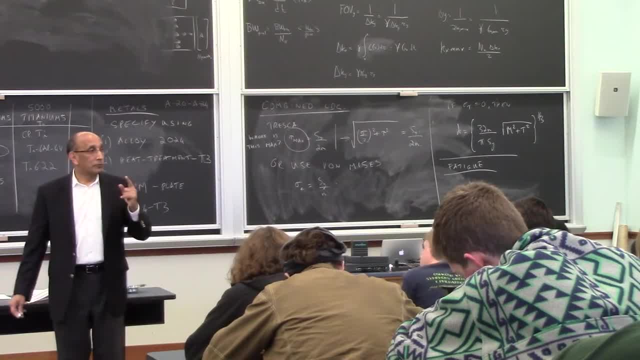 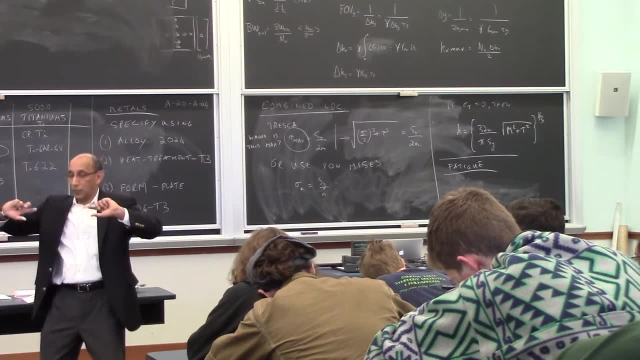 It was in tension And then, once it gets flipped over, Now it's in compression, So Your torque Is a fully reversible Right. So If you think about a given part of the shaft, It was in tension And then, once it gets flipped over, 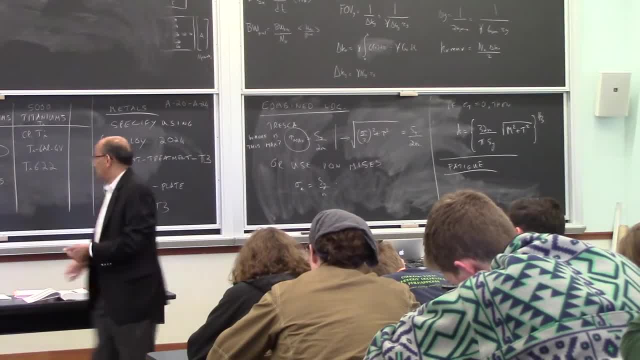 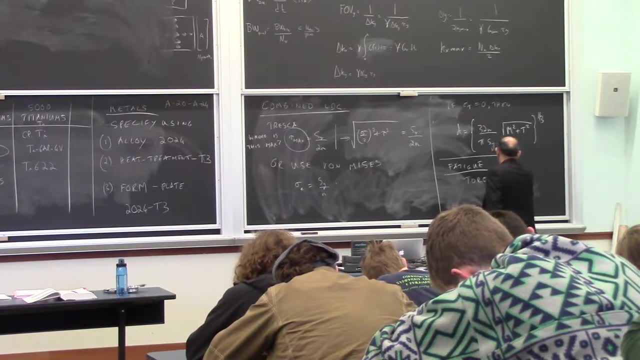 Now it's in compression, So Your torque Is a fully reversible Right, So Your torque Is steady And your Moment Is reversible. So this will give you Something like a sigma m. This will give you. 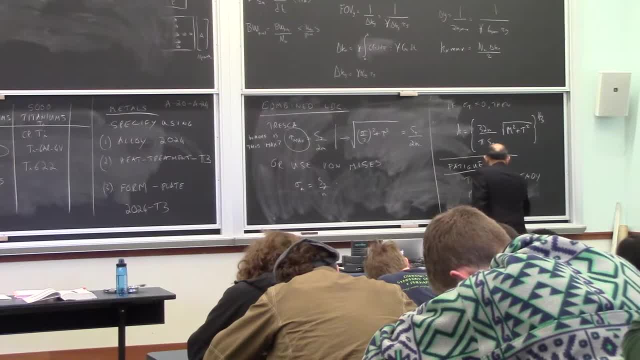 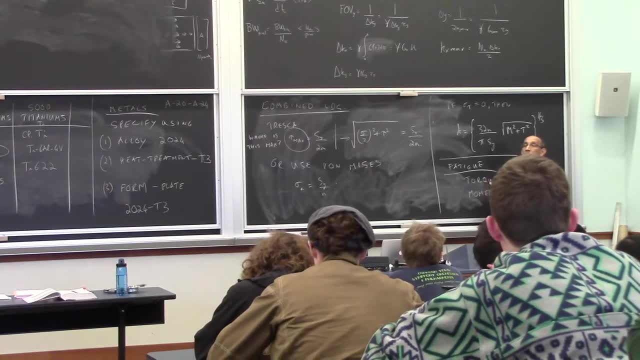 Something like a Amplitude Of the stress. And then you can use Your solid model Peripheral And your Curve of Peripheral And your Good Peripheral, Whichever one you want, And then You can Use. 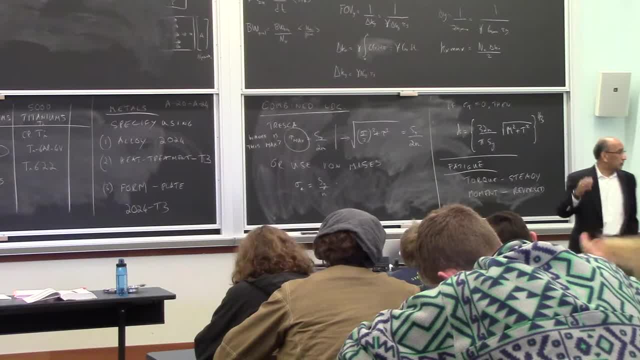 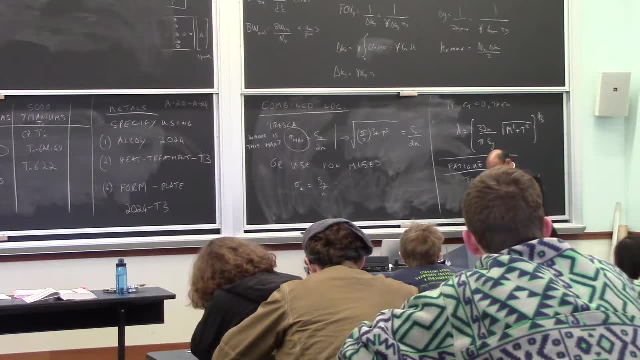 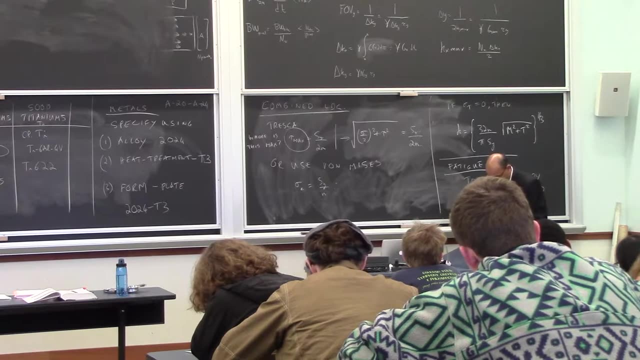 Your solid model Peripheral And your Curve of Peripheral And your Moment. So This is actually Very nicely done In your textbook. It is 360. On. I would Recommend You read Through. 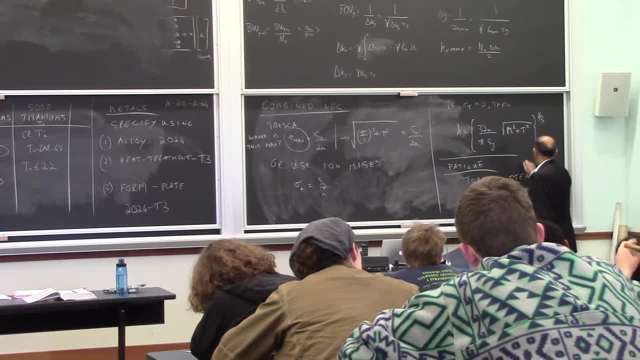 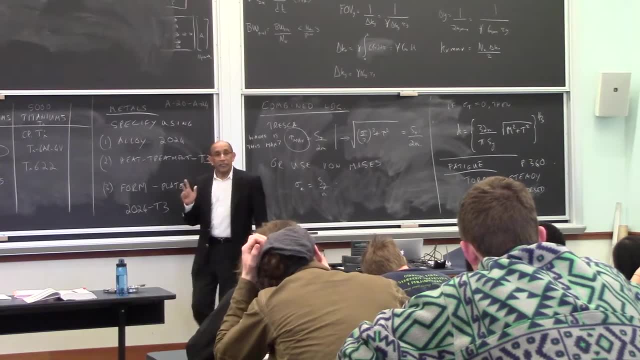 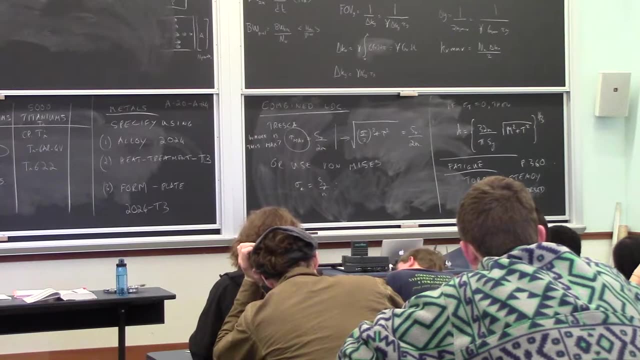 That section Because I know In fatigue It looks A little Messy And you get The End of All of these factors. A, A, K, D, K, C, K D I. 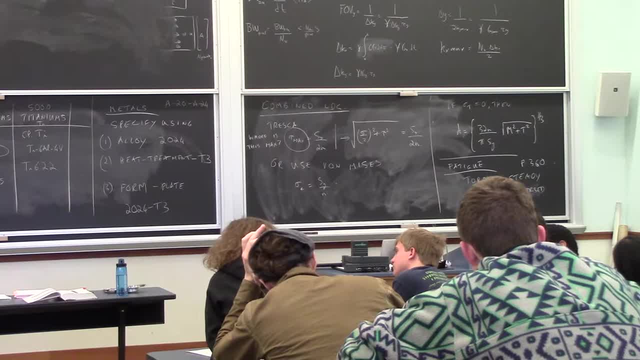 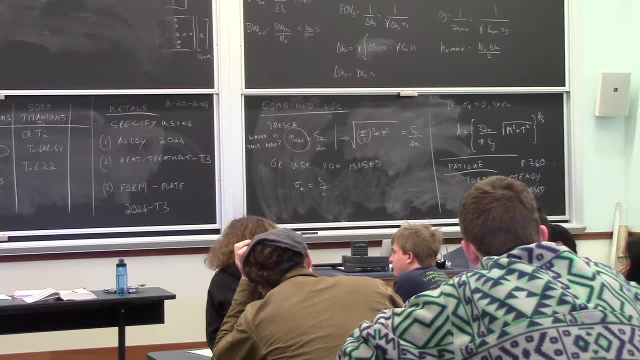 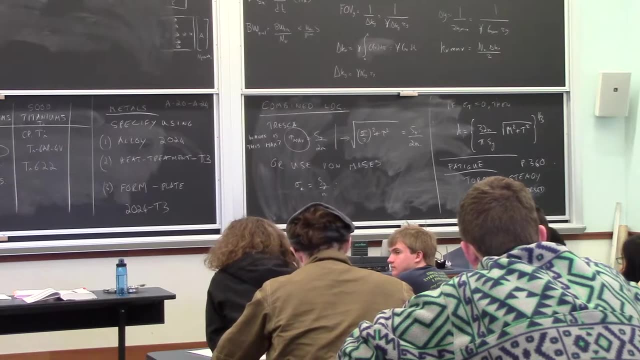 C Z I T V S x, Y, D, I, V, X V Y, N, X, X A, X A, X, X, X, V Y V. 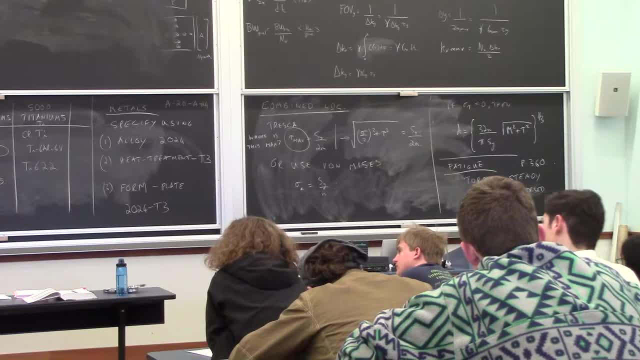 X, X, get more accurate and more careful for the analysis. but it costs quite a bit of time. Your time is fairly expensive. If you once you've been hired as an engineer by a company, your hourly rate is fairly high. And if it takes you three hours to solve something, 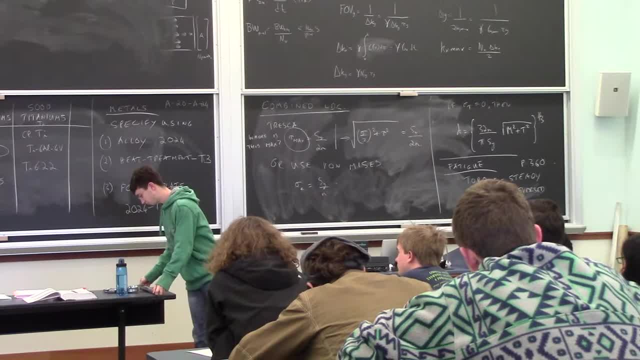 where you can look it up using this formula in ten seconds, you have cost that much more. So unless you're going to gain significantly from a people analysis, you don't necessarily do a people analysis. You pretty much have. There are a number of ways where you just have to make choices. 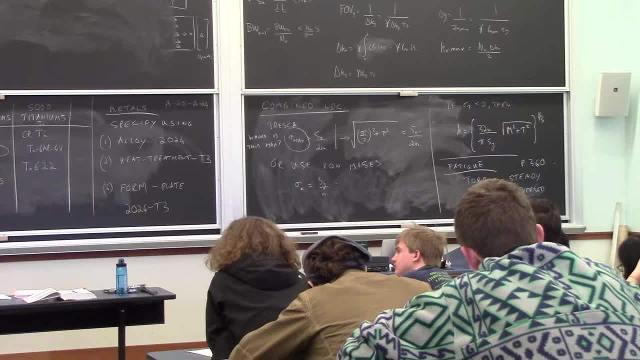 So usually if you go to a particular company, they will tell you: this is what we in our company for this application, this is what we said. Usually the way you get it is: you have a series of cases. 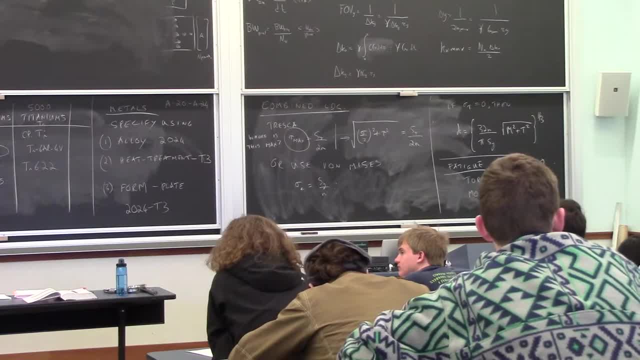 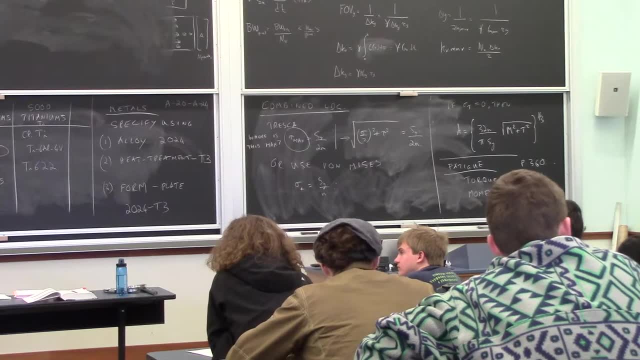 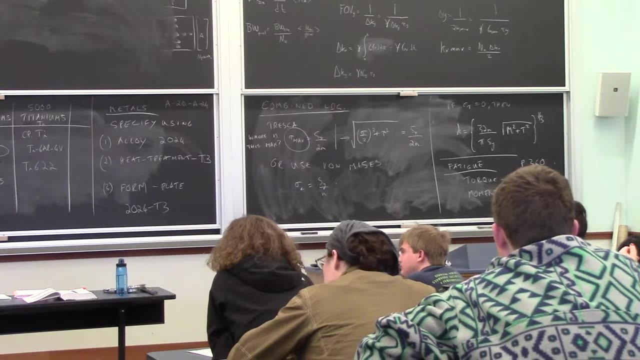 So in this case you can choose this value here, this case. here It's based on history. Usually it's based on data. So if you go to GM, for instance, actually the best example is GE, When GE does a chart design for all the Germans and so forth. they've built these things for 60,, 70 years. 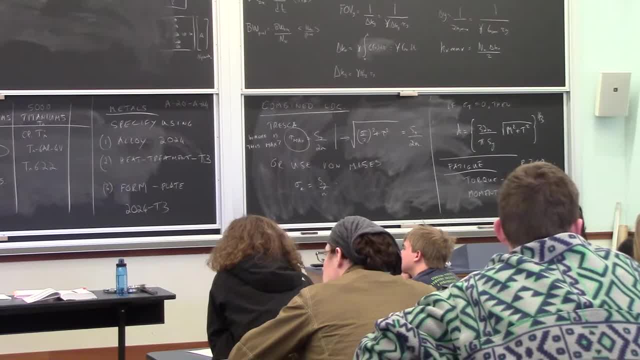 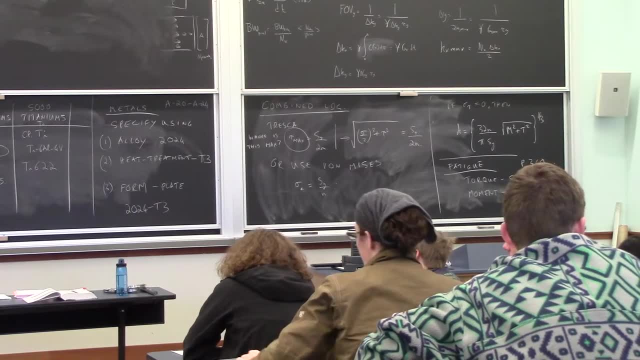 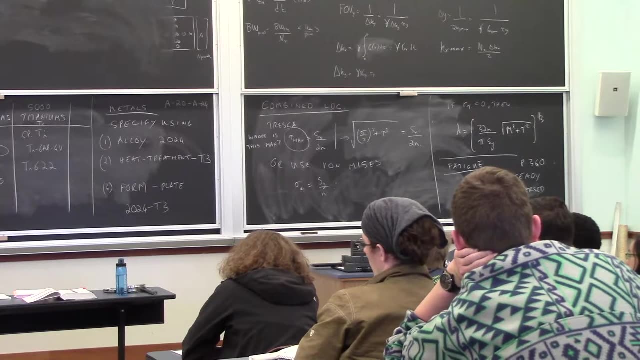 they've got this case for every single chart. they have used that data set And GE will not give those cases to anyone else. So GE protects that religiously. If you work for GE and then you go work for Bratton Whitney, you are bargained by contracting. 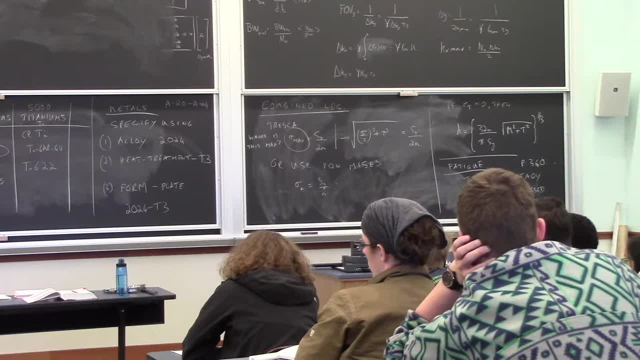 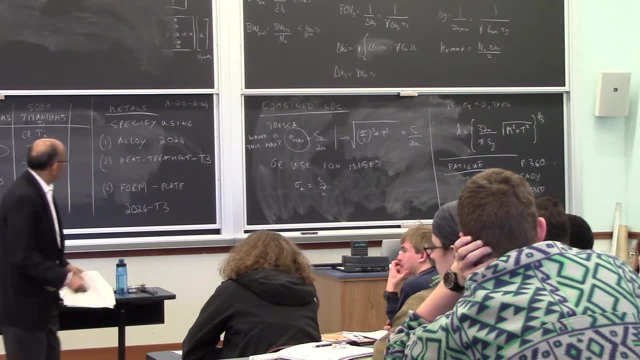 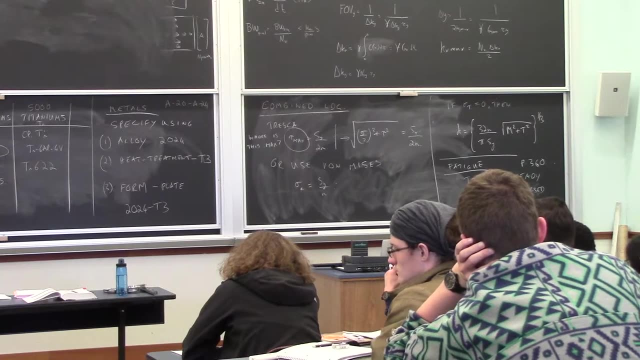 Actually, you cannot go work for Bratton Whitney for a certain time. There are some things you cannot go work in. All right, Now the book is pretty good about all of this. on chart design, There's one place where the book isn't as good as I'd like. 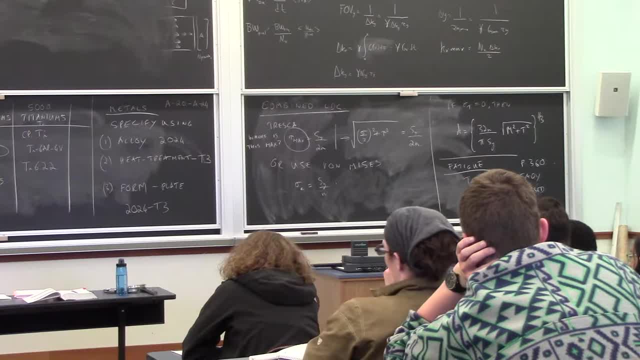 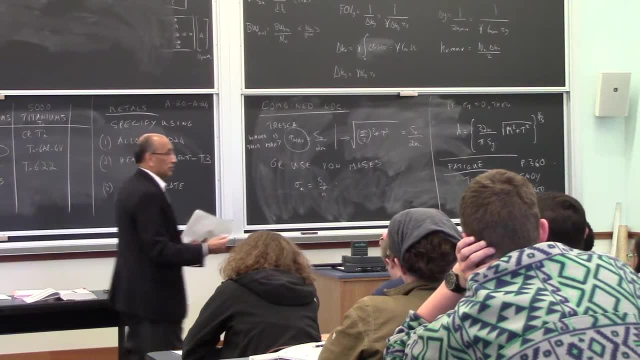 Let's talk about that for a minute. So all of this is sort of stress-based design. The reason that you don't have charters is because at completion, you simply don't put them on your chart. So you want to decide which ones project the llamas. 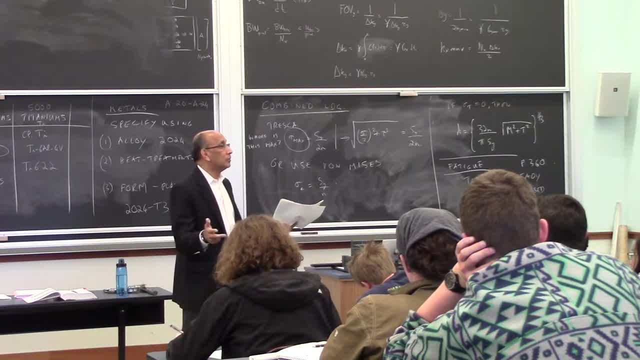 and how makes your chart to carry a certainはい. Well, suppose in one reflection phase. So you want to decide how must the chart would deflect under the moon? I have not taught you how to do deflection analysis in WA, España. 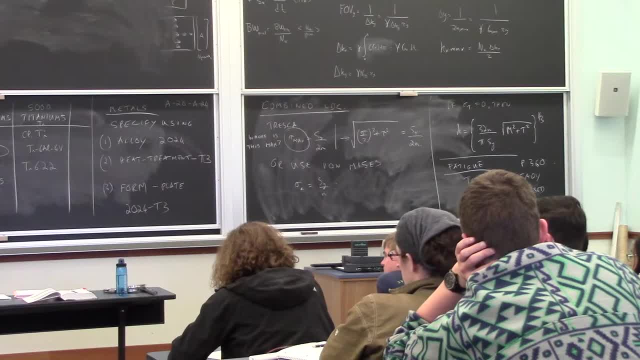 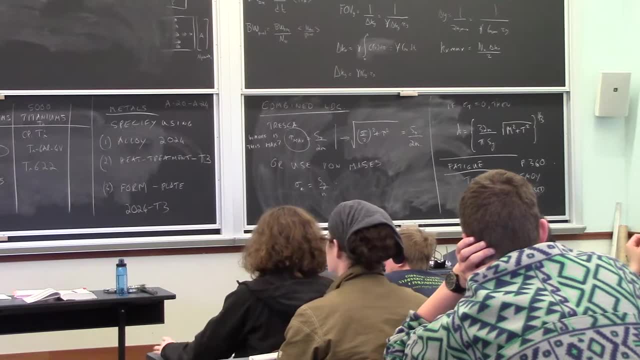 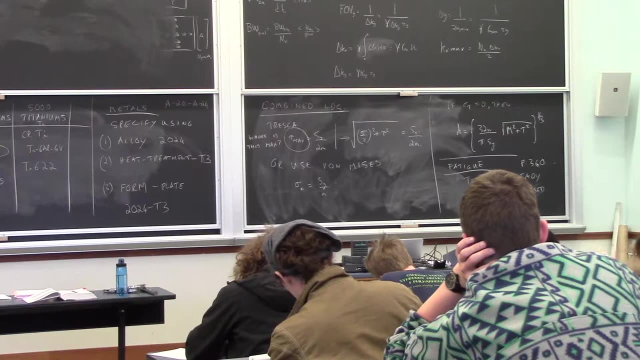 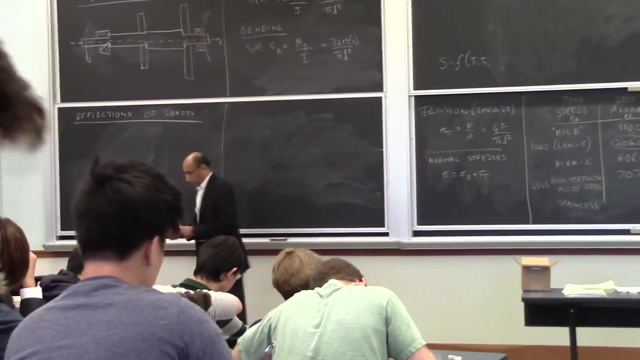 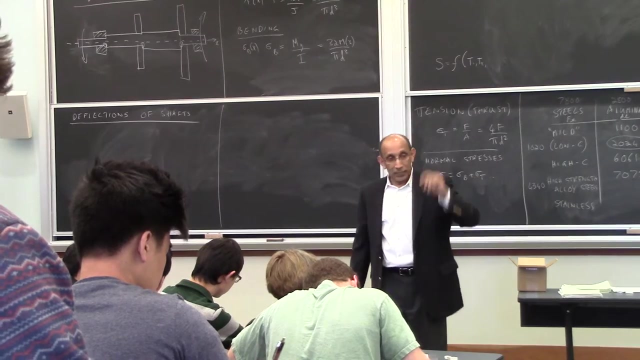 I wouldn't think you could put that in the selection mechanics, although you may have thought about it. So I'm going to give you a quick break. So the correct way to do stiffness analysis of shafts is to do a calculation like: 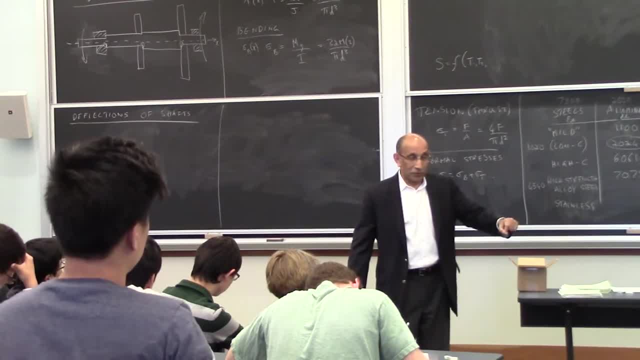 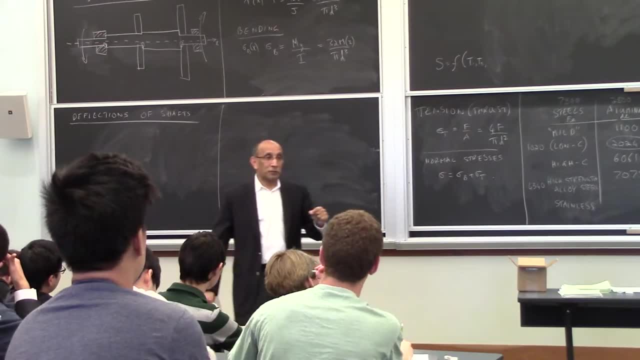 this: First you do the torsion calculations, calculate these deflections. you do that. Then you do the bending calculations, calculate the deflections. you do that and you add water, And for each of those deflections you will have to worry about what are the stress. 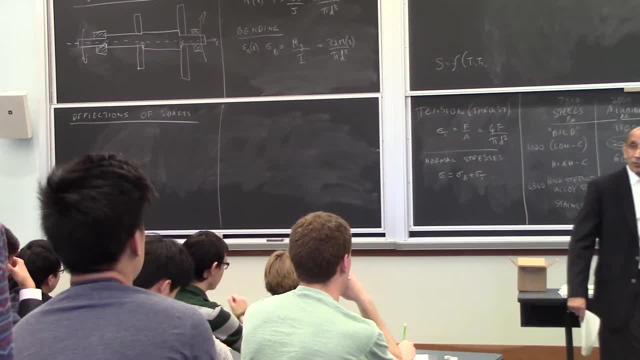 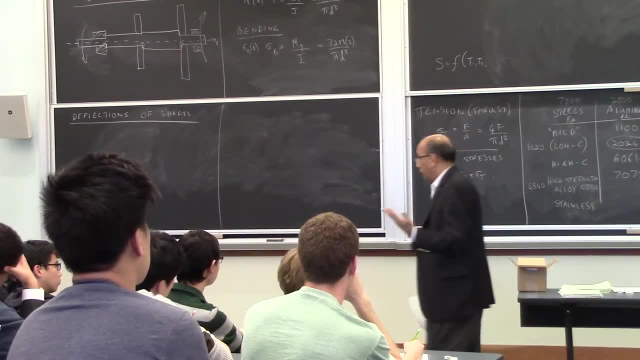 concentrations. what does that mean in terms of deflections? So usually you end up doing a computation of some sort, maybe a final element of that. That's the way one traditionally does it. However, that's too complicated for this class. That's going to give you a heuristic. 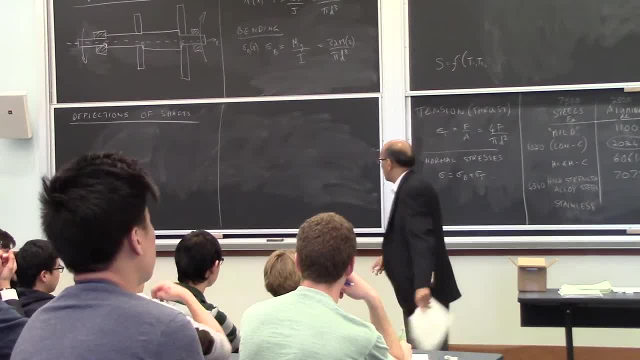 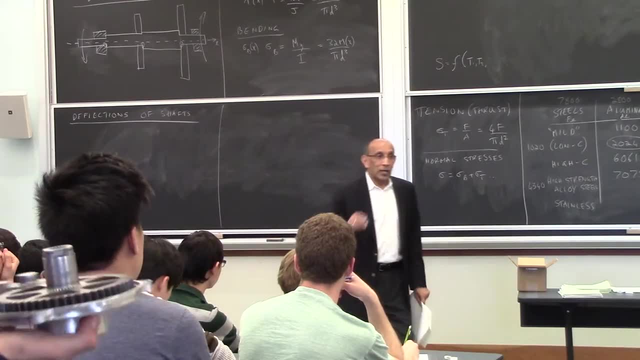 way of doing it. That's based on what you've done. A lot of people have done for many years before they had man-at-arms because they said they didn't have access to something. So what they did was they said: I'm not really. 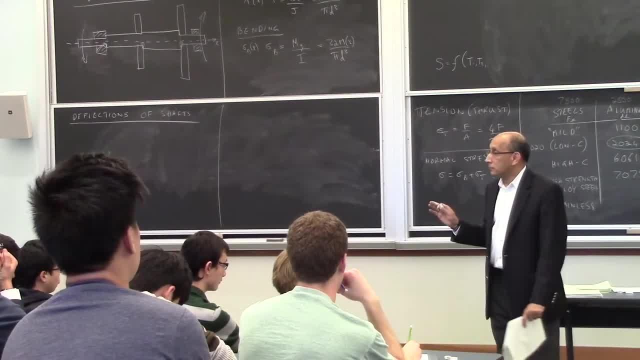 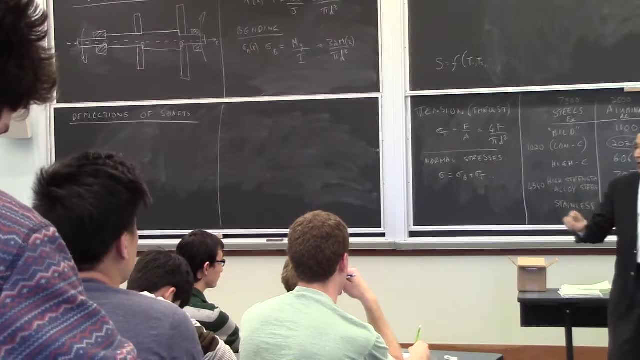 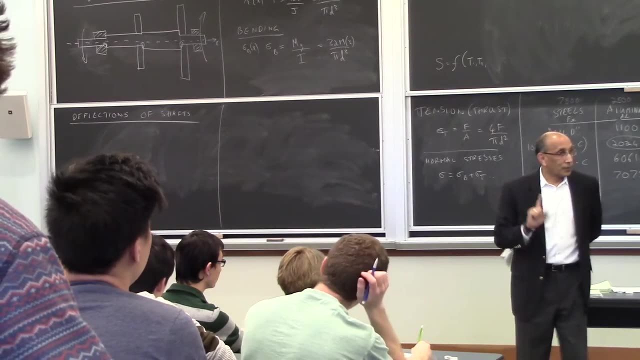 going to worry about designing a shaft so it doesn't deflect. I'm not going to try to design to fix deflections. Instead, what I will do is I will calculate how far apart the bearings have to be to limit my deflection. So let's think this through for a minute. 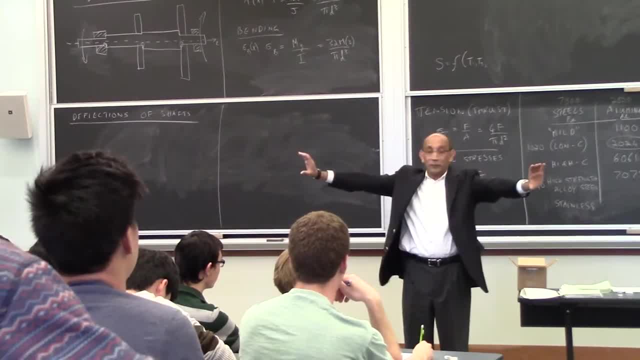 In principle. if I took my shaft right, here's the deflection. This is a long shaft. If I put just two bearings on it in the middle of the shaft, it could hang down a bit. That would make a deflection. That's better. 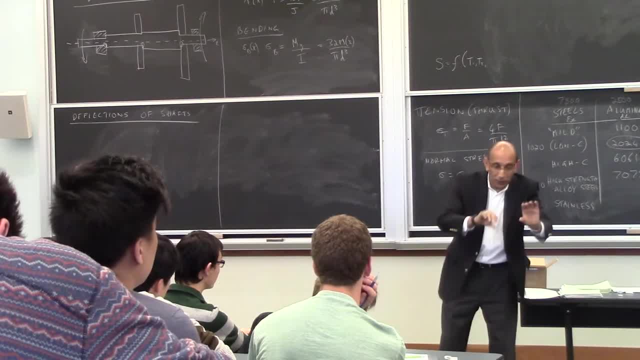 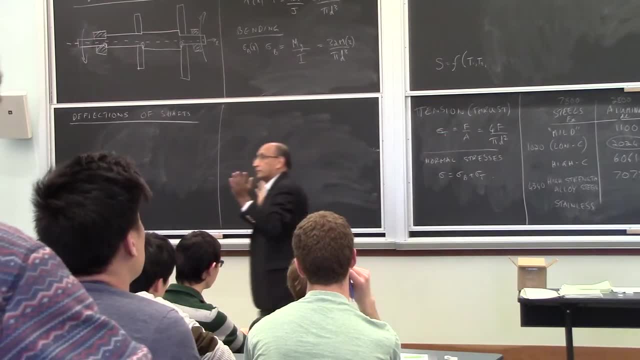 Then if I put another bearing in the middle now, this part will hang down a bit, this part will hang down a bit. That can make a deflection. So in principle, if I put enough bearings on it, my deflection is going to be zero. Because if I put enough bearings on it I 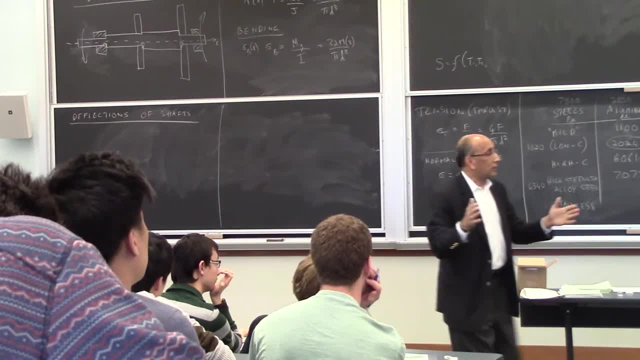 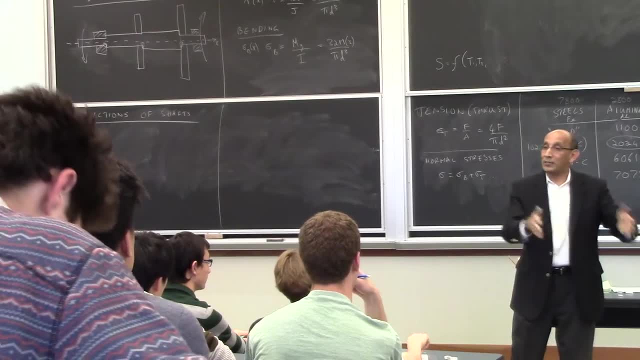 don't have a shaft. So the question is: what is the distance between bearings that you are willing to accept? And you determine that by saying what is the deflection distance I'm willing to accept between bearings. So this is a quick way of doing shaft design. 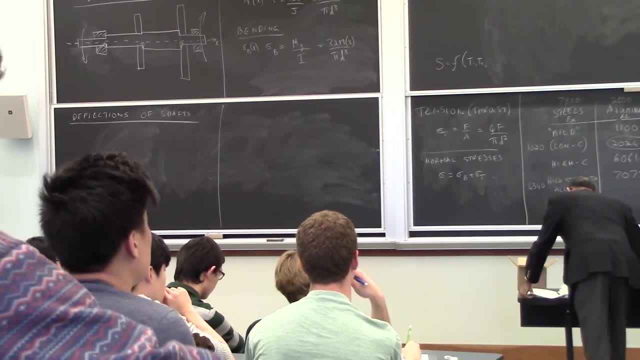 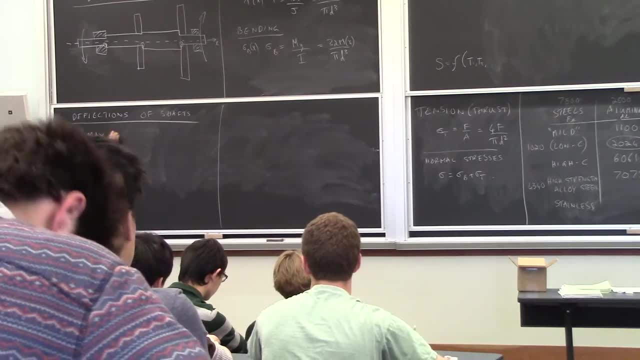 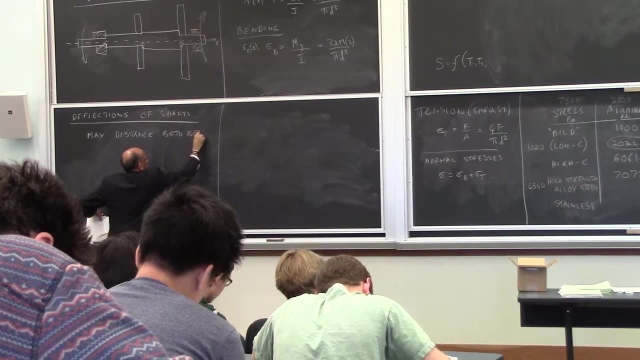 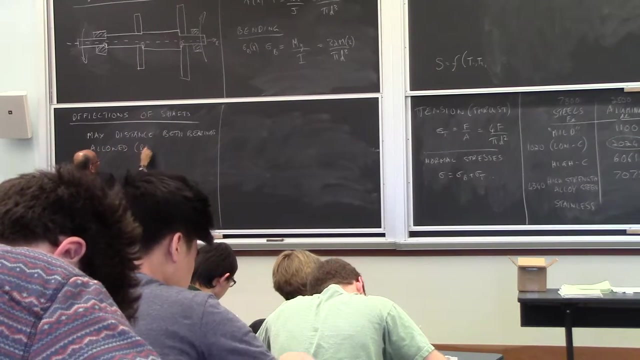 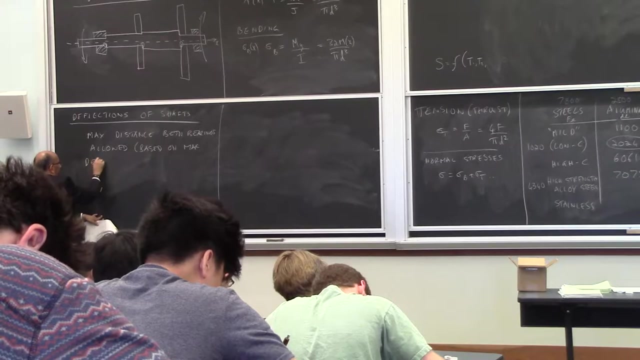 Just decide what deflection is that you're going to accept. So here are the distances between bearings that typically one finds. So let's look at the maximum distance between bearings And if you're going to allow- By the way, this is based on the idea that you have a maximum deflection of 0.8 millimeters- 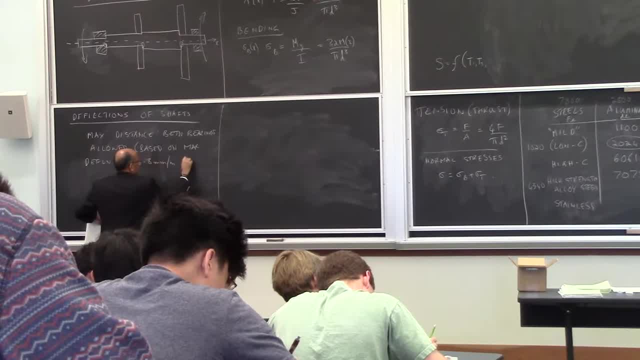 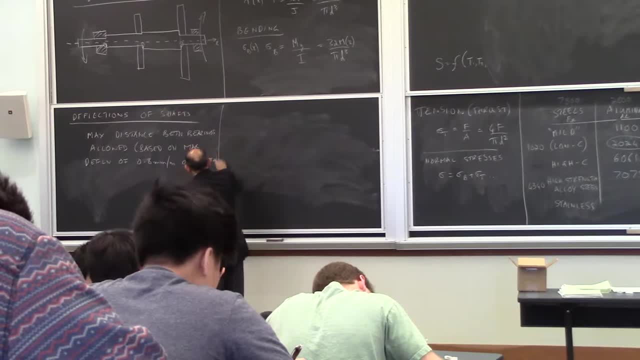 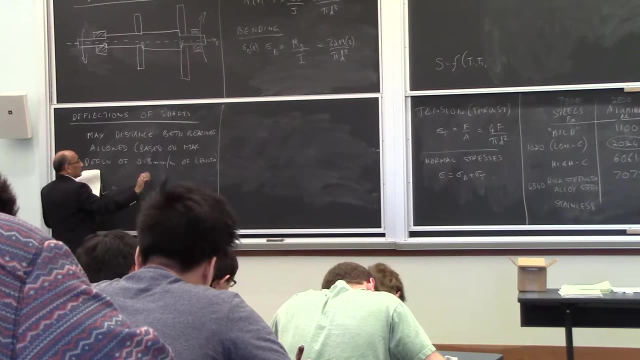 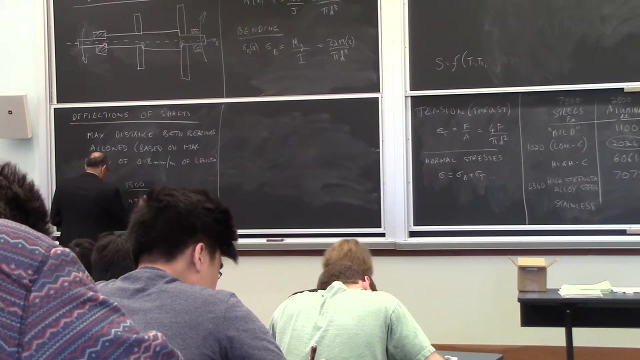 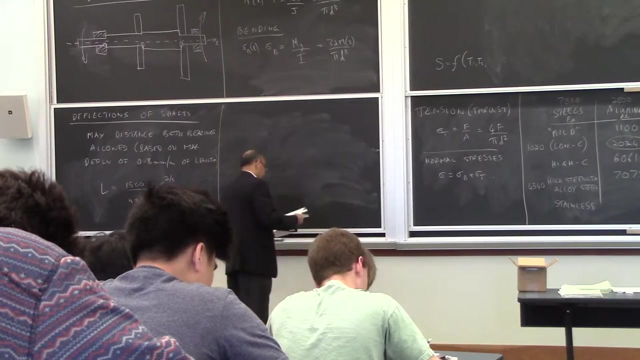 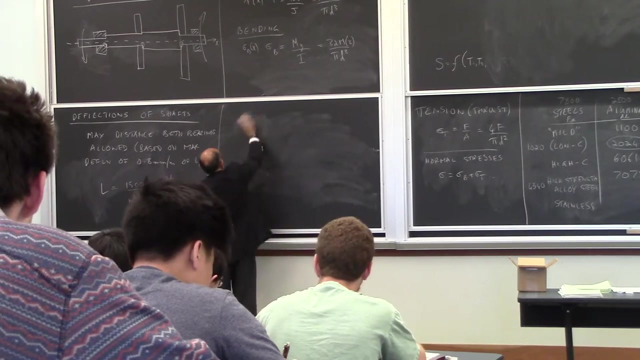 per meter of shaft. If you assume that's what you're willing to accept, then here's the equation And everything here is in terms of meters. So this is the SI units, But these are the critical diameter And you'll see. 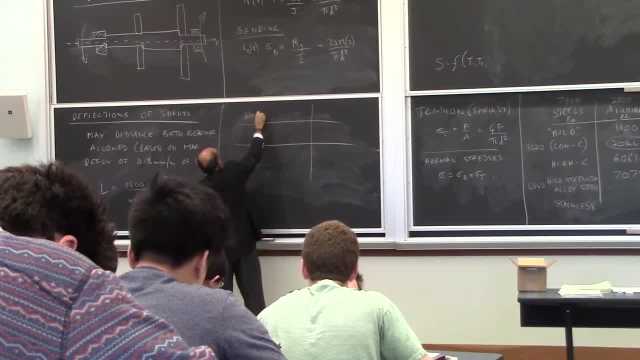 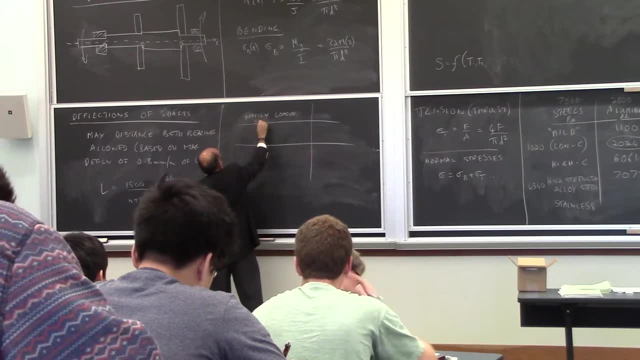 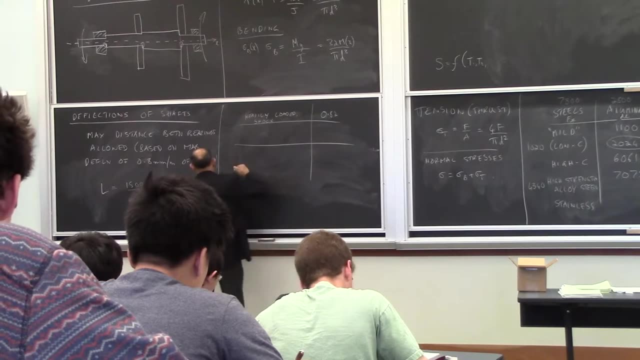 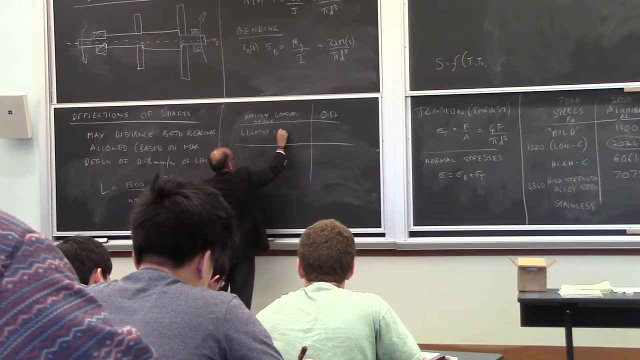 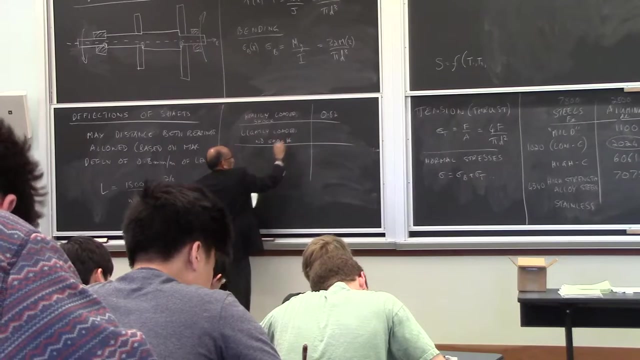 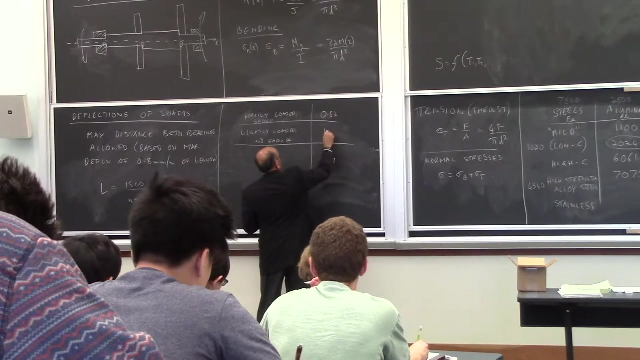 So if I have a heavily loaded shaft, with shock when I make C 0.8, if it's lightly loaded, no shock. so the idea of shock is that something falls in it And you make C 1.1.. 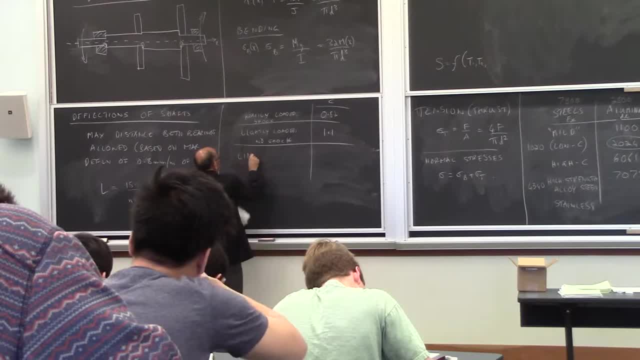 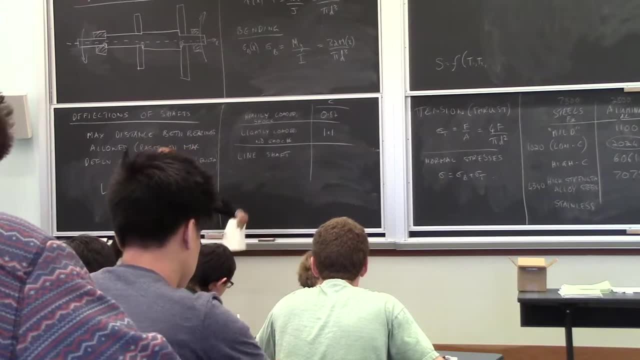 And if you have what's called a Ryan shaft, it's very lightly loaded. So this might be the kind of thing you would have seen in the old movies that people had where they had machine shops, where you had one shaft running up a roof. 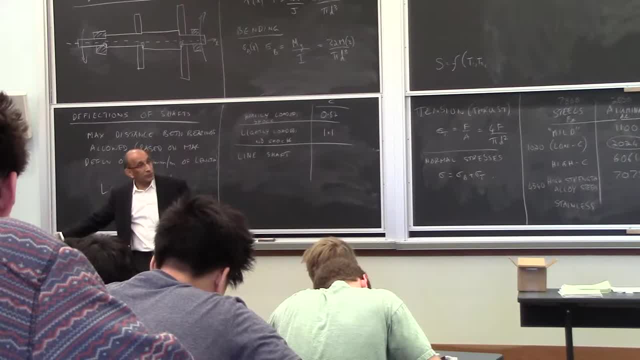 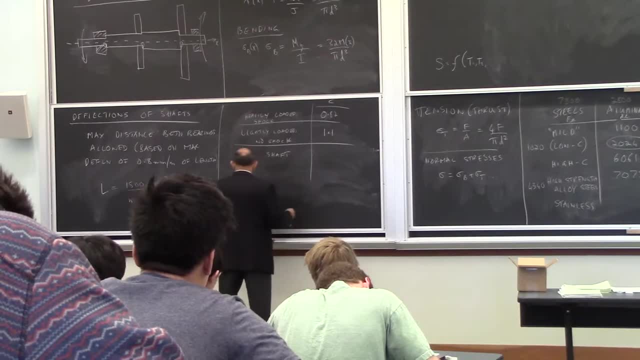 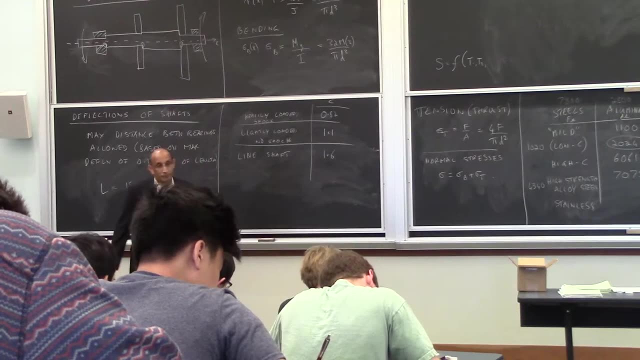 a whole bunch of coonies and then dunce coming down through the two machines. Those are called Ryan shafts. You can see those in the Smithsonian Tower. You might have visually understood what they were. For this case you would end up with a C of like 1.5 or 0.6.. 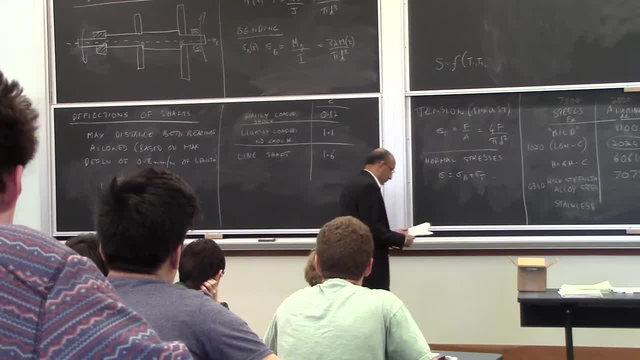 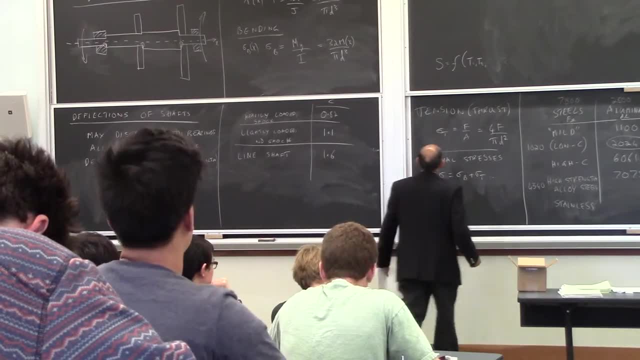 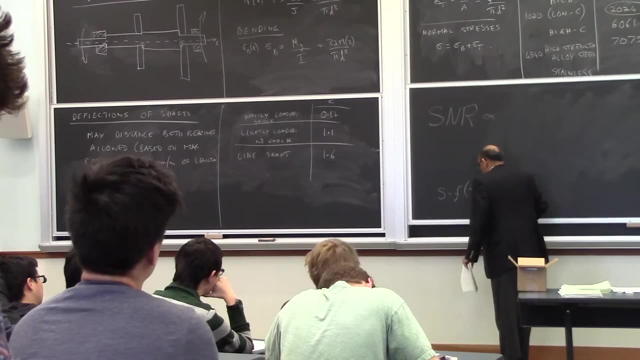 This gives you a rough way of calculating the D of that. And here's a different D. there It's the same last name, Okay. so with that in mind, I'm going to give you a summary of a process for design of shafts. 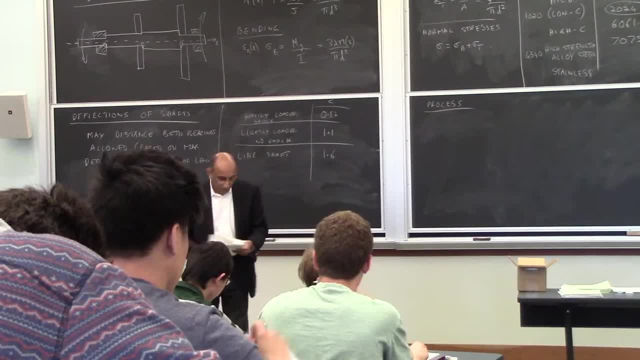 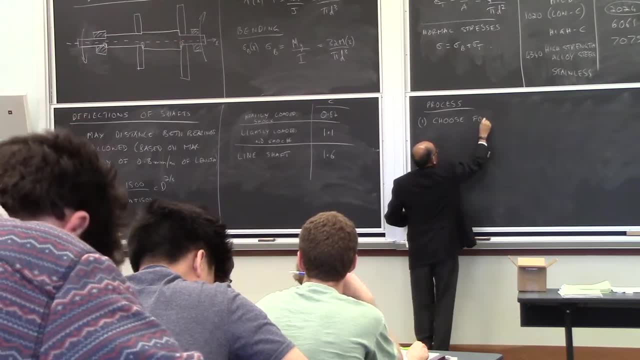 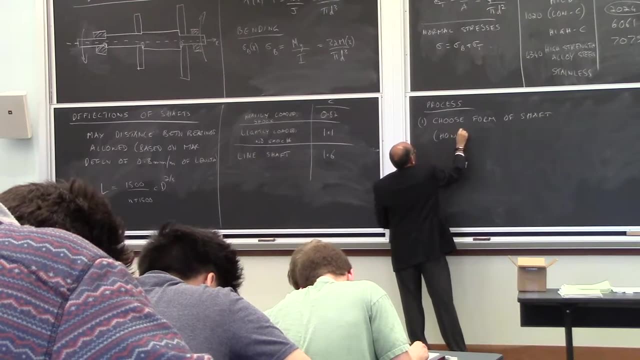 This is just one example. I don't know if people will agree with it. It's meaningless to me either way. So first you choose the form of the shaft. So this might be saying: how many steps do you need And how far apart do they have to be to use? 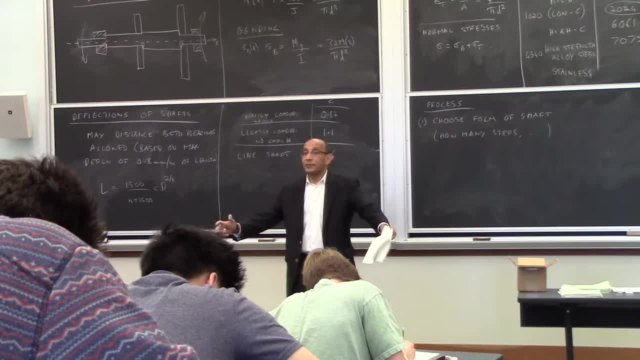 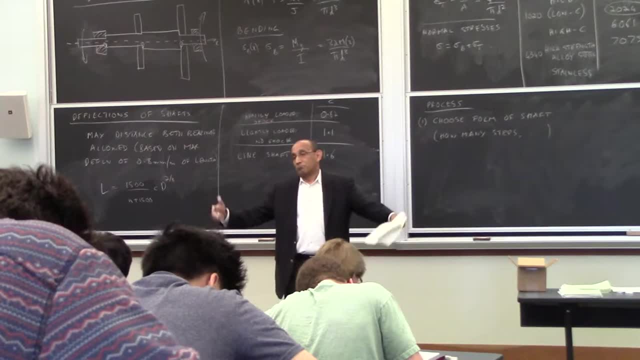 So this is basically the one that tells you I have only this much room to put the thing, So the shaft has to be about this long because I have only that much room in my machine And I can only have typically spacings of this order. 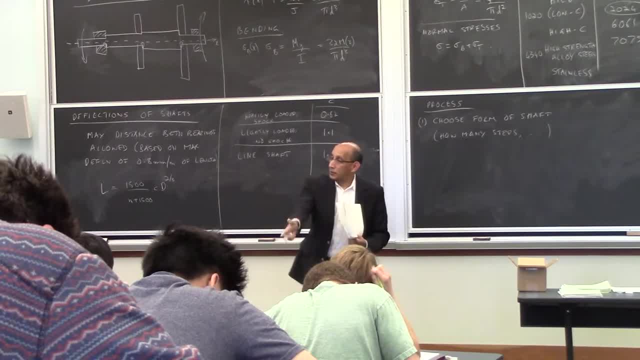 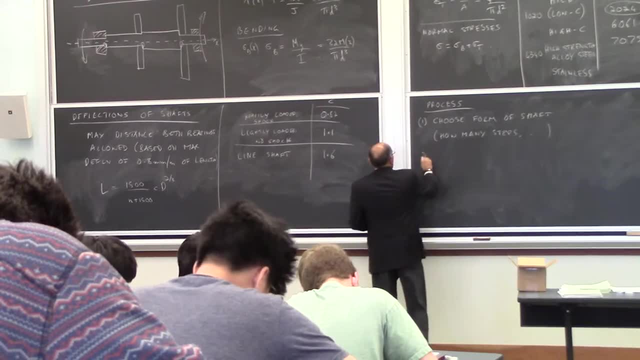 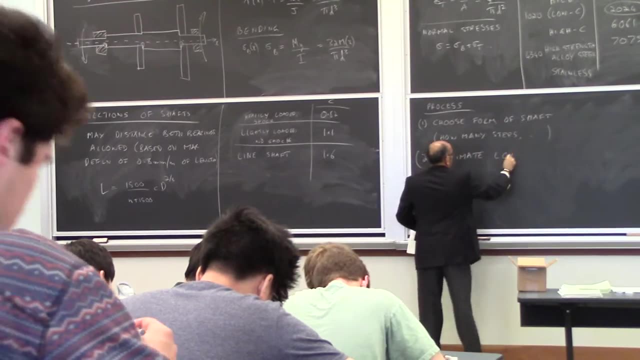 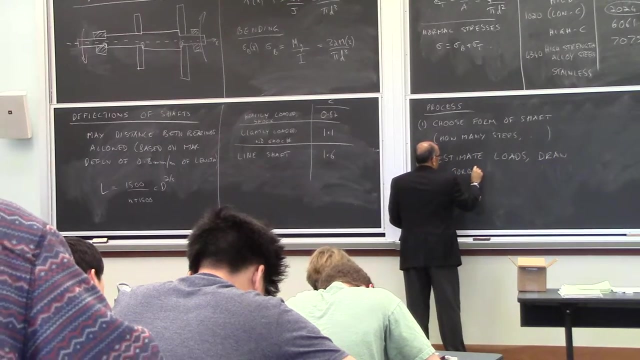 because my power source is here and it faces with the little part that's here, So I'm constrained by the rest of the system. Once you've got that, you estimate the loads And you draw the torque diagram, the bending moment diagram. 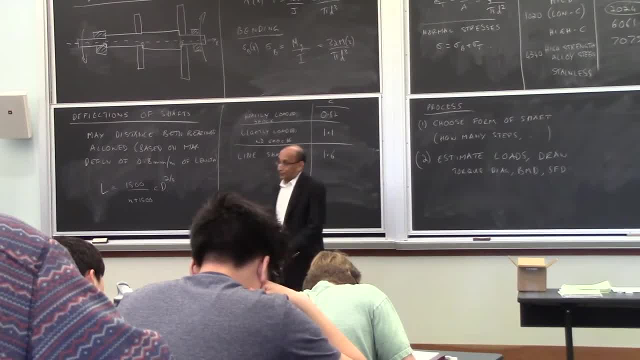 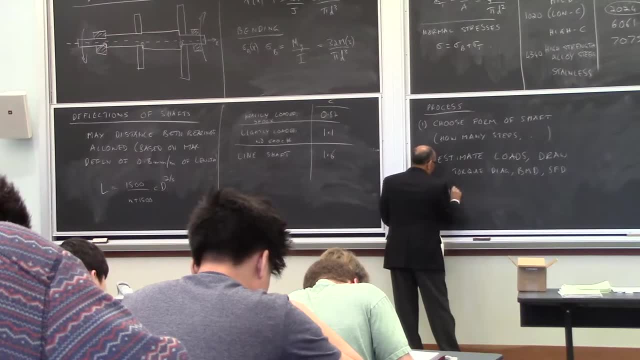 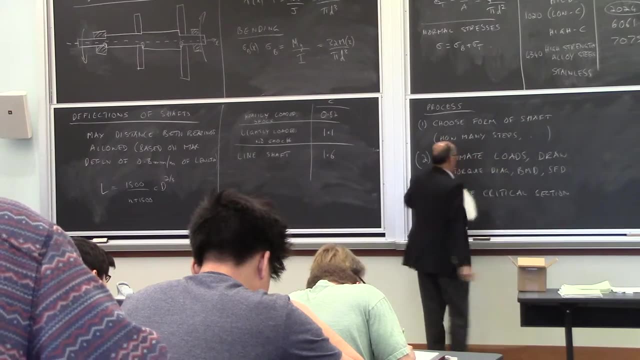 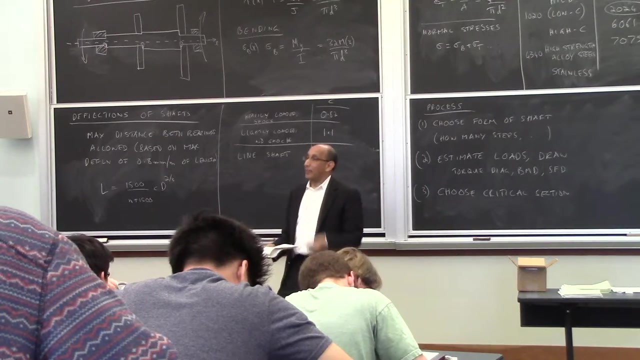 and the shear force diagram. Then you choose the critical section. Basically, once you've got those three, you calculate your stresses and you decide where it's likely to be critical. You know where the M is the highest and the C is the highest. 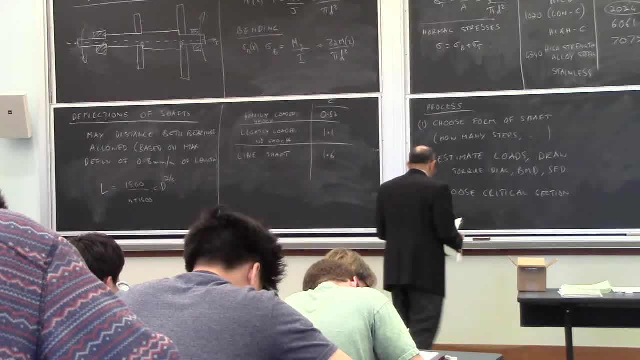 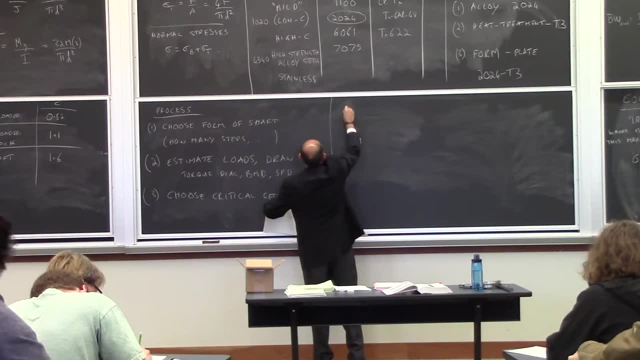 and where the signal's going to be the highest. So you're just using this to identify where things are likely to be bad. Sometimes you know you've got the science and you have two or three points and you say I'm going to calculate with those three points. 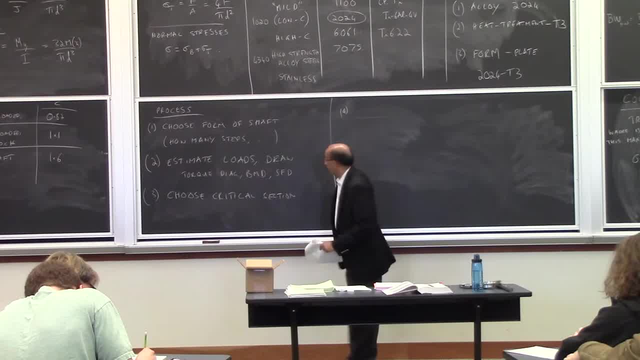 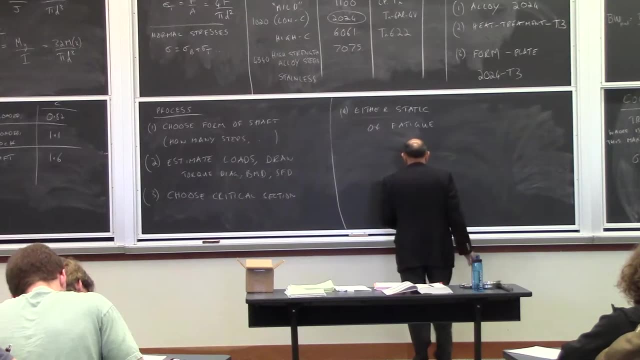 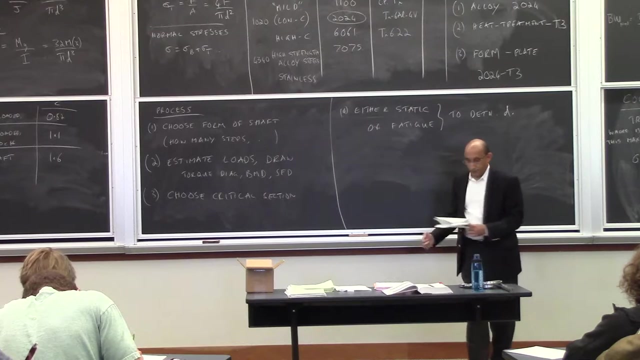 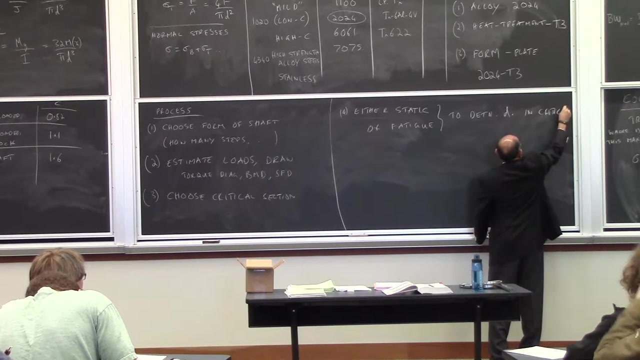 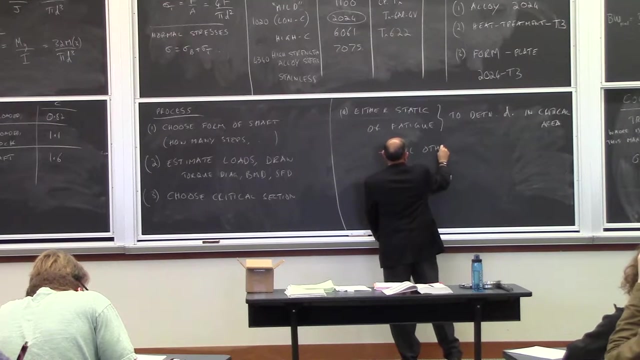 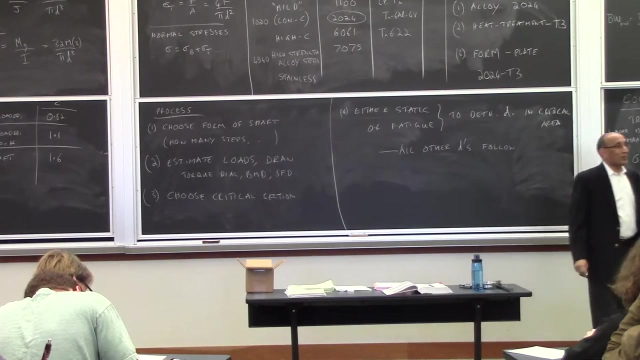 And after you've done the whole calculation, you say, well, this is bad. OK, Now we choose either static or the key analysis to determine D, And you're determining D in the critical area Once you know what the diameter's going to be. 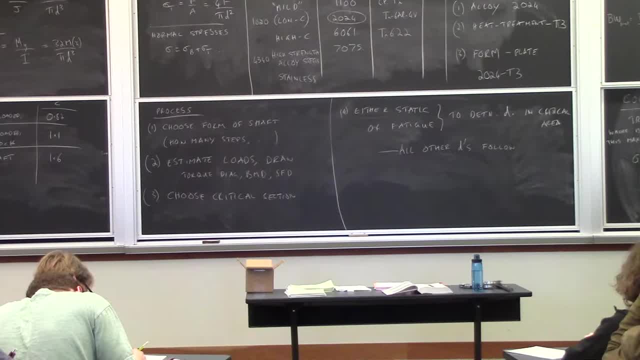 in the critical area. the diameters everywhere else will fall because you decided where your steps are going to be. Basically, you have much more freedom in the place you're going to come from. You can choose diameters because you know you've got a middle factor. 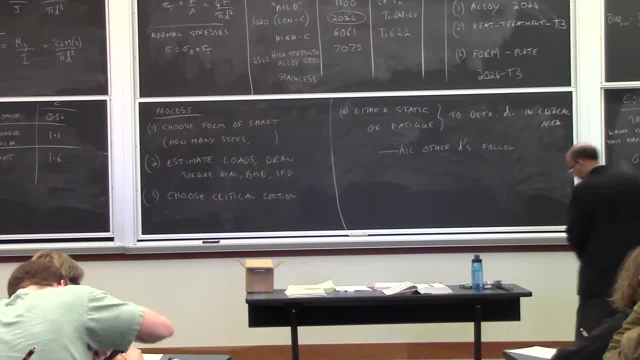 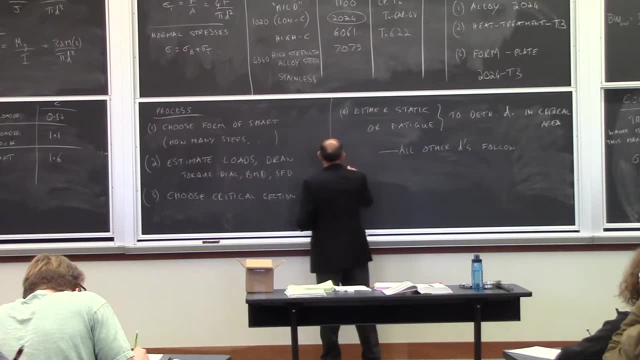 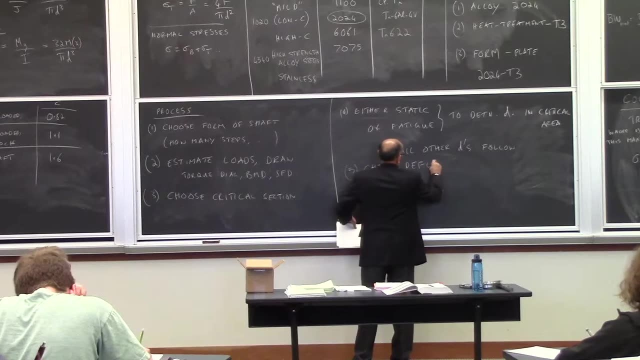 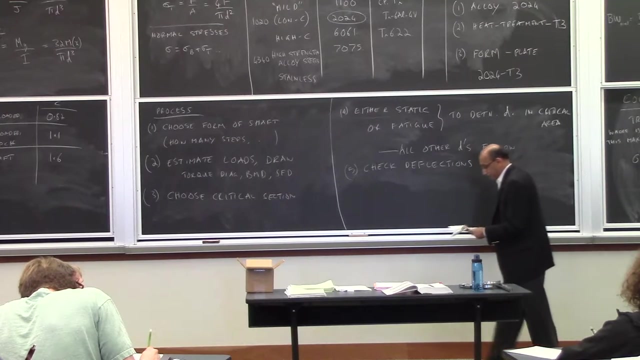 if you get it All right At this point. sometimes you want to go and check reproductions. You'll see that relationship I just gave you. Look at where the bearing's at In this class, because I haven't really given you enough time. 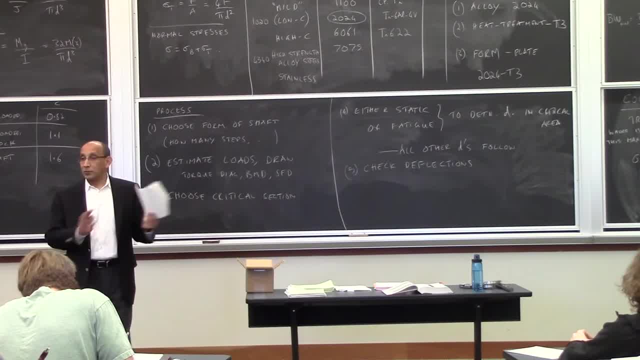 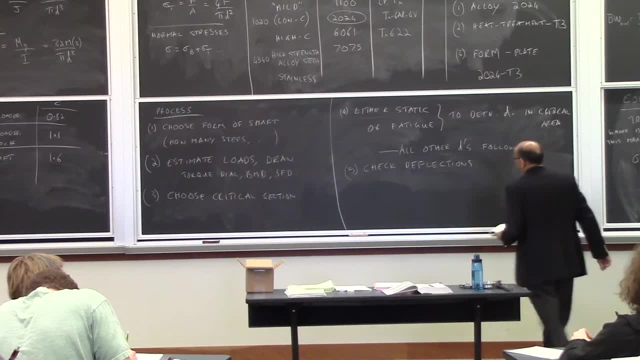 to do what the flexion is going on. Let that go, That one is not going to do it. Then six, something we have not done yet, but I'll show you how to do it later. It's like a very good idea. 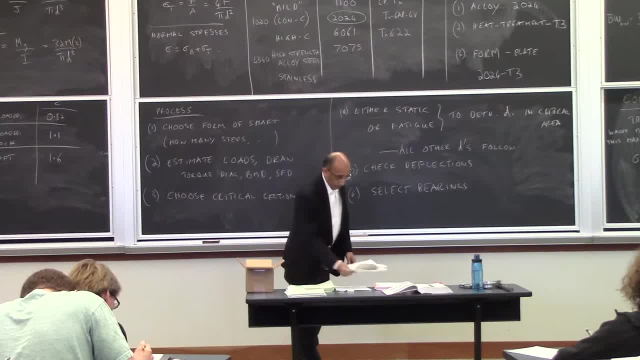 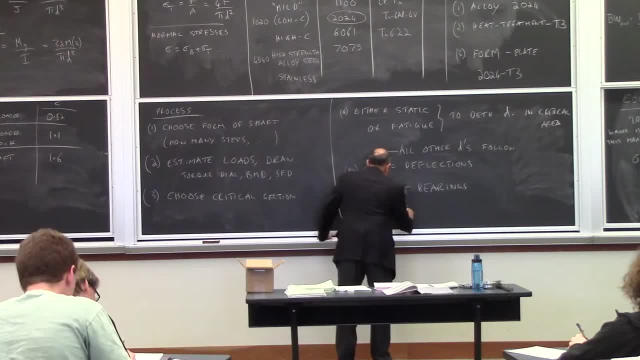 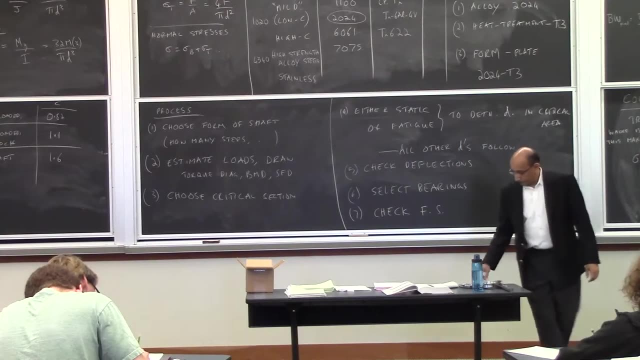 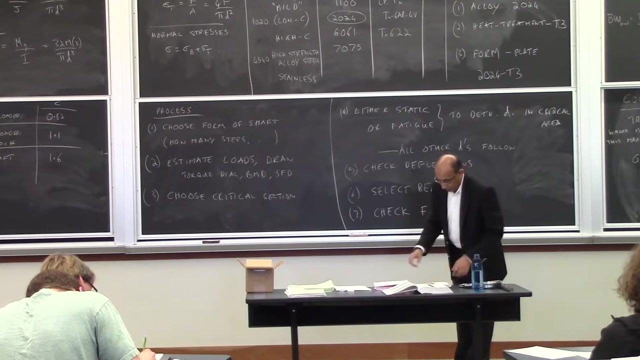 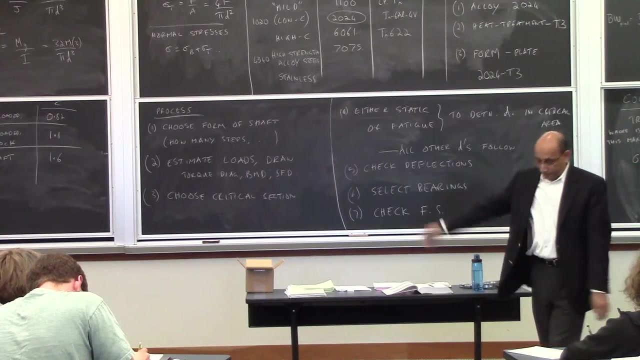 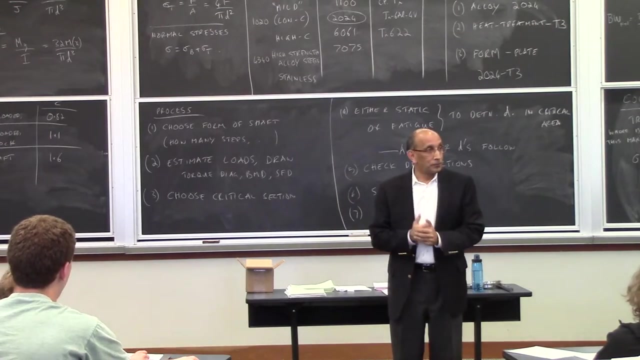 We'll do that a little later in the class. Then we'll check the output Back to the seat. We'll check the back to the seat. everyone, Everyone, please. Finally, straight forward, Pulling together all the things we've done. 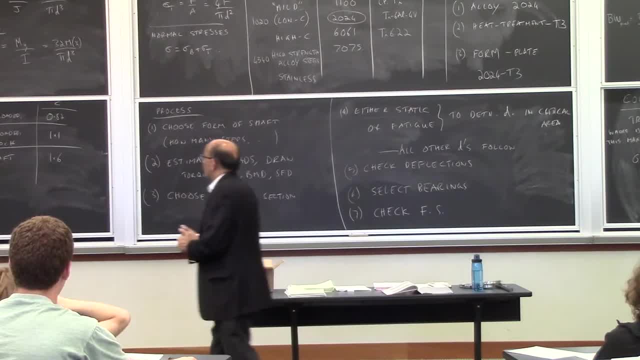 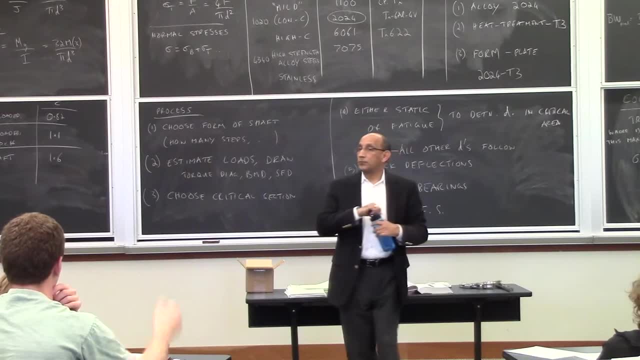 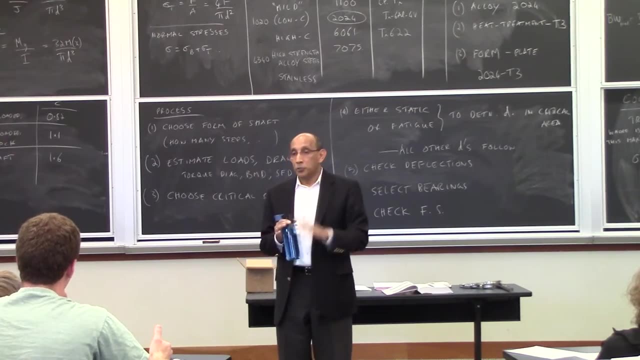 All right Time to change gears. So this is shaft design. yeah, Sometimes you do have to worry about it, So you should always check. Usually it's small, But under some conditions there are very short shafts, very large shuffles. 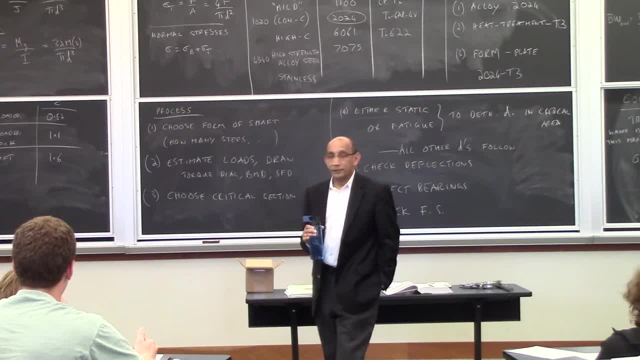 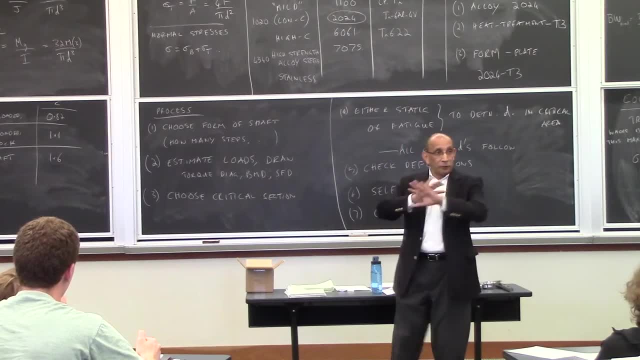 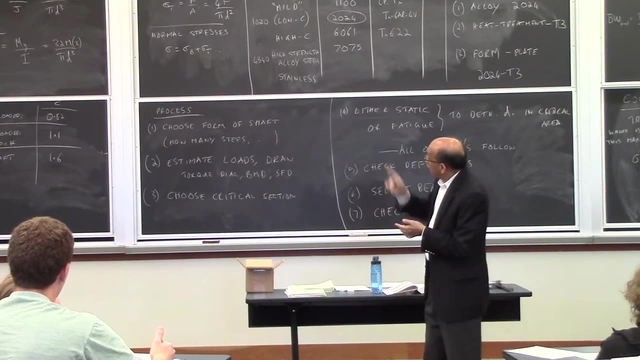 but you can do it, Okay. So this was our first example of a full-scale design. Now I'd like to move to a different problem, but you can see right here where it might become possible. Suppose that, instead of putting my shaft in tension, 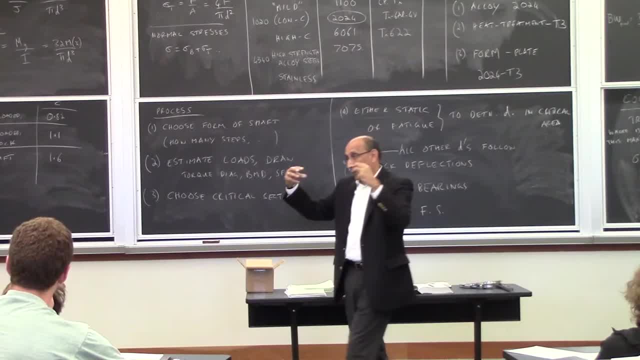 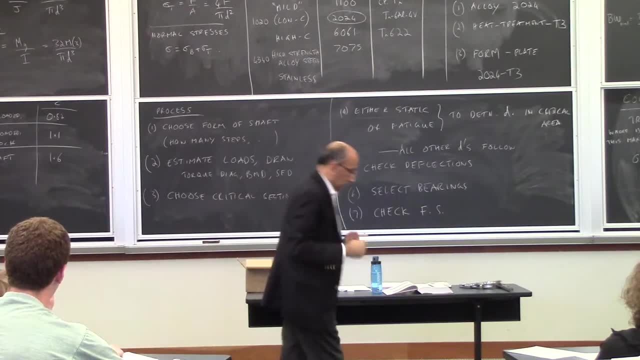 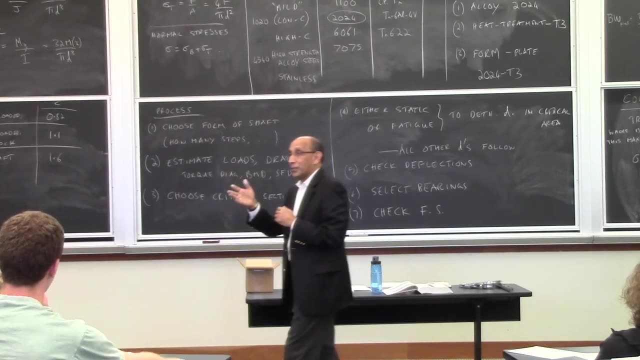 I put it in compression. So we know how to design in tension and we have assumed all along through our calculations that tension and compression are the same. But you know that in compression systems can fail differently than in tension because they can buck. 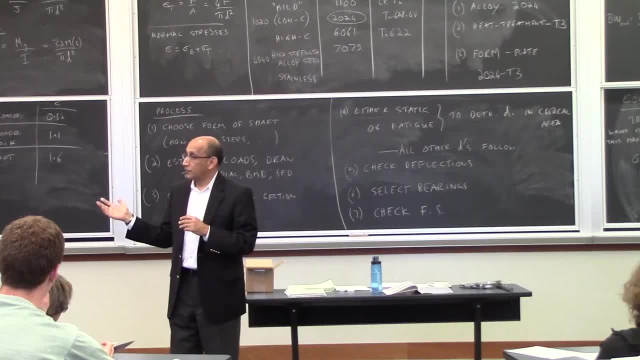 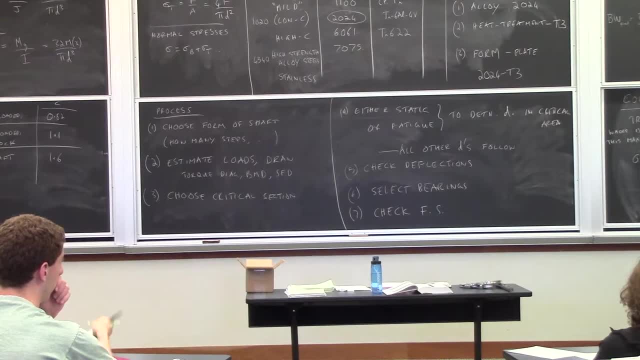 and you guys all have a physical fee for bucking. You'll see, that's how it works. So actually we had some demos of it, but I think this is for the MPD lab too. I don't know, Do you guys think you can make this bubble? 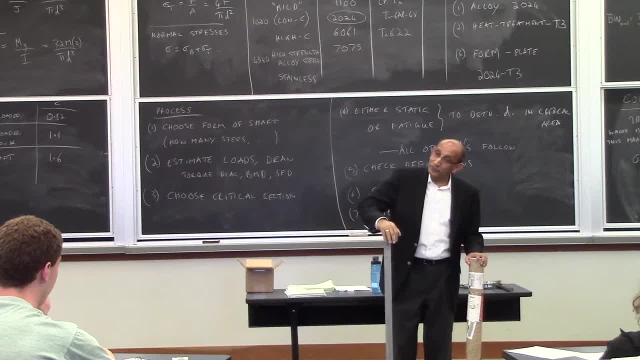 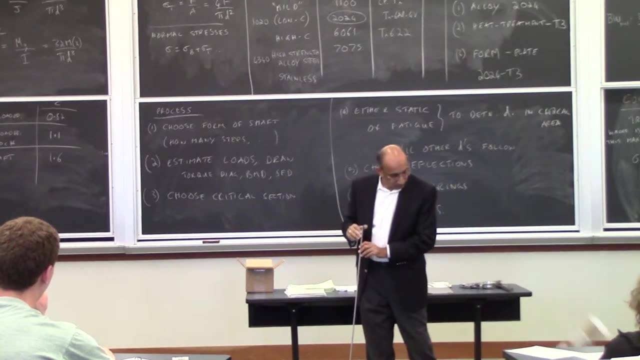 So not that difficult. This is just me. Can you see how much it's deflecting inside this? Okay, I would not say this. On the other hand, you notice it's deflecting this way, but not at all this way. 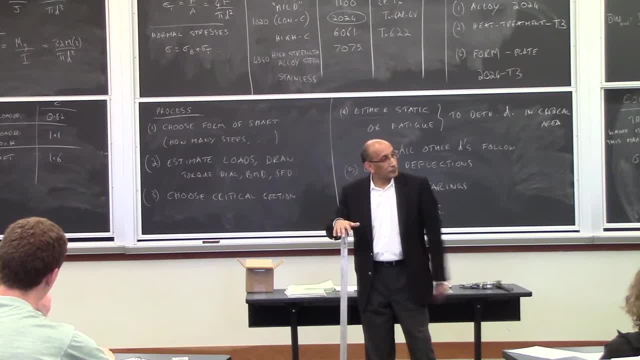 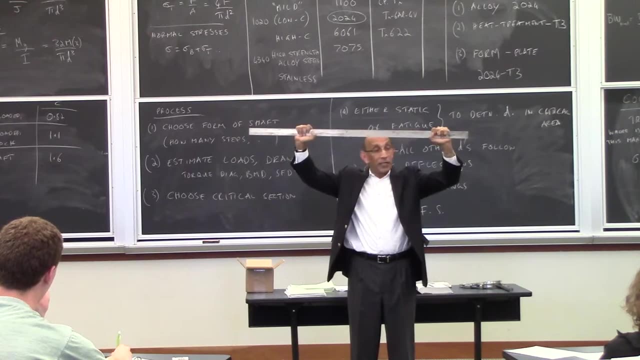 It only buckles back, It doesn't buckle up. So this is a bit like a bending. There's a moment of inertia That, as you remember, in bending, the moment of inertia in this moment is negligible. The moment of inertia this way is very high. 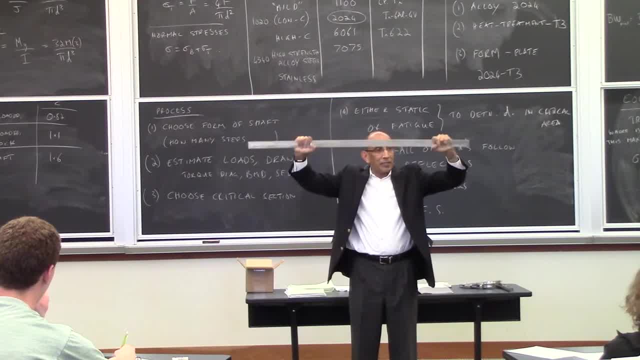 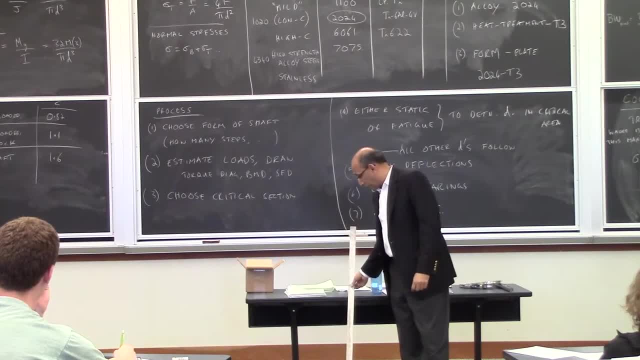 So it can buckle this way because it's like a bending bubble. It cannot buckle this way, Right? So buckling is a limit-mode problem that we have to figure out. There are other examples here. There are things Steve was going to show you. 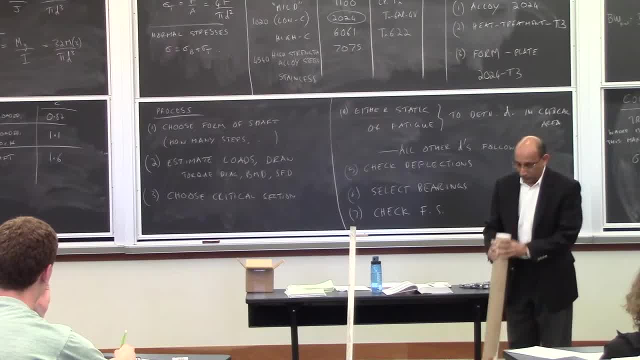 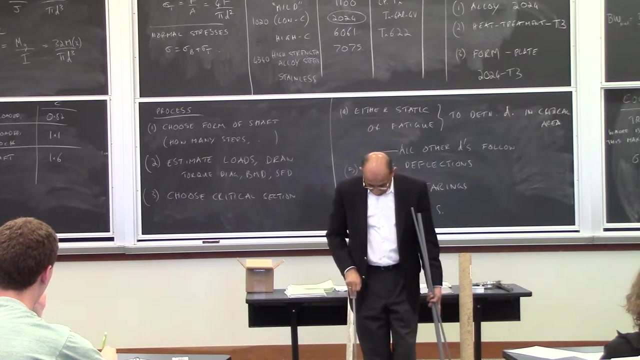 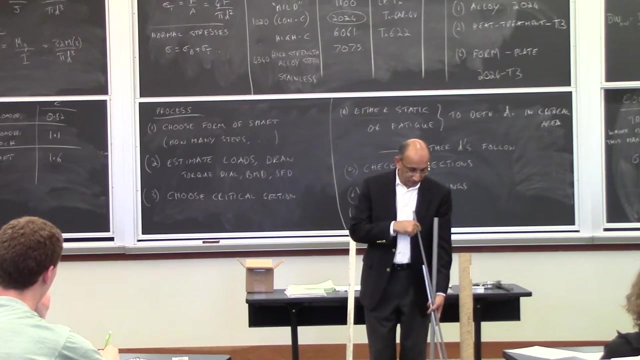 but I'll show you this first and I can get this going. All right, Okay, Aluminum straw. I would actually use it as a cane. ABS straw. I would not use it as a cane, Because it's the same diameter. 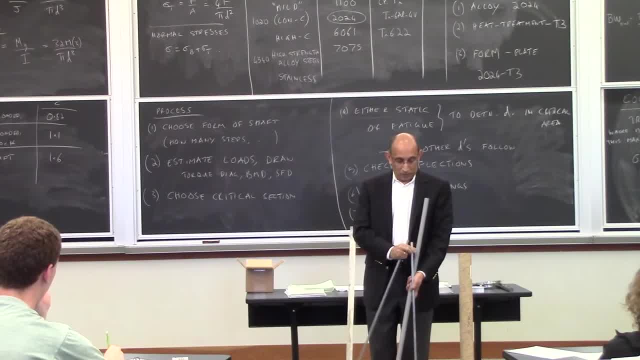 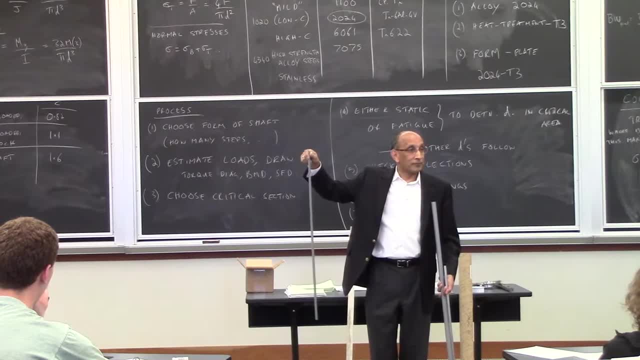 The difference is the stiffness. So these two are the same moment of inertia. but the stiffness of this, the Young's model of this, the modulus of this is much lower. So the Young's modulus of all the other models is in the range of the GPA. 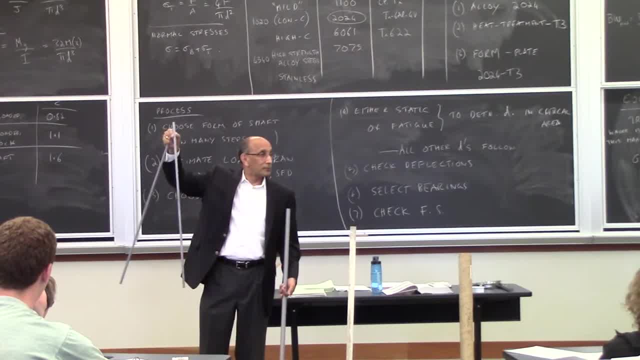 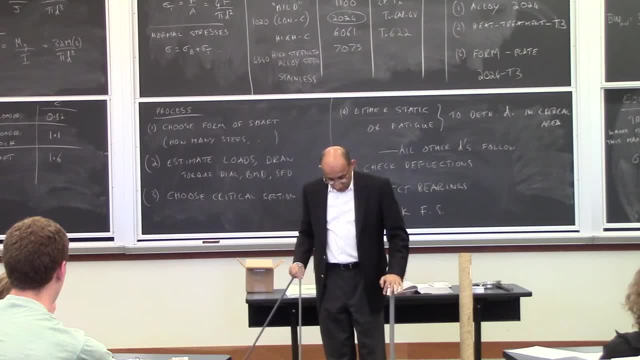 The Young's modulus of this thing is like 70 GPA. Now this thing has the same Young's modulus as this, but yeah, it could be this big. So if I take my moment of inertia up higher, I'll be able to survive significantly. 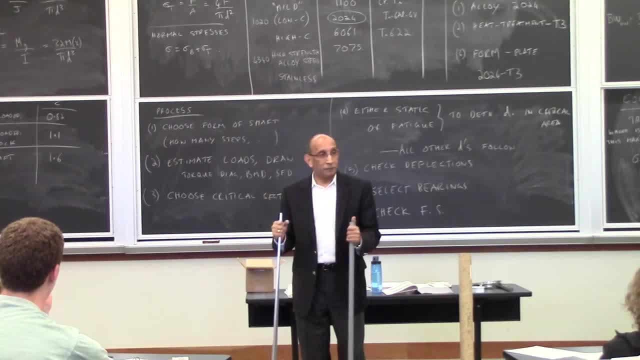 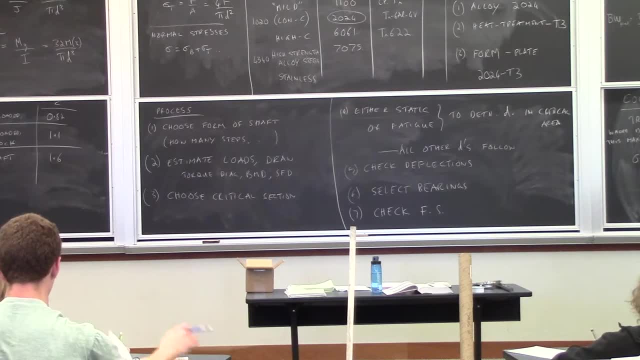 So that's the basic. We showed you right here that buckling is a form of bending. What's happening is: let's just think this through for a minute and I'll put it in this in the next class, But you guys need to understand how this works. 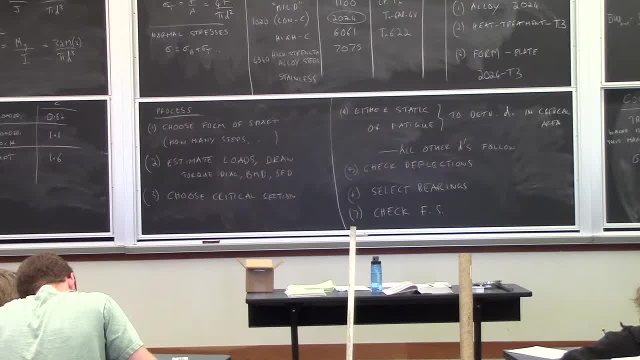 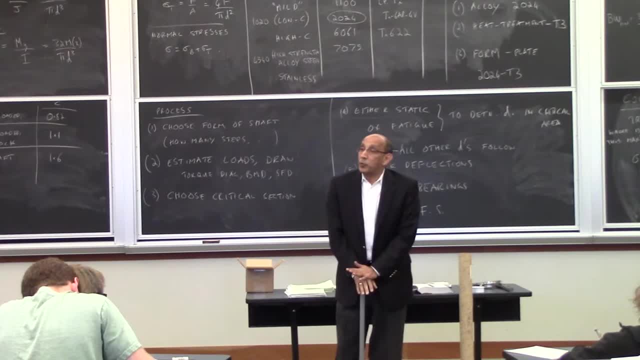 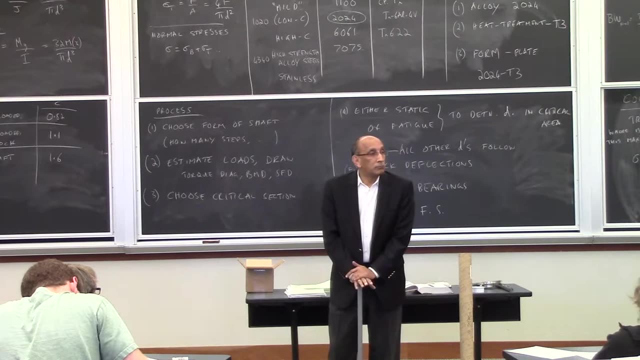 So that's actually the name. Stop by thinking about it a bit like a mathematical problem. If I were to analyze this as a compression problem, what would I do? I would take my applied force divide by my area and I'd say: it's whatever the stress is. 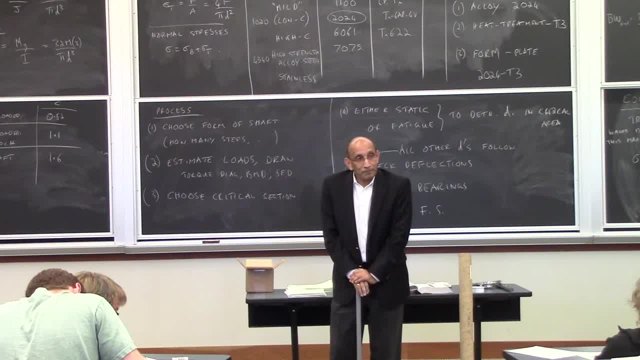 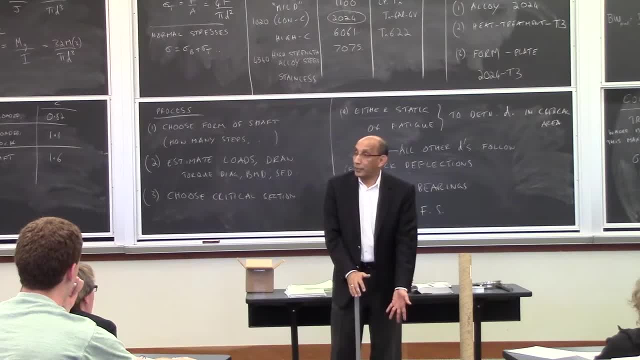 that stress is below you. I'm safe If I try to analyze this as a bending problem. well, I don't really have a bending moment. It's straight. There's no bending moment here. On the other hand, what's really happened there? 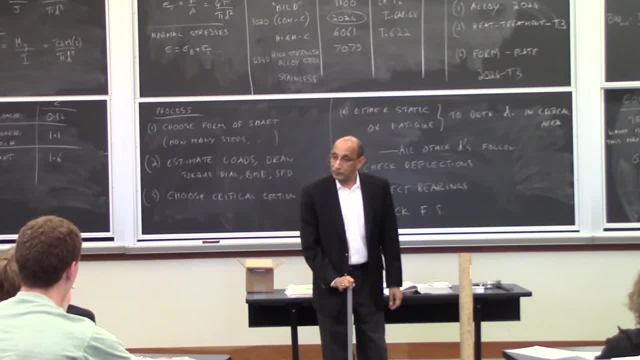 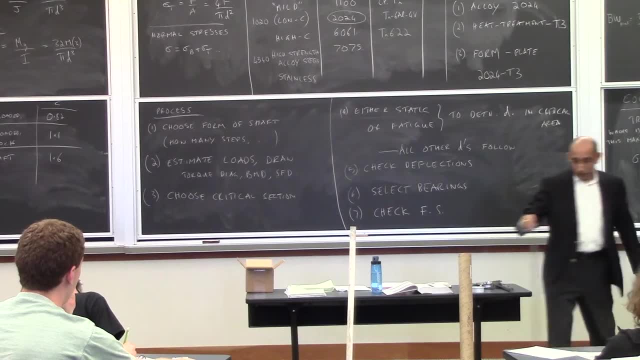 was. you assumed that this thing was straight and stayed straight. That's how you did the problem. But if I take this rod and I look at it, obviously I can solve it as a simple compression problem. Applied force divide by the area. that's true. 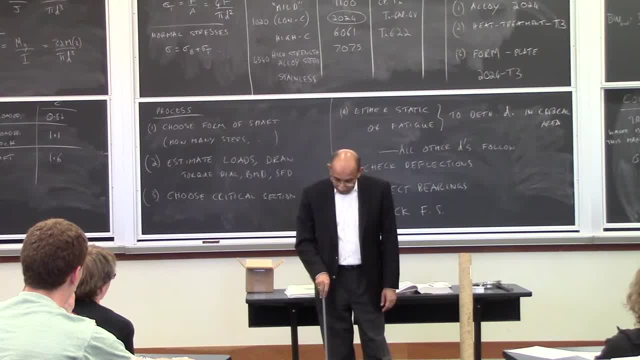 My stress is too below your stress, But the fact is, if I apply a big enough load, it does bend Once it begins to bend. now I have a bending moment. So the real question is: when do I switch from being straight to beginning to bend? 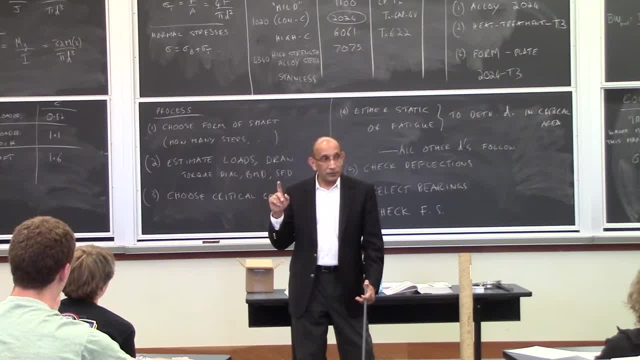 Mathematically. for those of you who like mathematics, this is the fact that when you did the analysis, you assumed there was only one answer, When really there were two answers. There was one answer if there was bending, and there was a different answer if there was no bending. 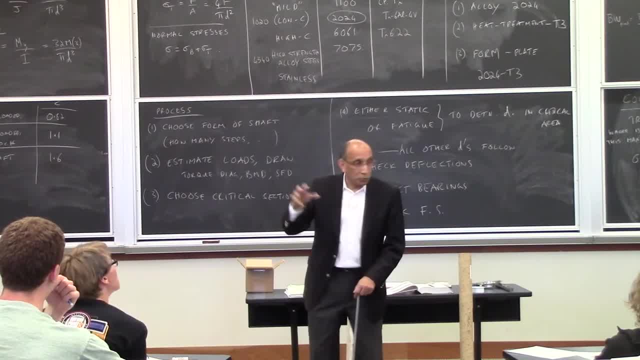 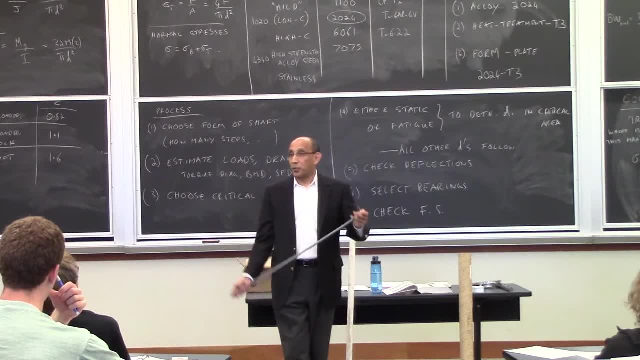 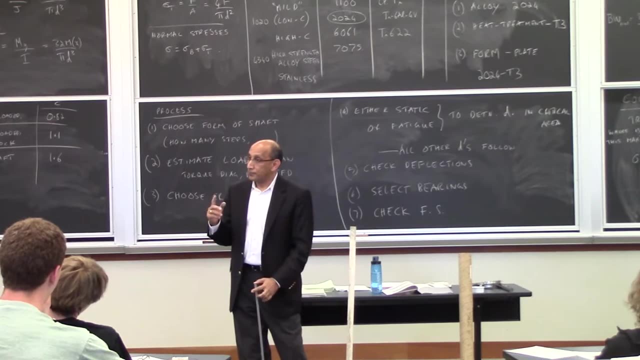 And you did only the answer with no bending. Your assumption prevented you from seeing one possible solution. So there are mathematical ways of setting up problems so that you can automatically get all the possible answers. There are multiple solutions, down to one problem, Depending on the mode of estimation you get. 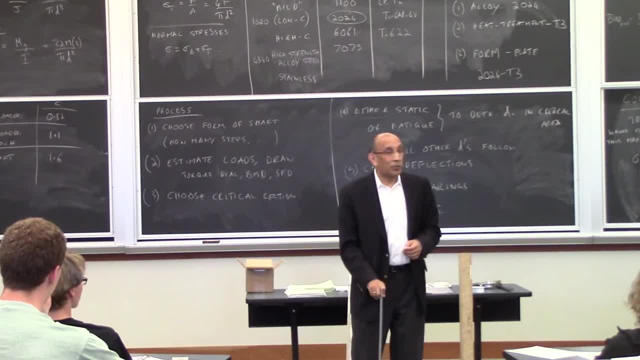 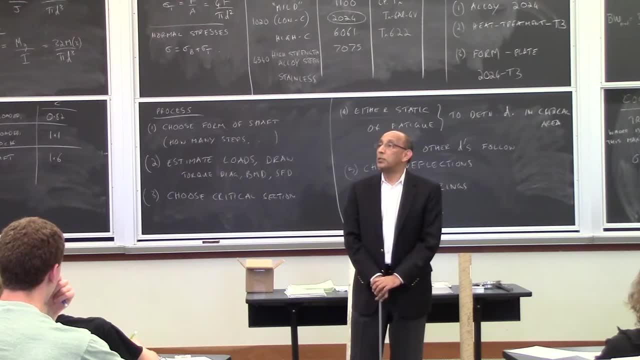 So this is a change in the differential equation. These kinds of problems are called stability problems. The question is: is your system stable? Is the box stable? Bottling is a stability problem. It is the stability of a column. So the reason people were able to bring down 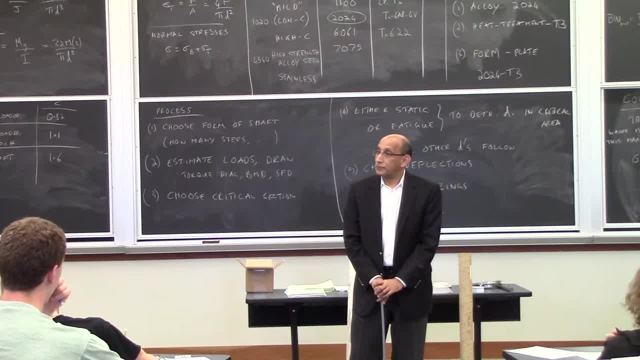 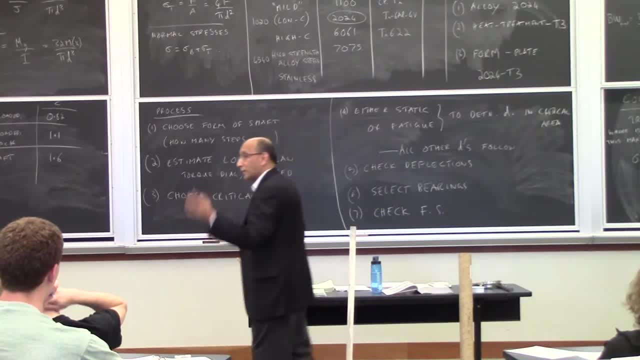 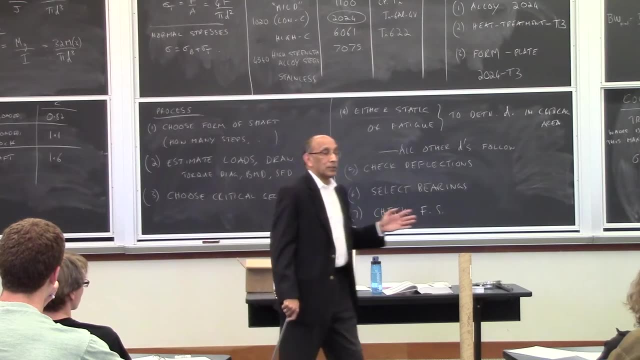 a concrete center was bottling. So if you put planes in, the steel in the towers was designed to carry the loads of the towers Without bottling. The steel in the towers was actually designed to carry the loads of the plane as well. 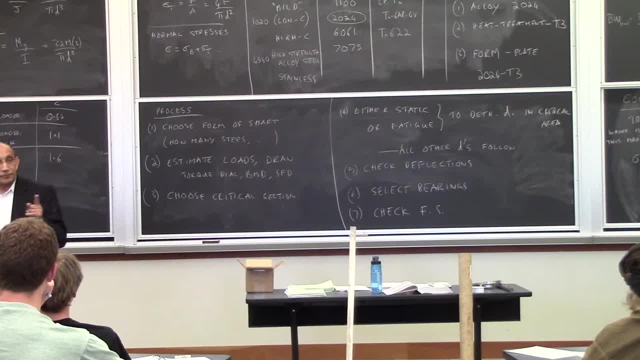 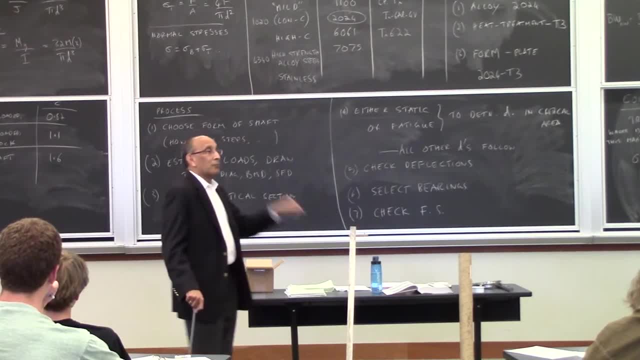 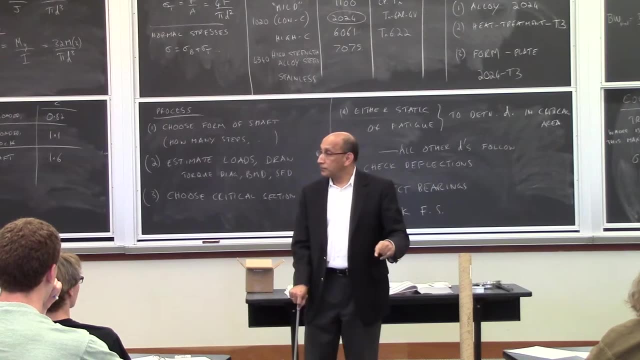 if the plane were in the towers Without bottling. But the plane exploded. And what if you look at the spot on the side of the Everest? The temperature inside the columns went up. The steel became soft. The Young's modulus changes the temperature. 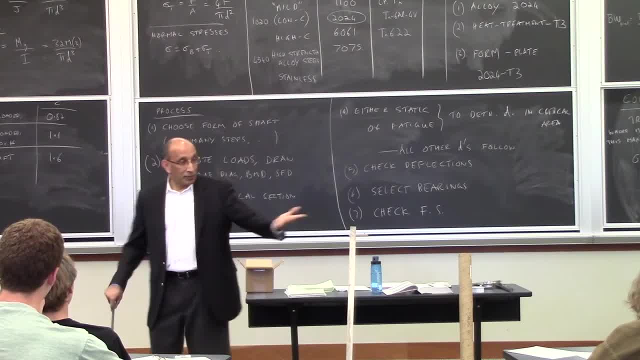 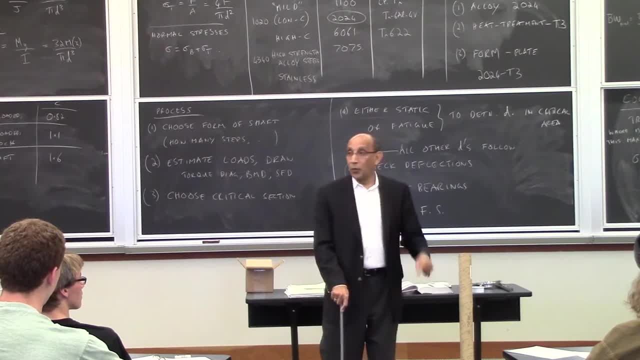 at the temperature of time. Obviously, if you measure something, the Young's modulus is very zero. but it's little. The Young's modulus stopped. The system began to buckle Once one part began to buckle. now the problem is the stability problem. 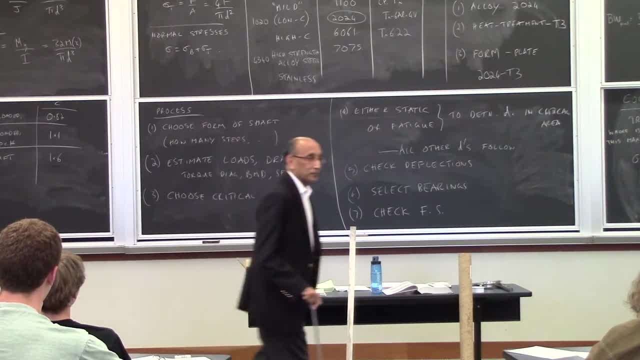 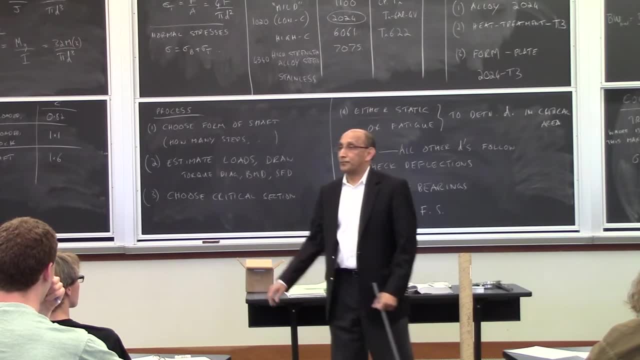 Stability was never designed to have part of the problem. The building was designed to always stay still. If one part buckled, the whole system buckles. You can design a building so that one floor will buckle and the rest survive, If you're doing earthquake design. 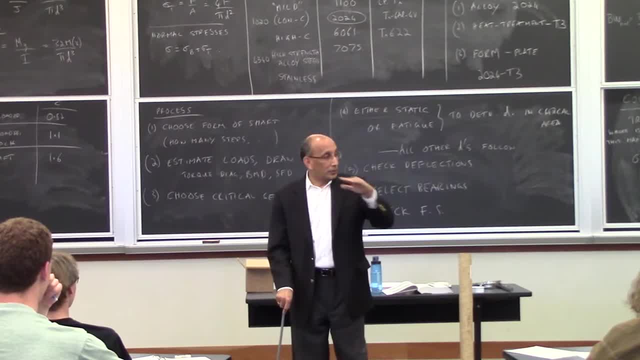 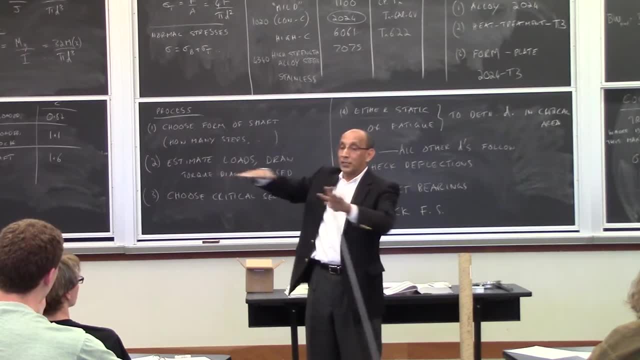 you do this all the time. If you design the building so that you can lose one floor, in fact you can have. if you go to Kobe and look at what happened after the Kobe earthquake, you had rows of buildings where the entire building. 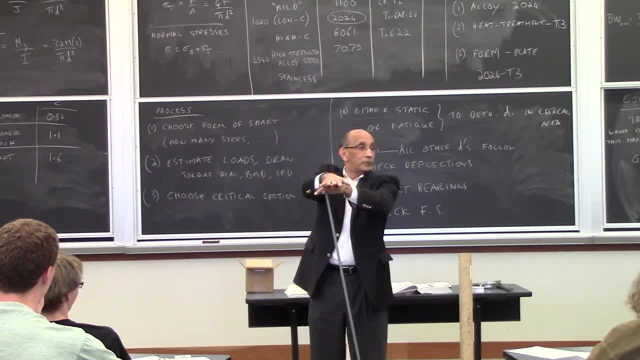 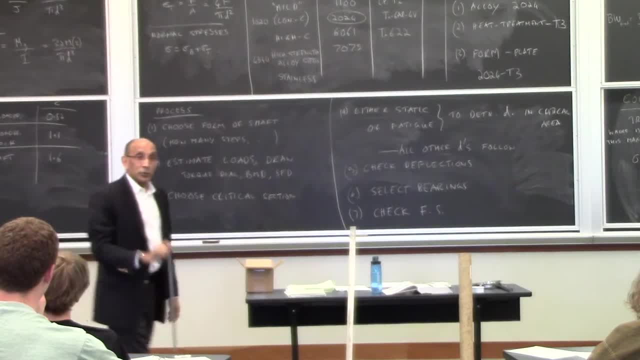 essentially collapsed one floor down, But the building was still there. The other floors were still there. the water floor was still there. the floor in between is gone, But you couldn't have done that with the steel tower that we had in the water. 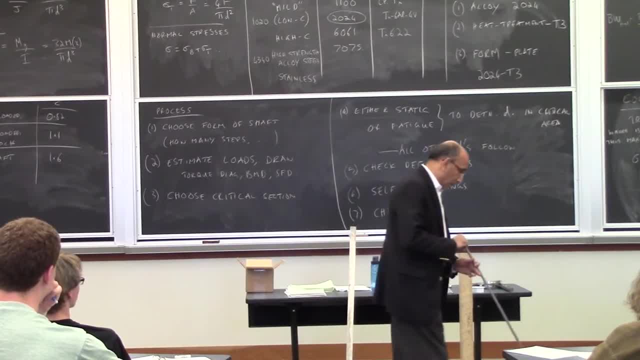 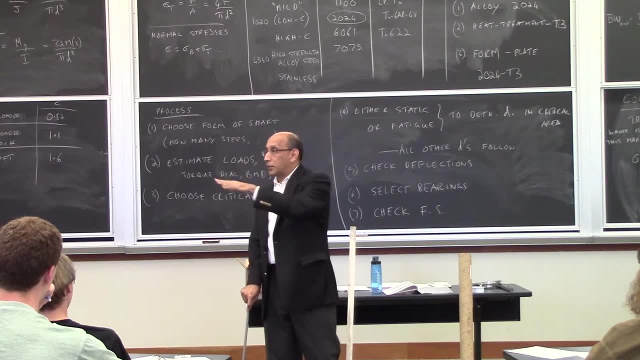 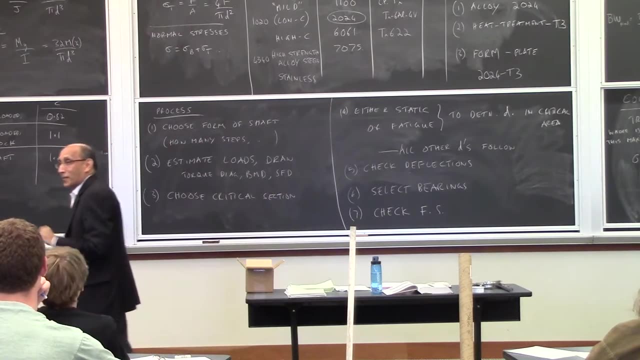 So that was the design. So that's one example. Another place where Buckley misquoted: When you guys have your, if you look at your typical phones like she's looking at them, if you look at how the phone fails when that phone fails. 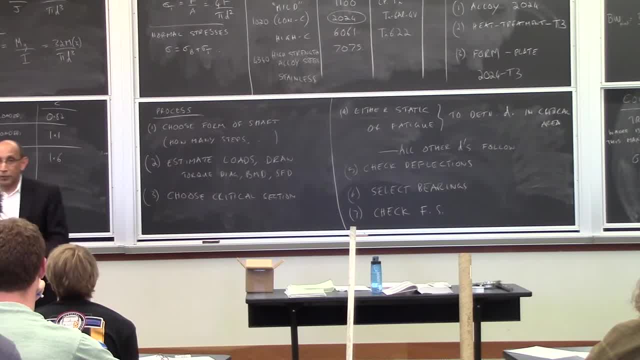 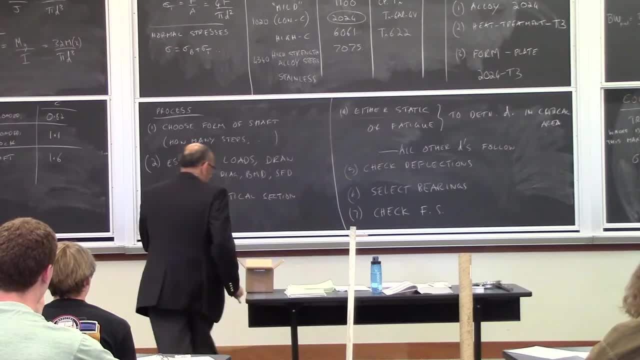 almost always it's failing because you've got a problem. So there are these wires right. So if you think about the phone, let's say: this is the silicon wafer, Let's use this. So this is the silicon wafer. 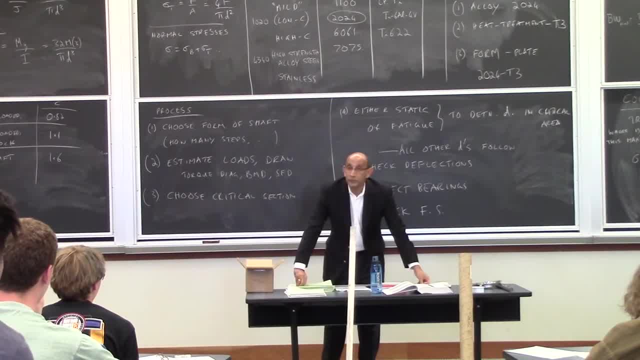 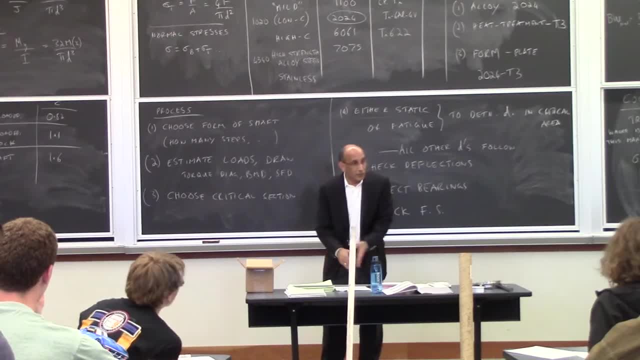 This is the chip. On the chip, I've got a metal wire. It's my copper foil. I'm putting down a load, a thin strip of copper. This is the conduction right. I move electrons along this, So this is copper. 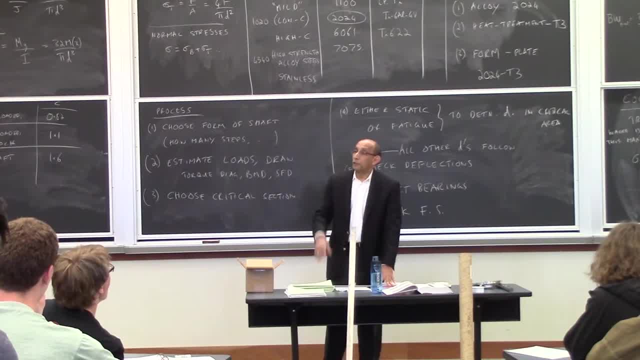 which is relatively low. Coefficient of thermal expansion Underneath the silicon. I'm sorry, relatively high coefficient of thermal expansion Underneath the silicon. relatively low coefficient of thermal expansion. I use my phone for a while. The whole system warms up. 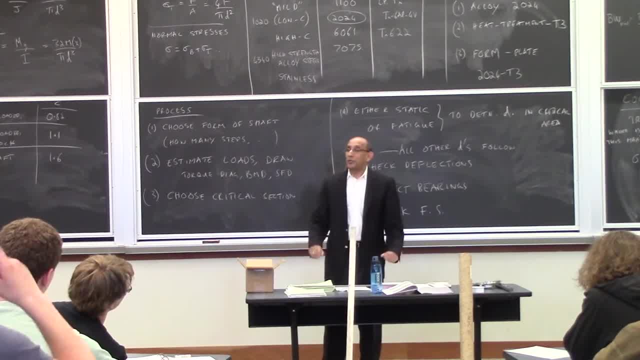 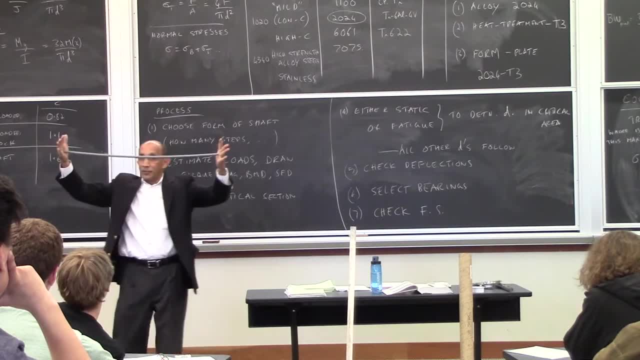 This wants to expand a great deal. The silicon says: I'm not going to expand that much. So this effectively wants to become longer. The silicon says: I won't let you become longer. That amounts to squeezing this in The copper buckles up. 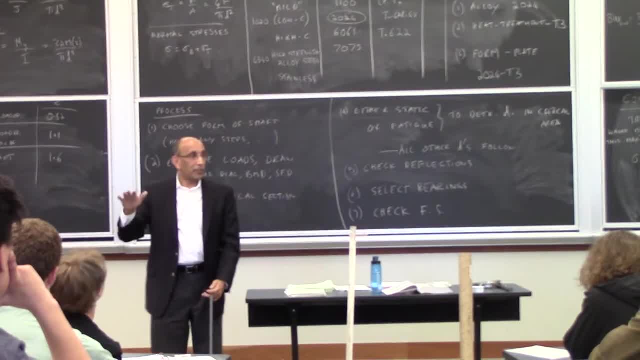 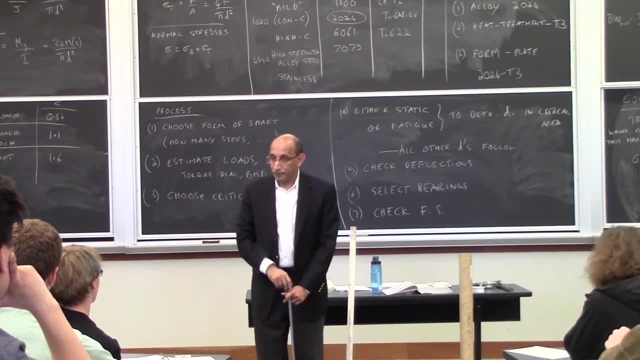 and your phone stops working. Buckling instability is what limits most electronic devices in terms of use. So you said that we couldn't design it. We did not, We could, We could, We just didn't design it appropriately. Could we call that an design? 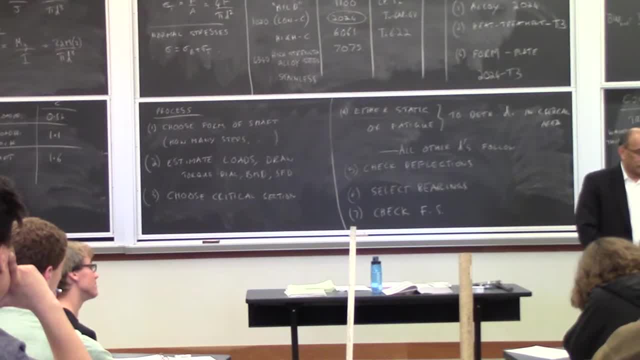 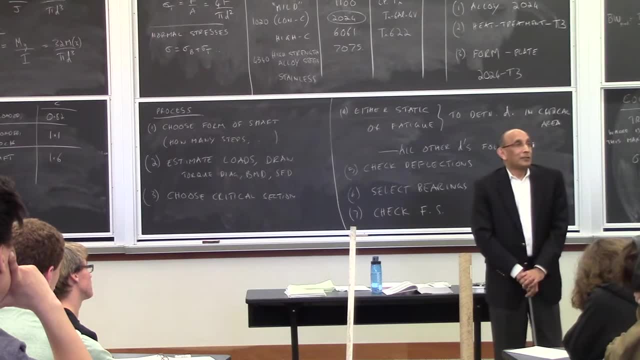 I mean as far as a person with vision and more of a sense of hey. by the way, I want to make sure that I don't crash into this Right. Well, I think you're asking a philosophical question. So the question is: 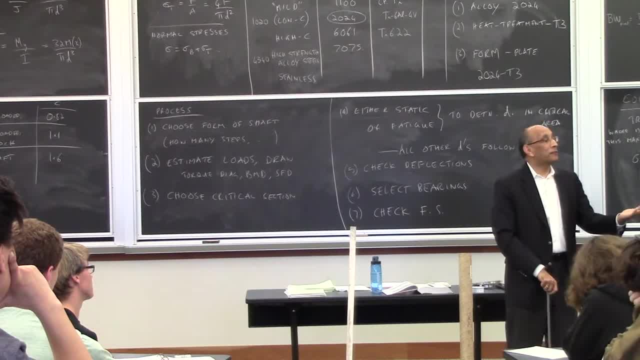 was it a design flaw? And the answer is: as far as the designer was concerned, this was not an additional issue that we just began to design. That's cool. Whether you call that a flaw is a question of how you develop your system. 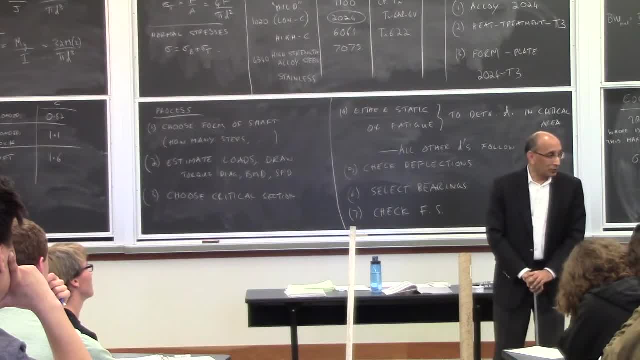 I wouldn't say it's a flaw. You can tell people what a design flaw is. That's it. Another example that might be kind of wrong is to look outside and look at the trees. Now, that's an apple tree, but look down there. 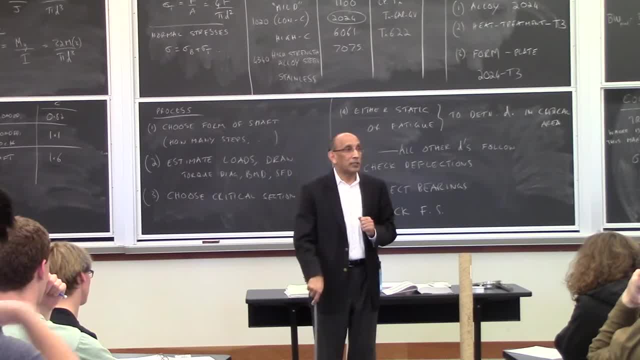 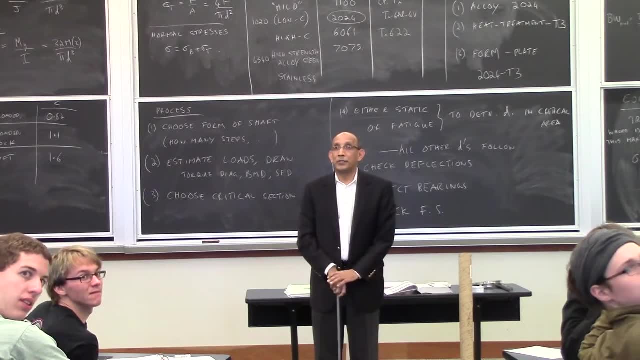 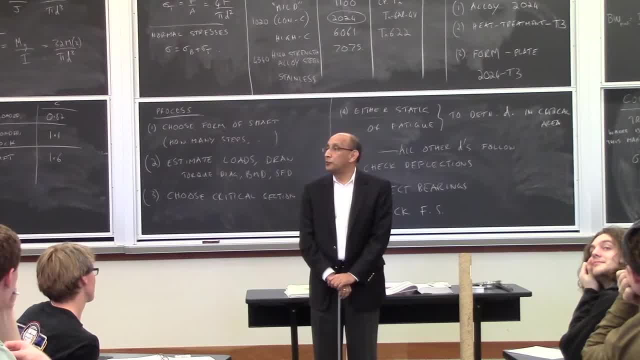 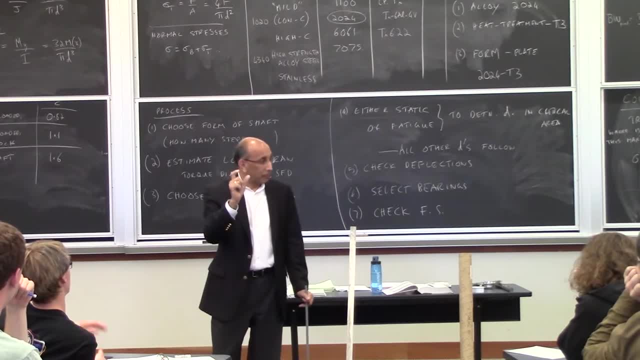 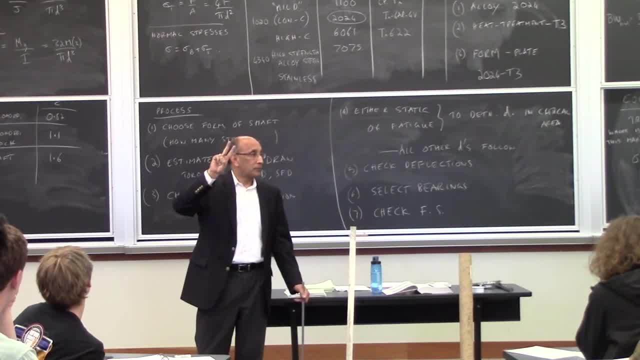 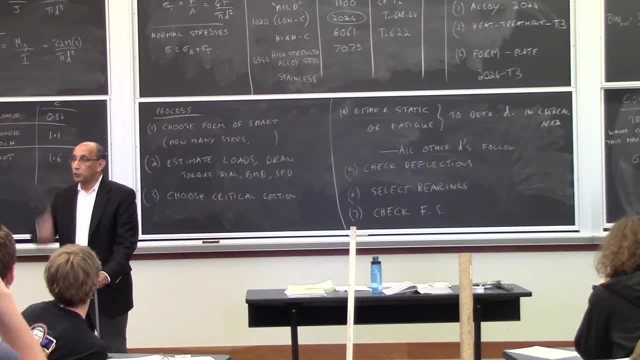 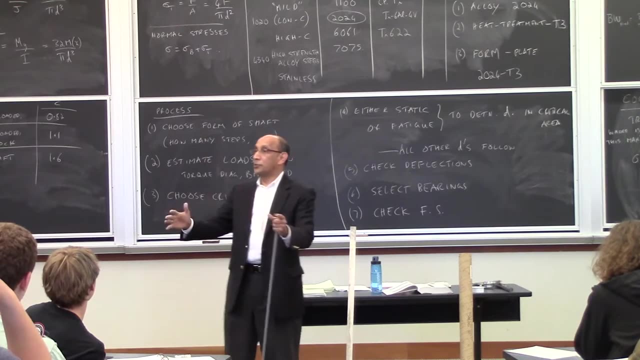 into a bubble, into it. That's what the trees do. They suck that stuff up from under it. water the nutrients mold it up, grow the tissue. they grow the leaves. you increase the mass. The same tree which initially had no load up in front on the top. 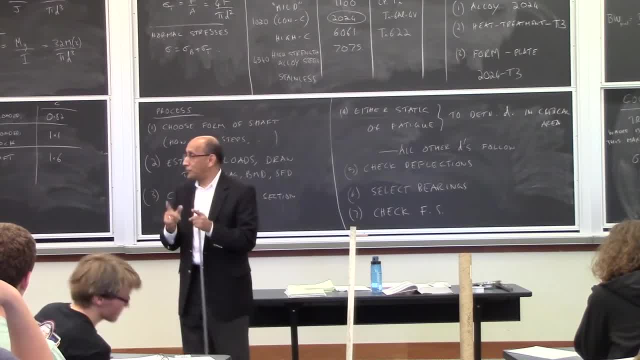 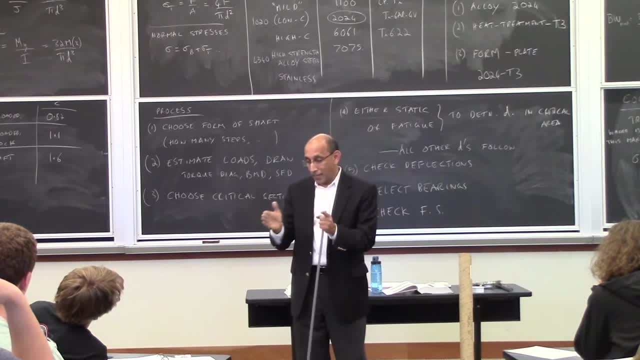 now has all that load from the top. The tree trunk is designed to carry that load, that to carry wind loads. You can look at the ratio of the diameter of the trunk to the length of the trunk. That's determined by the bottom. 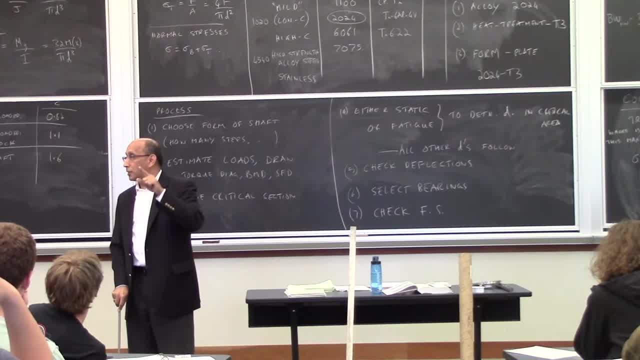 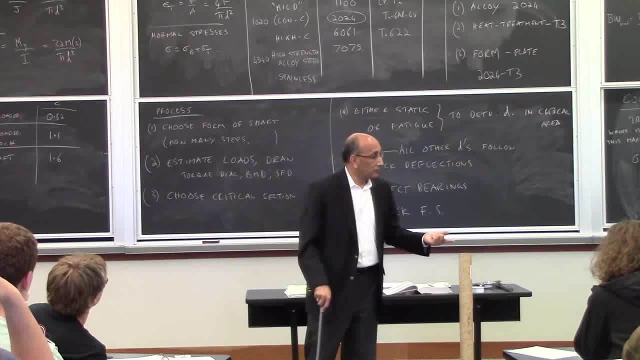 So how trees grow is determined by the bottom. How far they grow, how fast they can grow, how quickly they can recover in the spring, that's determined by the bottom. The strength of the hillside is determined by how much material they move up. Each time you move that material up, you're taking it out of the soil. You're going to change the ground underneath The trees will compact. That's what it will do Over time. that erodes the hillside. That affects the hillside. 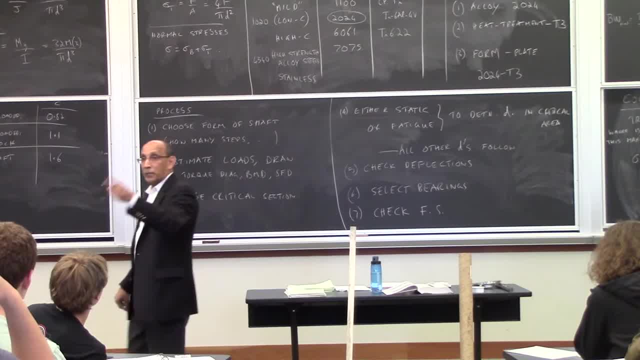 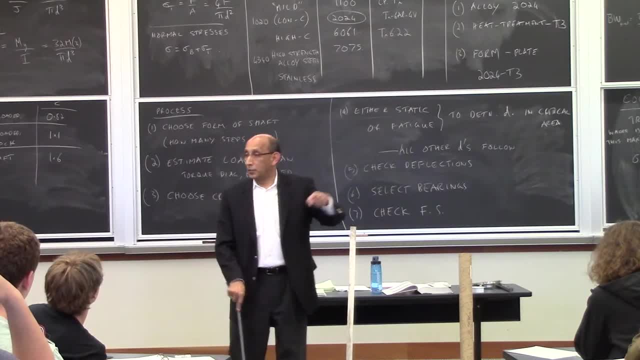 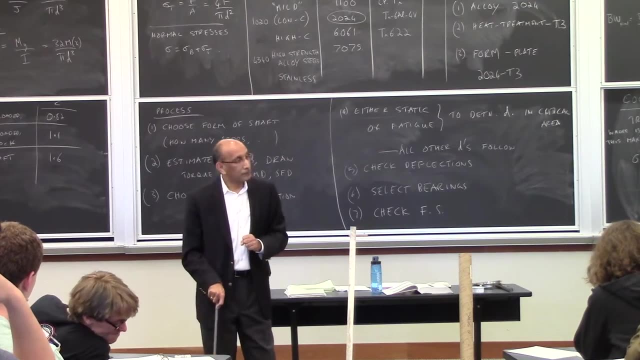 You change the compaction. If you are a paper-making company, you decide which side of the hill you're going to harvest the trees from, based on how bubbling the soil is going to grow. As the trees are growing, the roots, the roots embedded in the earth. would that compensate for? Well, the roots really are determined by the diffusion problem. They need the food. They keep going for food. They're not. That's determined in the long term by how you can transport material, Not so much by the mechanical load. 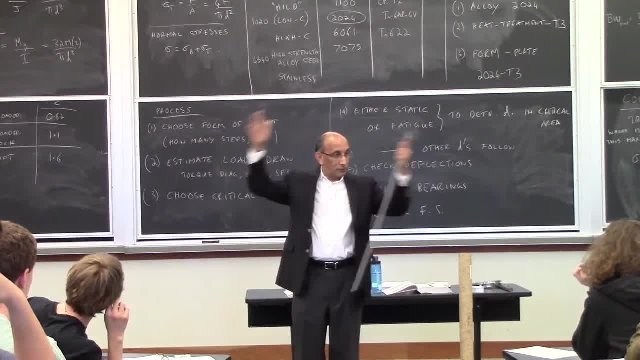 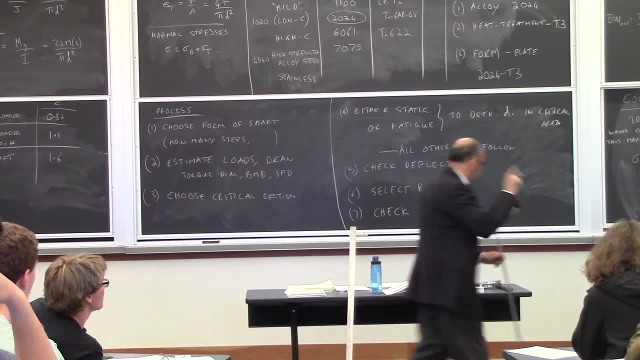 So one reason you don't see very tall, thin, heavy trees, that's because it's bubbling. And the last example I'll leave you with before we head out: oh, I do have a clicker that I'm going to need to buy. Sorry, And they stalled. there was a bunch of companies that called the railways and then it was nationalized and then it was denationalized and in the process they lost the data. 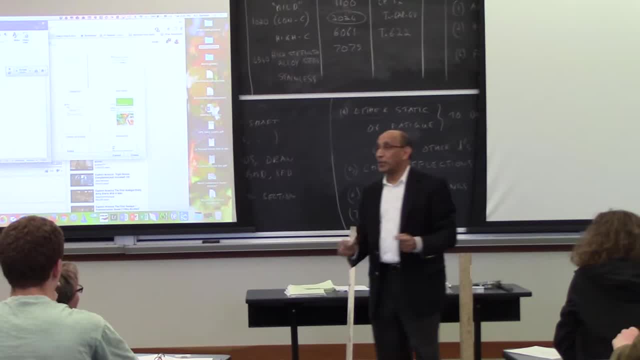 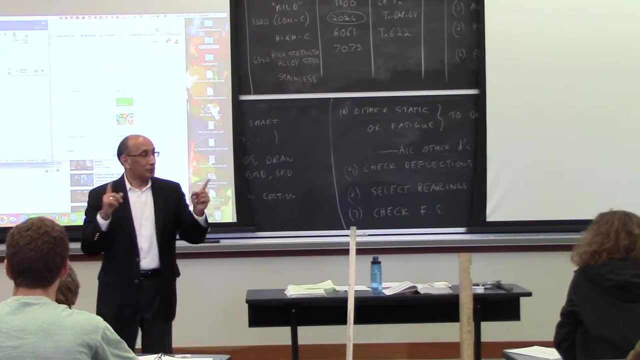 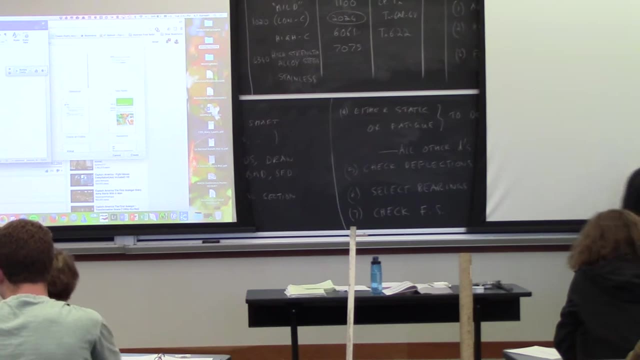 They don't know which joints are safe, and so they shut the entire system down to 30% of the output speed because they don't know which lines are still safe. So let's look at this, So let's go with the first one. 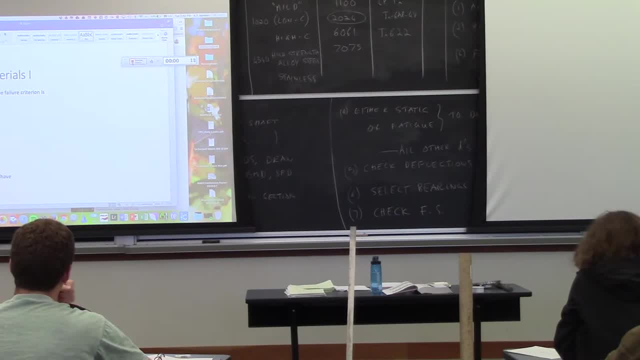 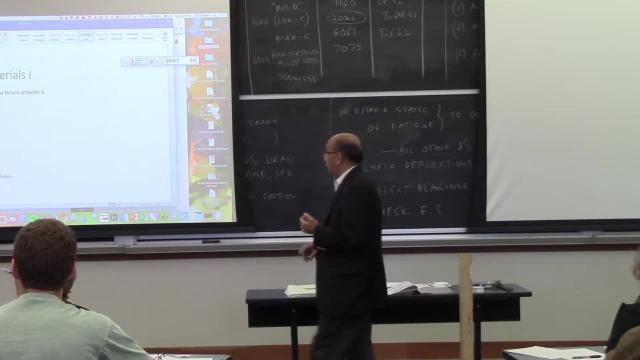 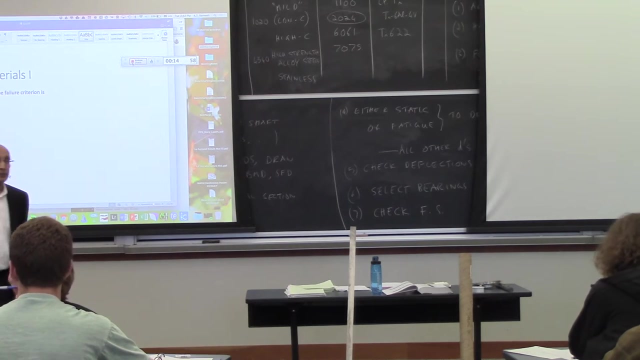 So the most conservative team in the country, Global. One of my friends went to the Golden, All right, All right, You have a second All right A team here. Would you like? 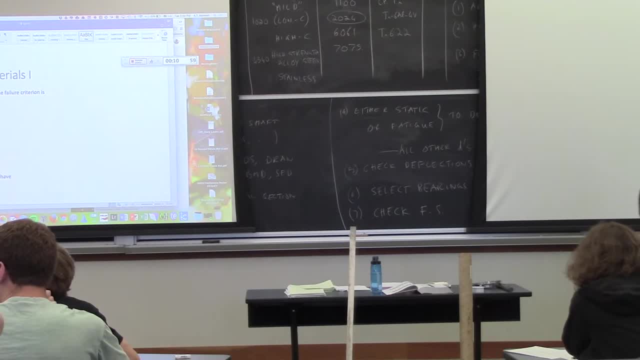 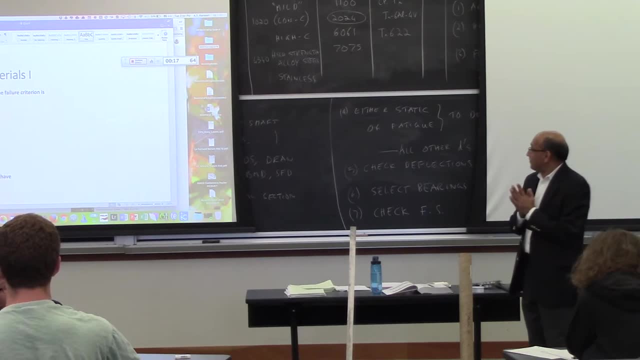 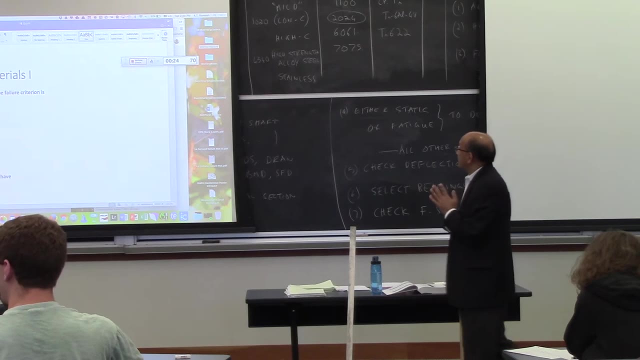 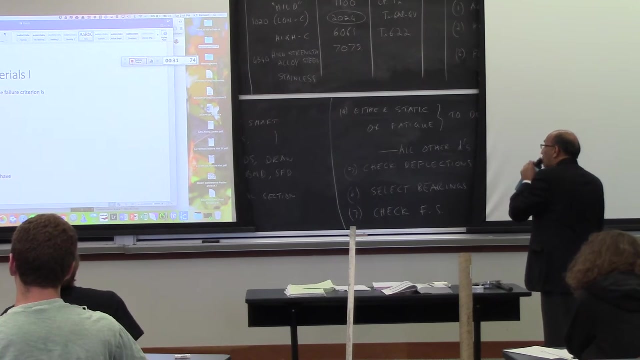 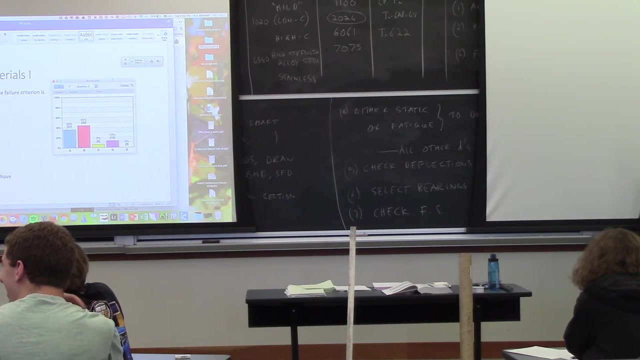 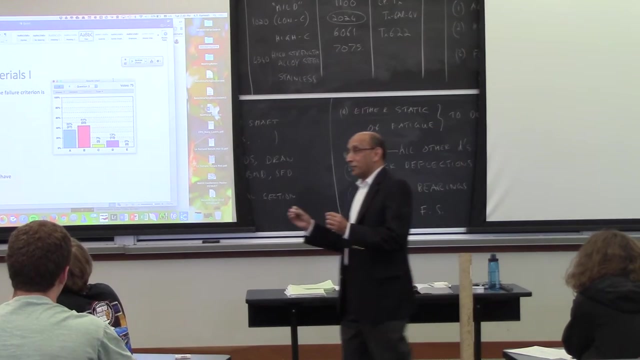 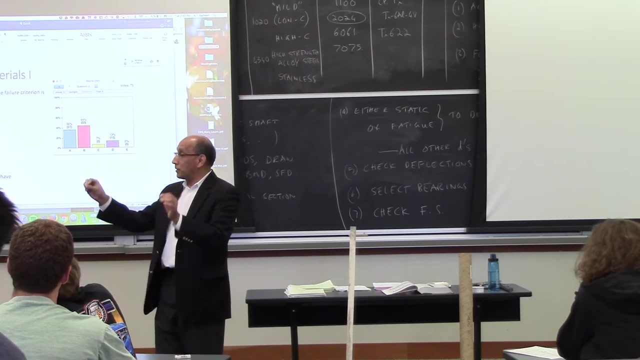 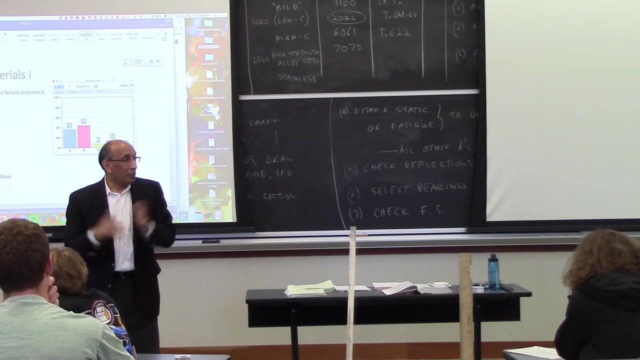 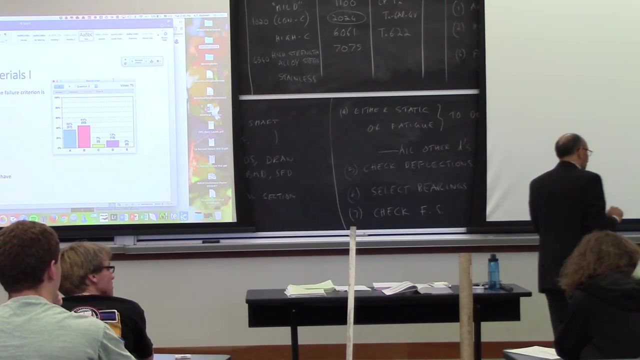 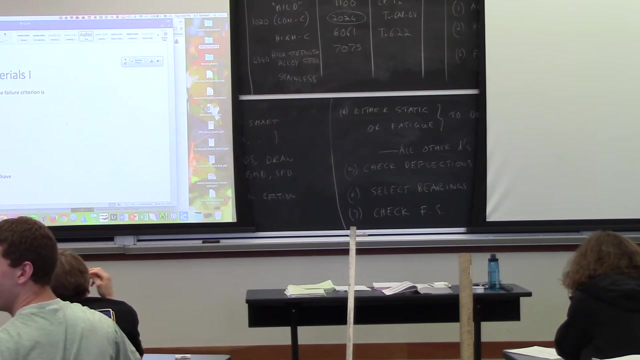 Thank you. Thank you, Fatigue is now a definitive answer of one of the three. It's a probability of one of the three. Okay, So what's wrong? Ice turns steams. 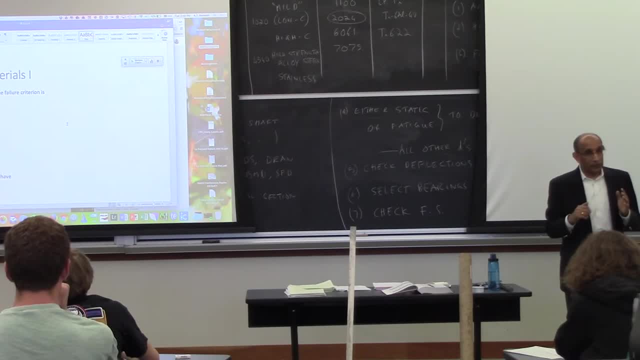 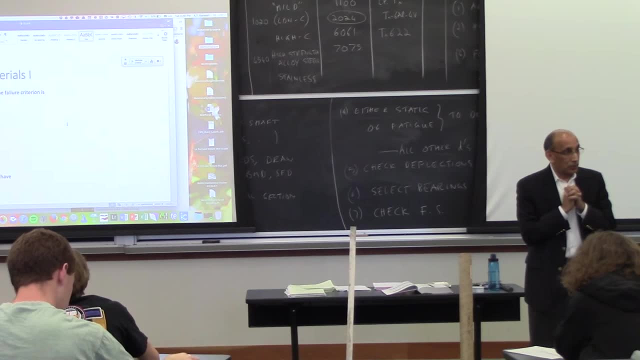 So we talked about strain hardening. Tom talked about this the last time around. We don't want ice turns steams now. We don't know if you guys want to listen up, but let's put it there. So it's an ice plant. 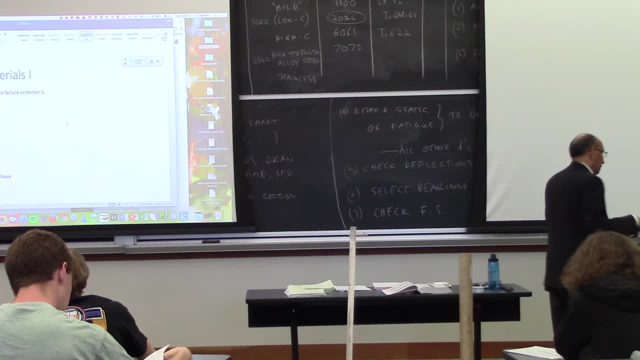 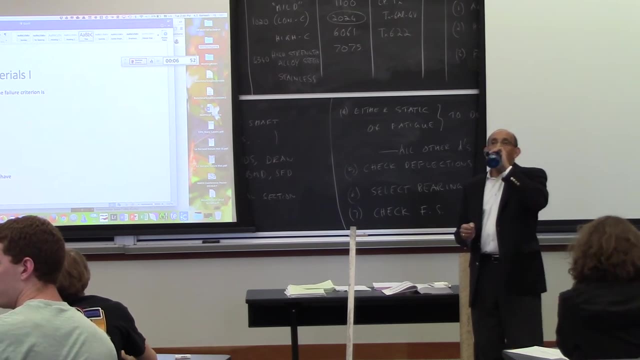 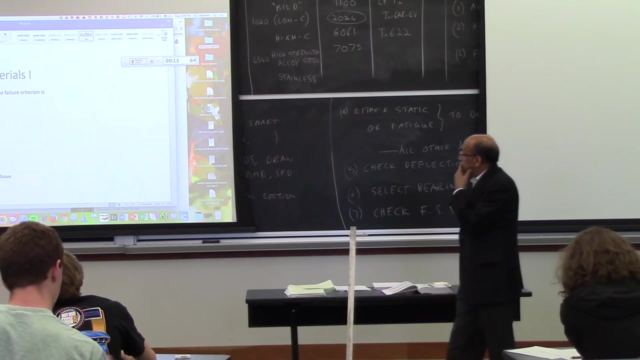 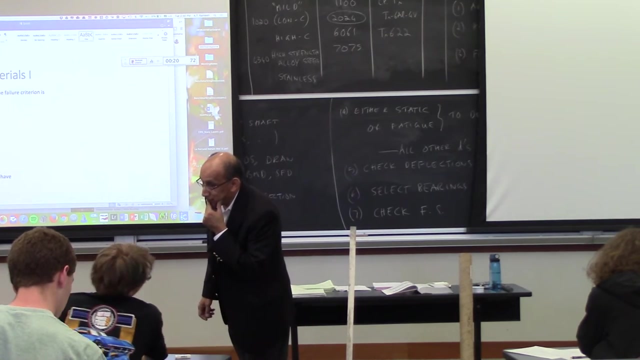 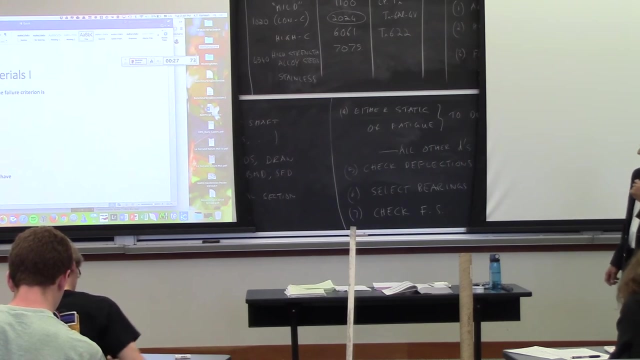 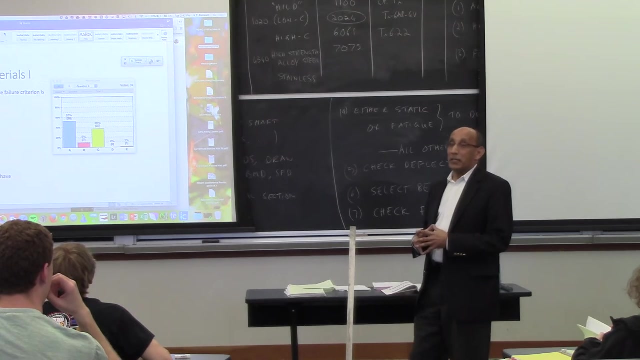 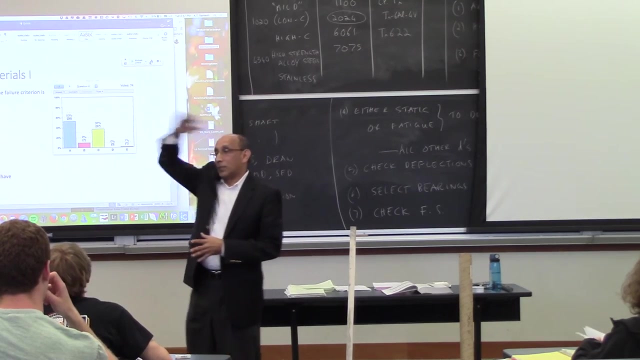 but it has ice strain hardening, no strain hardening, Thank you, Thank you. So the answer is actually more like B. So generally, what happens to the steams is, if you make them really strong, it's hard to get a high hardening atom. 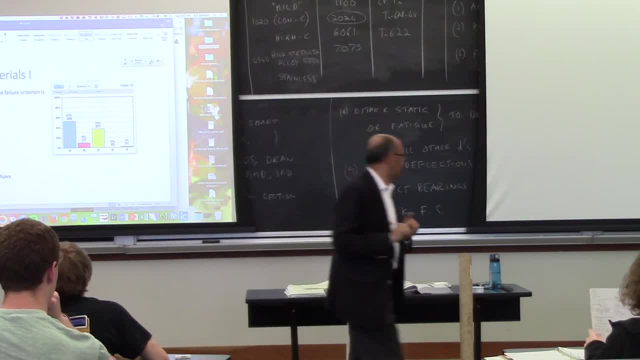 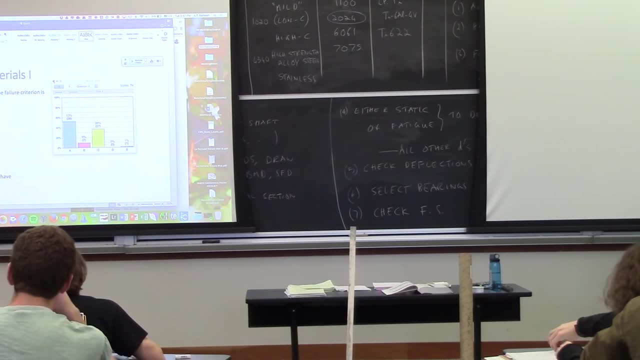 So I need to explain that a little more. I'll come back to it, And the last question I have here is really designed to evaluate a little bit about what to do with hardening. So if you have more hardening in the steam, 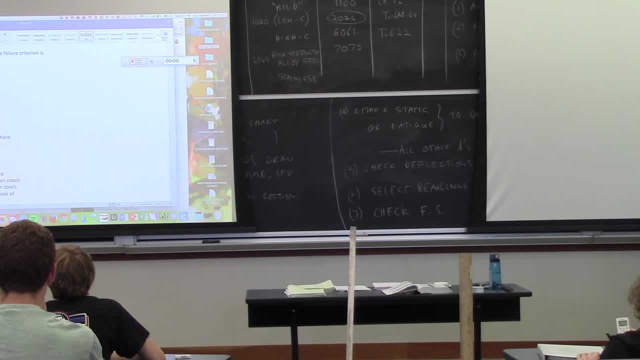 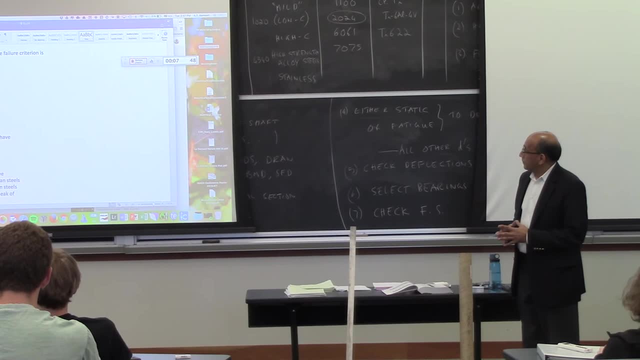 less hardening in the steam. what do you do with the hardening From your research? Okay, One thing I should tell you is the mid-term. the second mid-term will have a number of threads which are essentially multiple choice In this way. 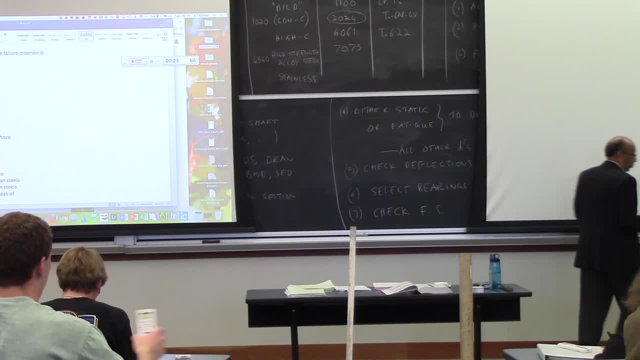